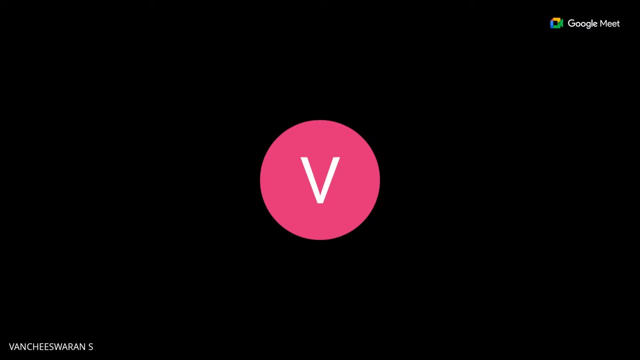 Thank you, Hi, good evening. Am I audible? Yes, sir, you are audible. Okay, fine, So let's start where we have left. So I think you guys have watched the lectures in week 11.. The additional lectures also are available, right? 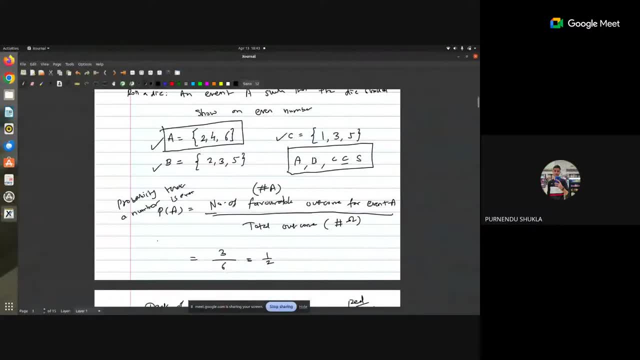 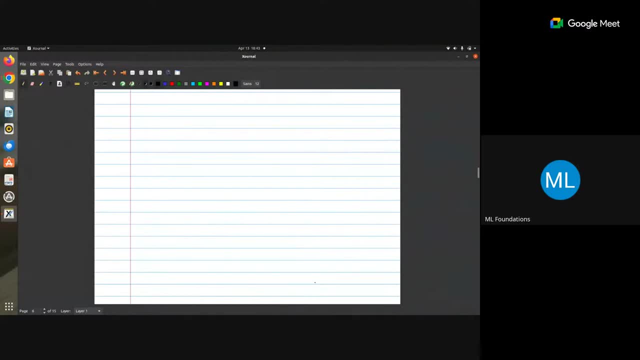 Yes, sir, Now it's available and I have some questions regarding it. Sure, So maybe, yeah, you can. regarding which topic you have questions? First one is regarding this probability space and second one is regarding random variables. So these are the things that we actually 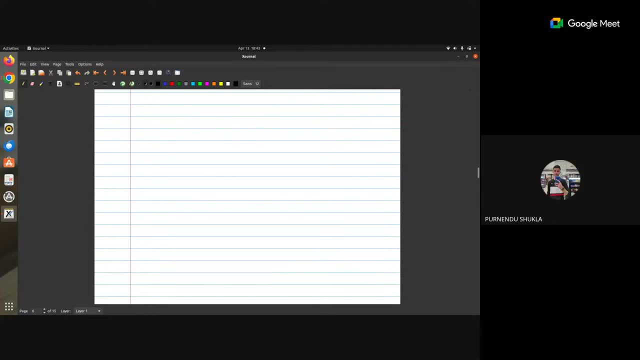 covered right. So I was applying the same logic but I was not getting the right answer. Yeah, can you just tell me the question? Question number 4 for R3 activity, question 3.. Question number 4.. How is 1 by? 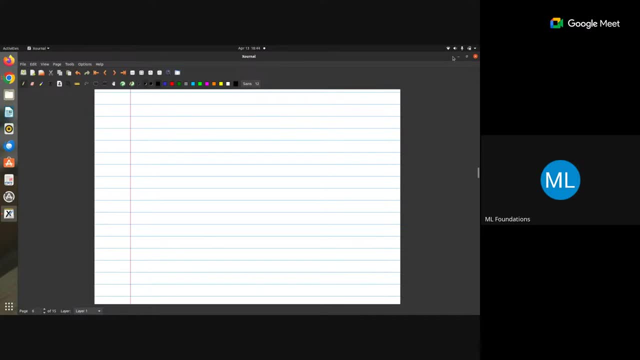 20?? No, no, can you just paste the question here, Maybe, or maybe tell me the question? Okay, so let x be a discrete, random variable with following probability: mass function: Find the value of k. So x is 1,, 2,. 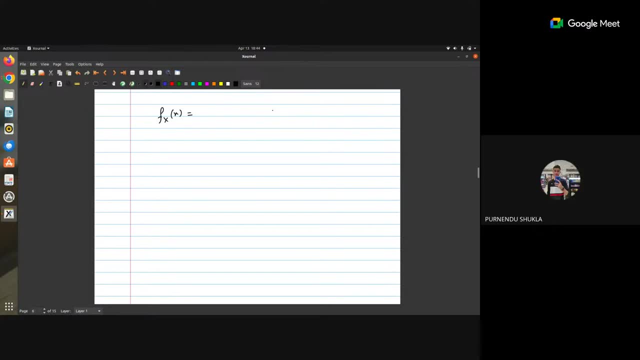 3, 4, 5.. For x equal to 1,, we have 10k 4,, 2, 5k, 3, 4k, 4, 10k square and 5, 10k square. 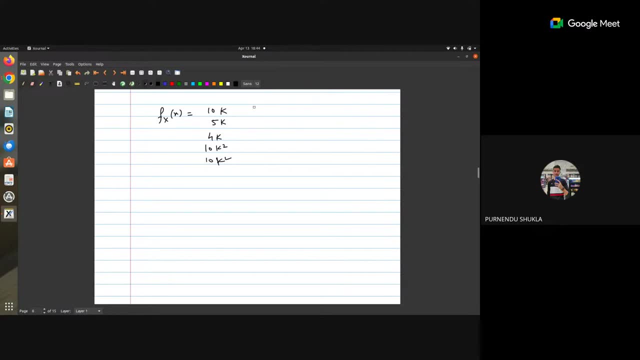 So means it was asking for what is the value of k that we need to find here. So means x equal to 1.. This is the function, right? Okay? So what are the properties? Yeah, so I use the property like summation of all. 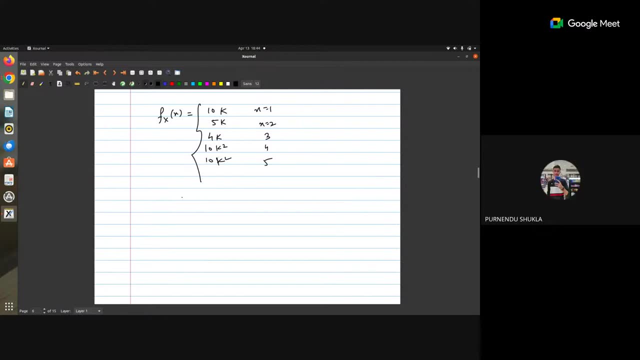 the probability will equal to 1.. So, in probability, mass function x equal to 1.. 10,, 5 and 4.. These are corrected: 10,, 5,, 4k and these are the 10 square And 10k square right. Yes, Yes, sir. 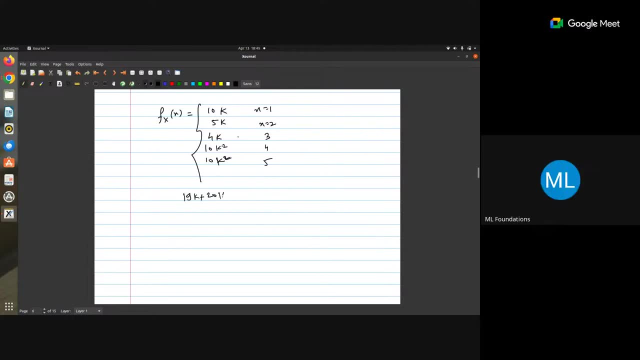 Yes, sir. So let's say this is 19k plus 20 square equals to 1, right, Correct, Sir? are you multiplying it x into p of x whole square means we do probability mass function x into this is you are saying. 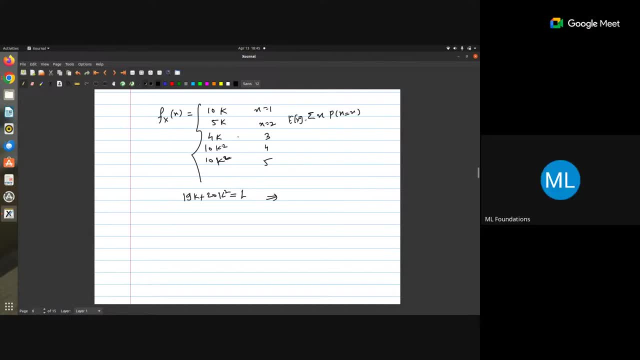 This? No, this is expectation. no, We have already discussed this. The property of probability is 1.. No, sir, actually told. this is the probability mass function: p, m, f. We have already. Then, sir, don't do it. 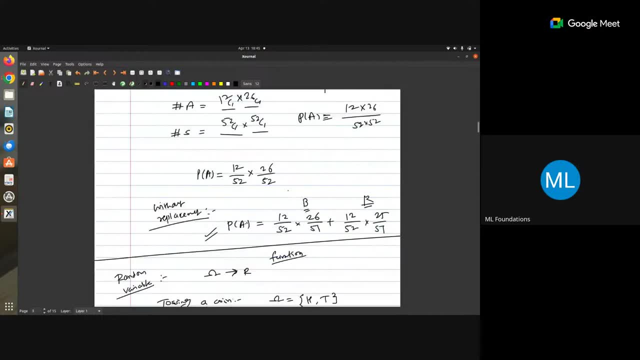 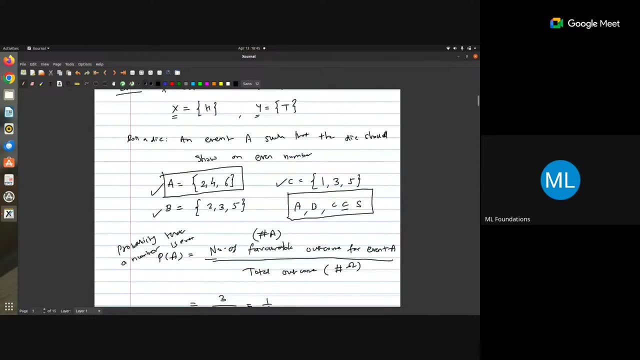 Then I will do it. We already have discussed this. I am having this, the previous sheet. I guess We have discussed that, I guess I don't know. Let's see P m, f. we need to find using x times. 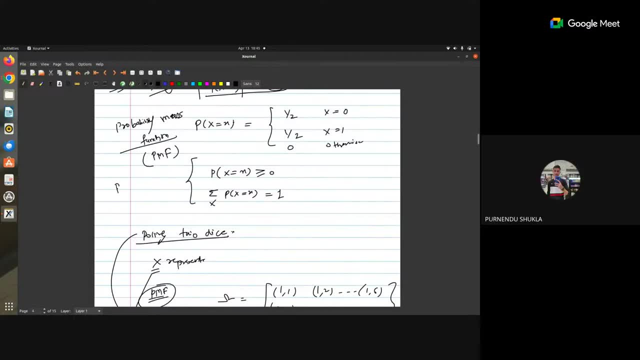 that p of x whole. These are the properties, right? Yes, yes, These are the properties of p, m, f, or what is it? Priority that x equals to x. for all random variables, It is greater than or equal to 0.. 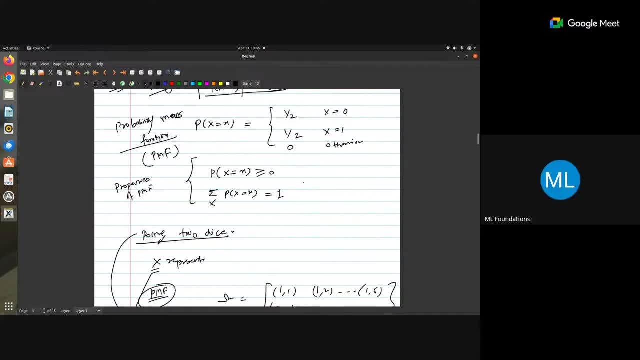 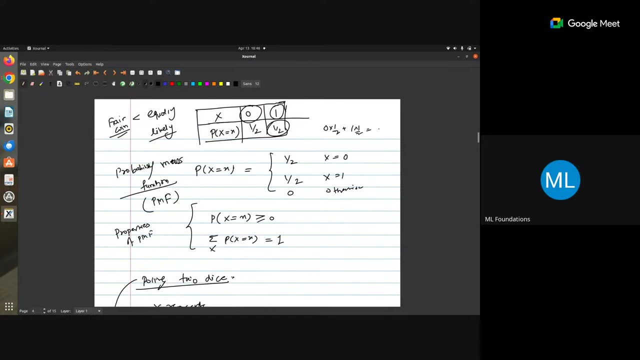 And sum of this priority should be equal to 1, right. So this half plus half should equal to 1, right Now, 0 into half plus 1 into half, This will become half, which is the expectation of x. 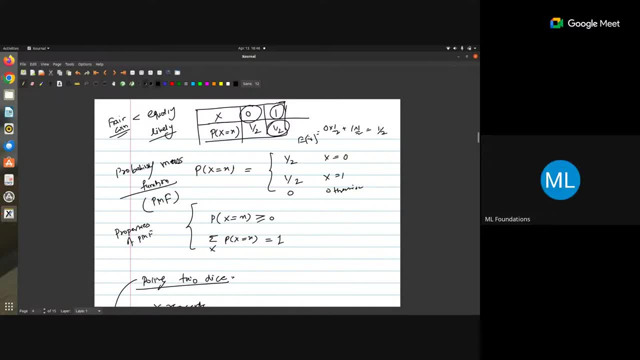 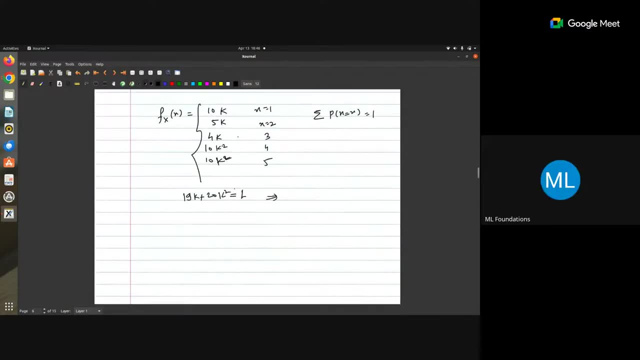 Okay, So expectation: we have seen the formula. You have applied the formula of expectation here. That's why you are getting drawn. And second one is regarding this: axioms, those formulas of the events that we define. It says simply: p of a is equal to 0.2. 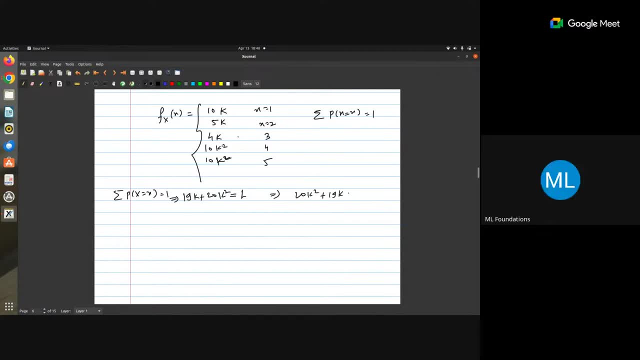 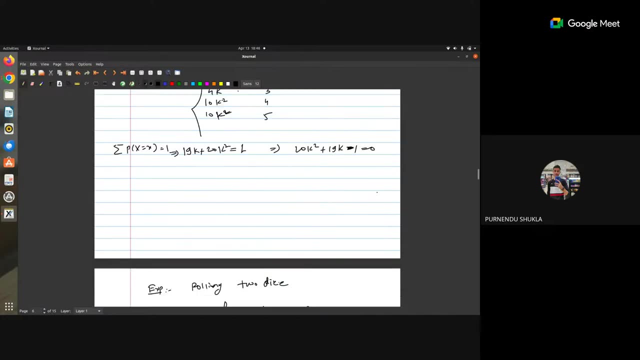 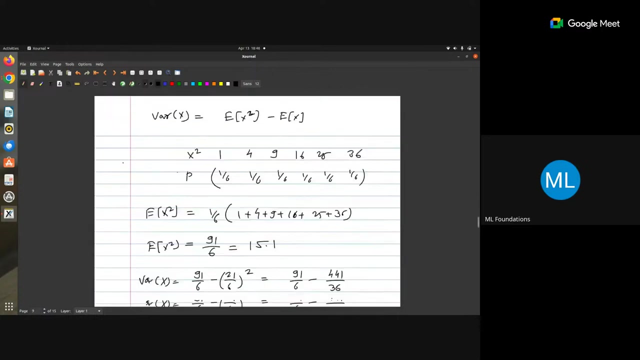 p of b union c is equal to 0.6.. And p of a union b union c is equal to 0.7.. So what is the value of p of a intersection b union c? Okay, We will start with these things. 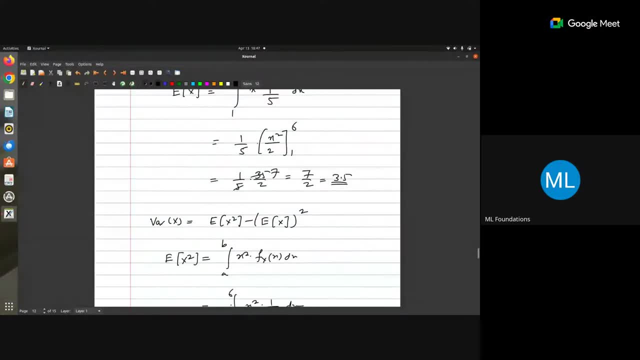 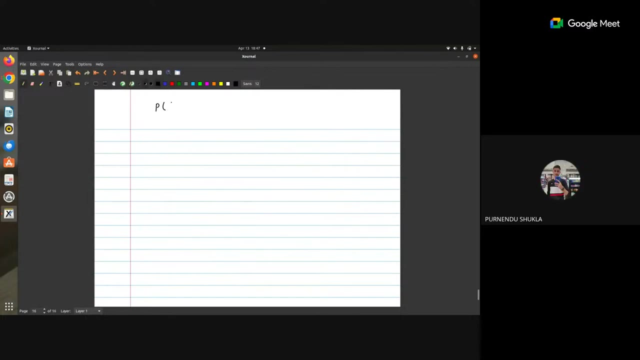 We will discuss all these things. Maybe I will start with this one. This is expectation. This is expectation. Okay, Okay, Yeah, tell me, what is it? Probability? It's p of a is equal to 0.2, p of b, union c, is equal to 0.6,. 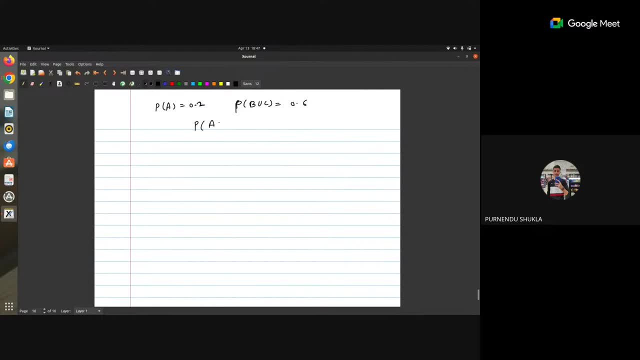 p of a union, b union c is equal to 0.7,, b union c is equal to 0.7, and then it is p of a intersection, b union c. so what i did was p of a, a union, sorry, a intersection like this: yes, yes, okay. what is it equals to? so it's nothing you. 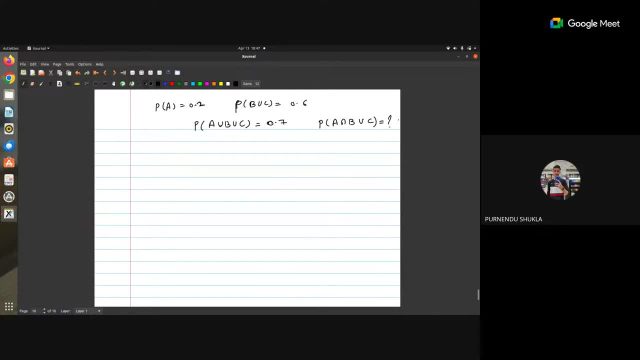 have to find the value of this p of a intersection b union. the bracket will be there. b union c is in another bracket. ah, that's right, so we do this thing first. actually, so means what my approach was. like a intersection b formula i was applying, so i was not getting the right answer or when i 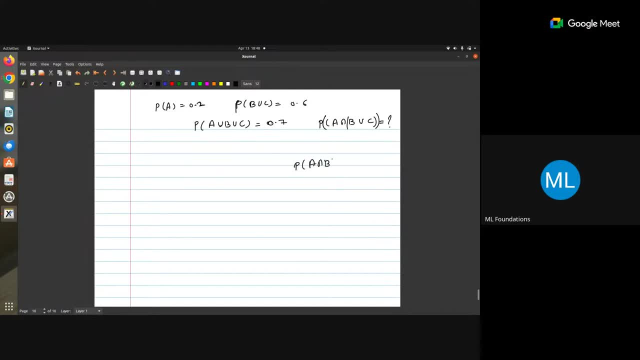 okay, so you, you are actually doing this. a intersection b and no, then it will be right. this is possible, right? yes, or you can actually find for this, and then you can. it's already there. b union 6.6 is there. you need to find what is a intersection b union c, right so? 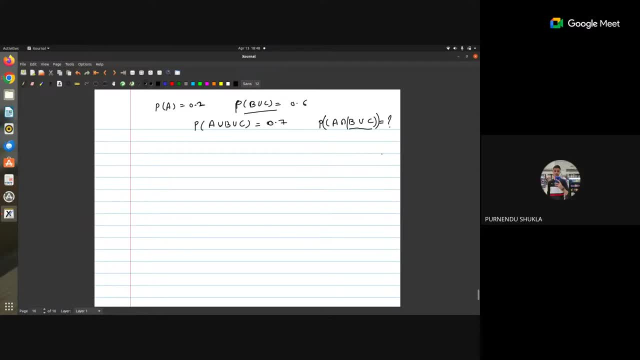 actually basically this: this thing, only p of a union b, union c, we can use directly, directly. how can you use? so we can use this, so we can use this formula. it is given, yeah, so make this. let's say d, okay, okay, so a union d. so what is the formula? a? or maybe, okay, let's say p of a plus p of. 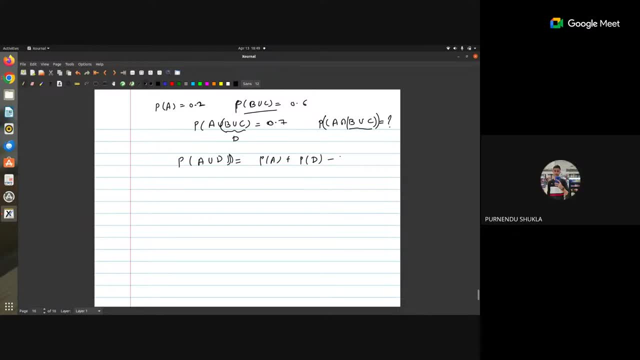 d of p of b minus minus p of a intersection d, a intersection d- right, correct, yes, yes, uh, but what do you want? let's say you want probability of a intersection d. right, you want this correct, yes, so this: so probability of a intersection d is equals to probability of a union d plus probability of. 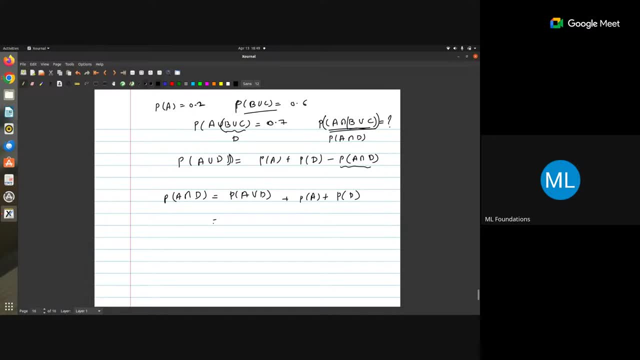 a plus probability of d, and i think you are. you are having all the values. the probability of a union d is 0.7, plus probability of a is 0.2 and plus probability of d as. uh, okay, i think. uh, what is this? is not this b union c is there? so sorry, no, no, it should be mine. 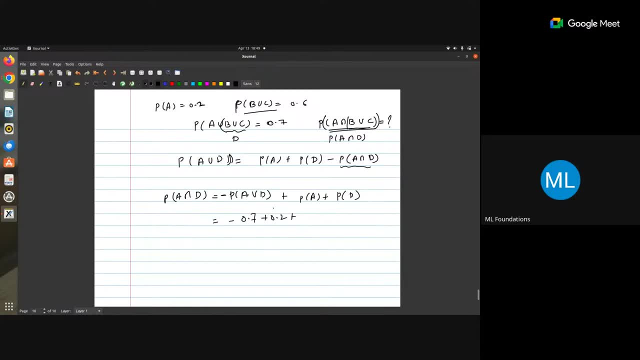 c is 0.6 already. ah, that is okay, but it should be minus, right, minus, yes, that will be minus 0.6, so then it should become 0.1- 0.1. yes, that's the right answer. this is how you. okay, so i can take. 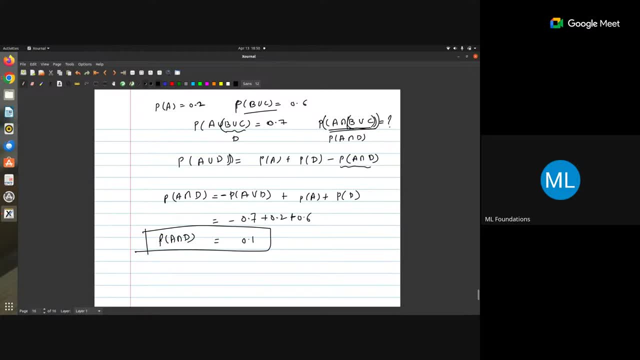 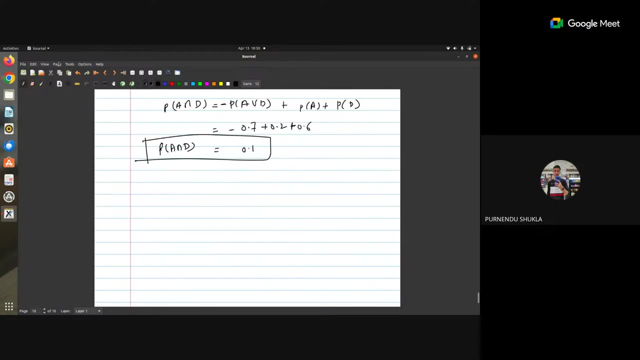 this no means i was just: yeah, this is one event, this is one event. you can consider this as one event and install it. i just wanted to clarify on that. only for conditioning. i watched the lecture, but we will see, we'll see. okay, let's, let's okay now. 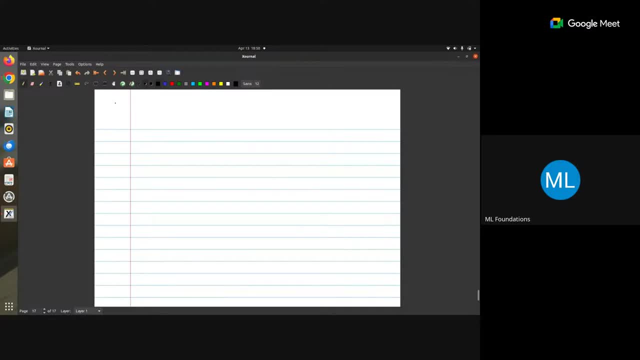 let's start a fresh for everyone. uh, let's say: uh, maybe we'll start with uh joint pdfs or joint pmx first, and then, uh, from there we'll see joint pdfs. okay, suppose, uh, random, there are two random variables, x and y. uh, with following joint pmf. okay, so you know how to write the joint pmf. 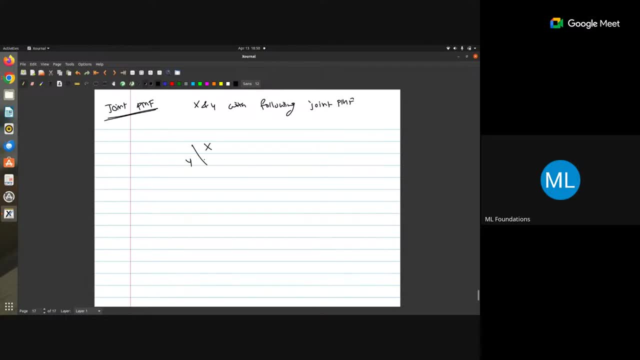 so let's say, we have x, we have y here. fine, i have this x here. okay, these are the two random variables, any two discrete random variables. okay, because pmf is, uh, basically defined only for discrete random variables. okay, so this is, and values are, let's say, zero, point one, point two, point five, zero. 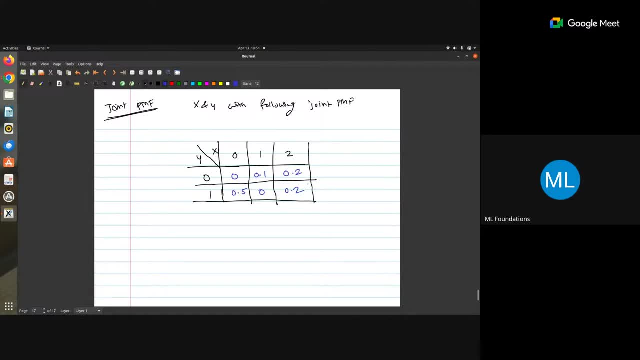 point two, is it correct? so let's say, if these are the values here, so what is the uh? what are the properties of uh, joint pdf or pmf? you can see that the sum uh of all these values right. so generally, what is this? x, zero, zero, what? 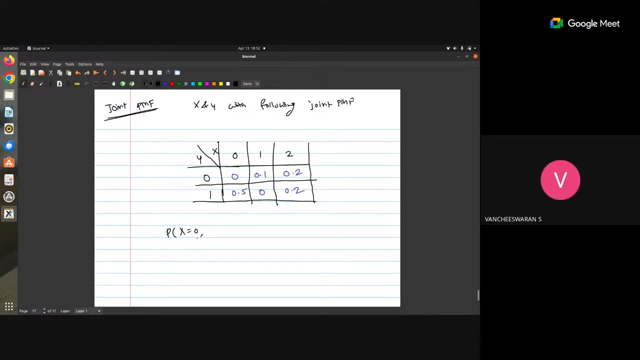 is that meant by? like probability that x equals to zero? is what let's say? it is probability that x equals to zero, intersection, right, yeah, this is the meaning of it. this is the meaning of this. is joint gender generally, it is a intersection and you can think it as uh, intersection, or let's. 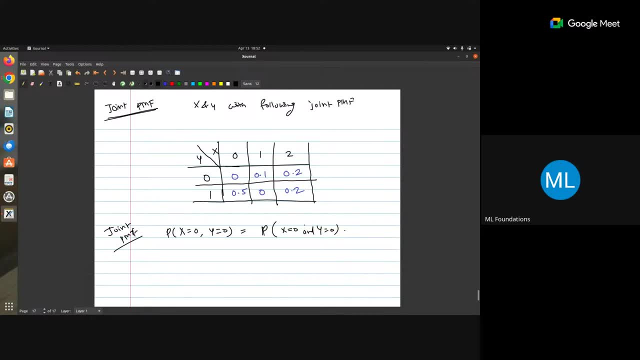 say: and okay, so there is one more concept, uh, which will come here, which is, uh, independence. right, uh, we'll talk about that also, but first of all think about this: okay, so, uh, yes, by basic principle of counting, you can know that the level of the exact wave here you know, r the'd uh, no, no, take up here andaze, okay, not, or do there and and le. inter section, or so that means having equal poi inter 말이ay noi of what so say uh alteca, which means yeah, so a candidate from the interpeare qui will come here. it is then, um, we'll talk about that also, but first of all think about this. okay, so I know we have some. 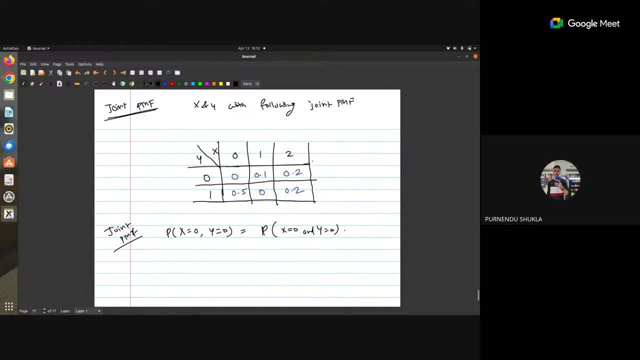 individual ideas. mr can bring that to you. so the integration by doing so means there is one front side set here. the est�� is known for counting if we have or we do a add, and if we have and we do a multiplication. yes, here we will do. 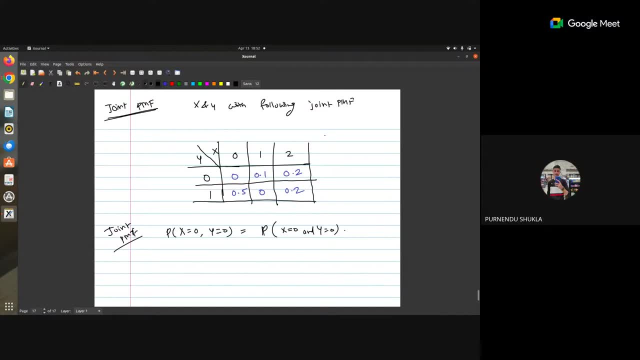 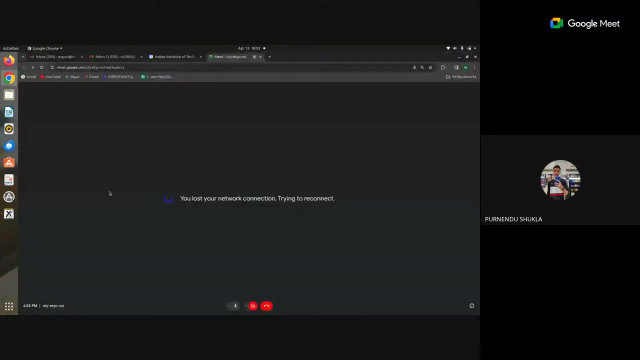 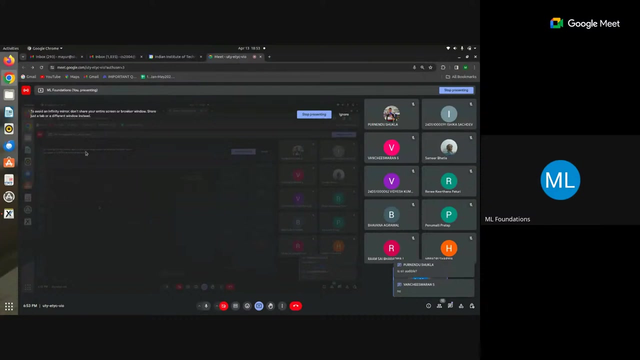 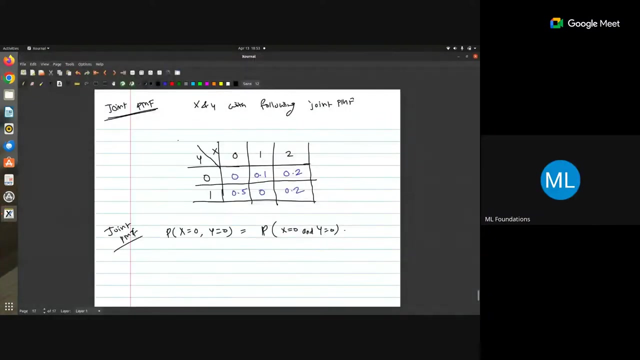 multiplication. sorry, you are not sorry. uh, i think my network was, yeah, so current, uh, am i audible now? yes, sir, no, you are okay, so, okay, uh. so let's say: uh, this and is there, but this is not every time you can say that it should be multiplied, like you can multiply generally, if you have the multiplication uh rule of counting. 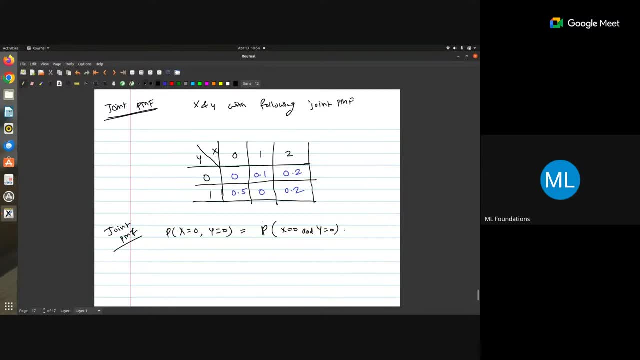 or maybe that, uh, it will come in probabilities also. it is a different here. also, it applies, it applies, but it depends on what it depends on. uh, the independence. we'll talk about that later. first of all, try to understand this joint pmf. what is the meaning of it? 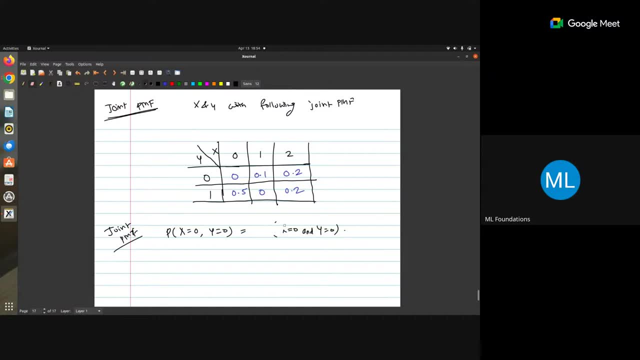 so when i say probability that x equals to 0 comma, y equals to 0, uh equals to zero. what does that mean? that uh, there is uh. like the probability that x equal, x equals to 0 and y equals to 0 happening at the same time right together, is 0.. similarly, that probability that x equals to 1. 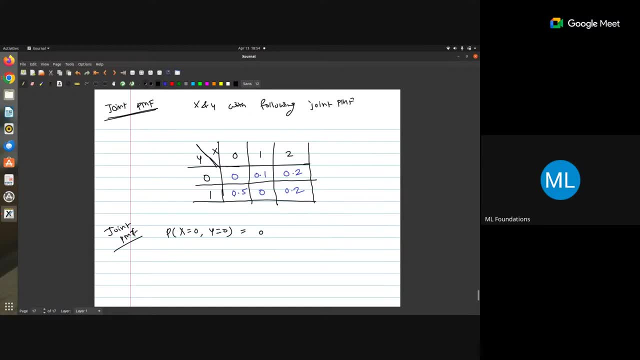 event that probability that x equals to 1 and y equals to 0 happening is 0.1. okay, so, uh, you can consider this as, let's say: uh, you have, uh, maybe you can consider any. uh, i don't know like you can take some example of x as a discrete random variable and y is another. 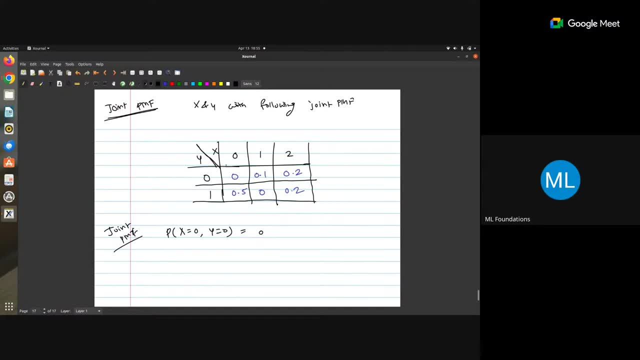 random variable. for example, let's say x is one person. let's say rowan is there. ron is having, uh, rowan may be having, like, uh, car. okay, what? what actually represents? let's say x represents. represents number of number of. let's say a bits. 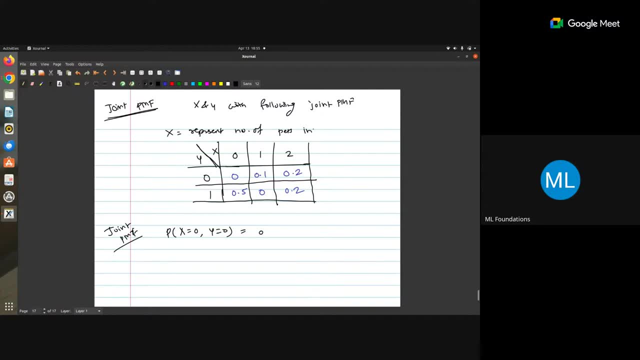 uh say at, uh, at some particular day or something like i don't know, maybe we can define or number of bits, he a number of, let's say, number of cars, this like something like this: okay, and why is uh? what is the probability that maybe this is rowan and suppose y is? 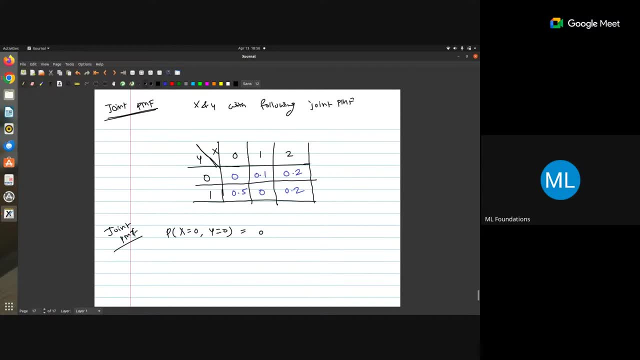 i don't know. okay, maybe we will think about some better random variables, but currently, okay, understand this as, let's say, one one person is uh having this, or maybe a random variable is having this: three uh values- 0, 1 and 2, and y is having two uh values, uh, zero and one. so what is the probability? 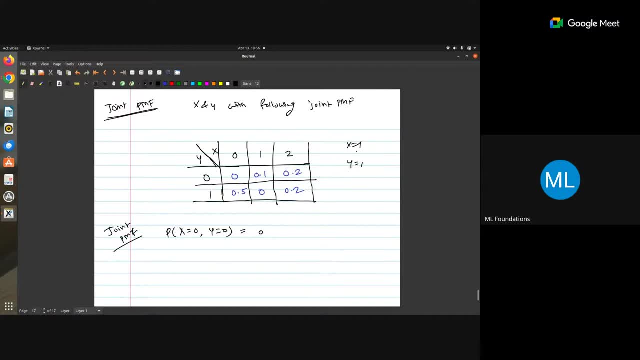 event and y equals to 1 is another event, right? so what is the probability that x is equals to 1, the the the event happening, x equals to 1 and the event y equals to 1 happening. what is the probability? and simultaneously, so that probability is given as this: it is 0, right. similarly, 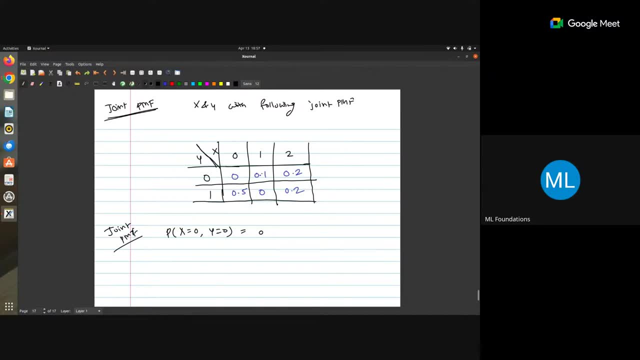 what is the probability that x equals to 2 and y equals to 1 happening at the same time is 0.2 right, okay, so that is the uh interpretation of this pmf table. right? one more thing is: uh, the important part about this is the sum of all the probabilities. right, some of all these joint 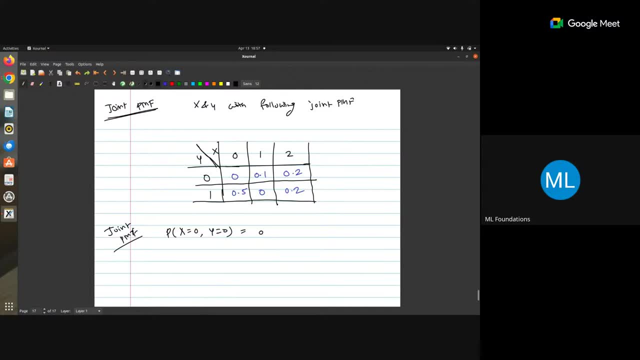 joint probabilities is equals to 1.. you can understand it from here: 0 plus 0.1 plus 0.2 is 0.3, 0.3 plus 0.5 is 0.8, and 0.5 plus 0.2 is 10.. so sum of all the joint probabilities. 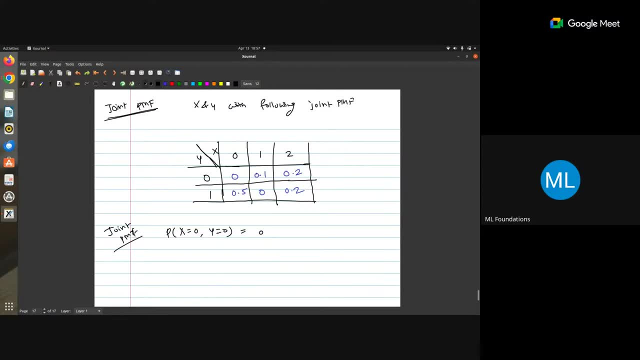 right, that should be equals to 1 for the given, uh, random variables. there is one more term: uh, so this is, uh, this is what this is. a joint probability. right, there is one more term. is that is called as marginal probability? okay, marginal probability. so what is? what is the? 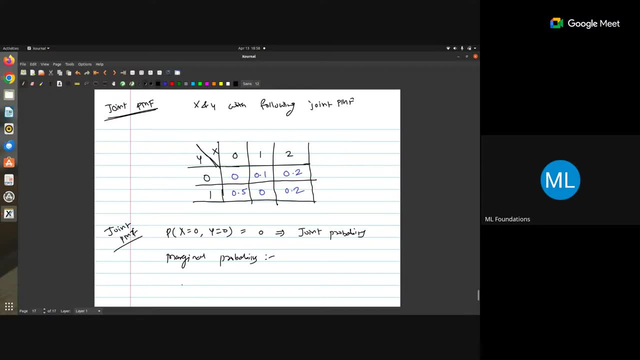 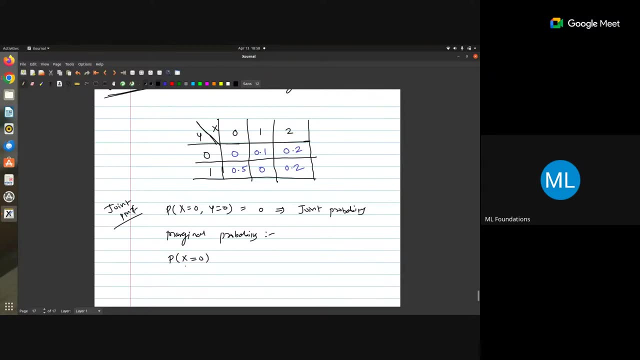 meaning of marginal probability here? uh, it is that like. so suppose, what is the? if i ask you to find what is the probability that x equals to 0, how? or maybe, let's say, y equals to 0? so what do you? what do you say, uh, what is the probability that y equals to 0? 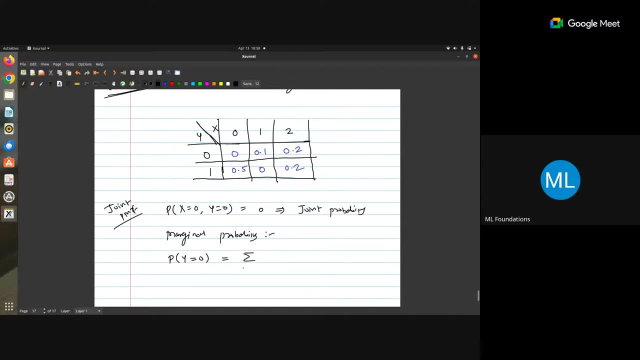 that means: uh, it's a sum of all the probabilities, keeping y equals to 0 as constant and you know, changing or, or. let's say x will go from, or x will be from the range of x 0 to 2, and uh, i'll say product x equals to small x. 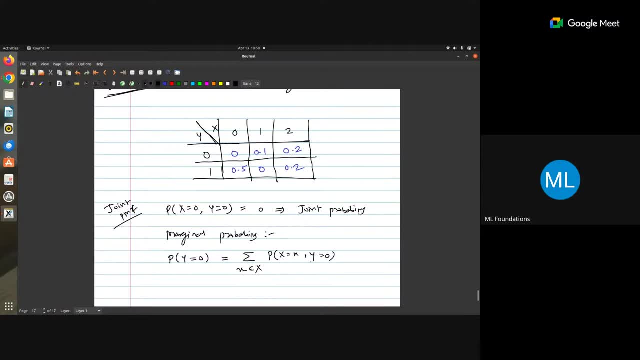 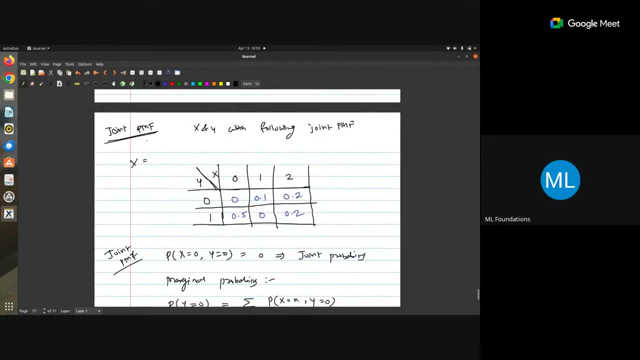 y equals to 0. okay, so this is the probability. so x will go from x. what is the range of x? x range of x is yeah, 0, 1, 2, 0, 1, 2. the range of y is only 0, 0, 1. no, range of y is 0, 1 and. 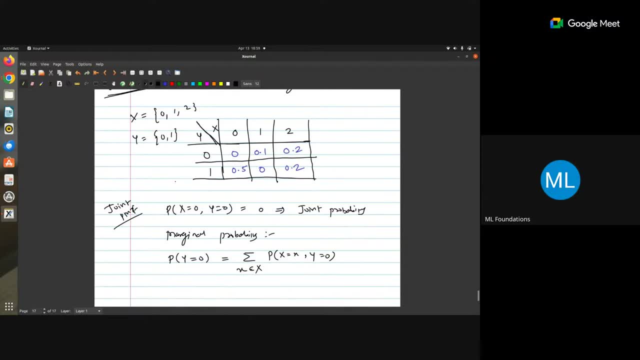 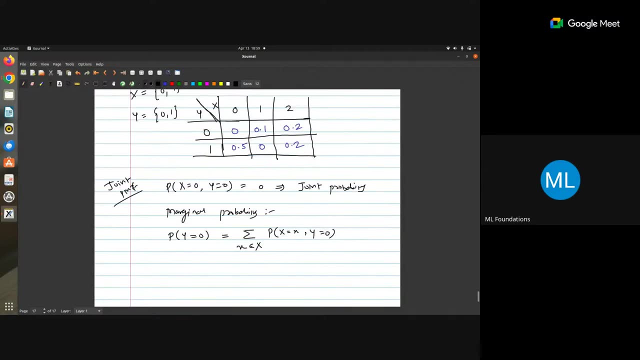 range of x is 0, 1 and 2.. so we need to find what is the probability that x equals to x, given y equals to 0, right? so that means i have to keep y equals to 0 constant and add all the probabilities across the range of x. okay, so maybe i'll say that. 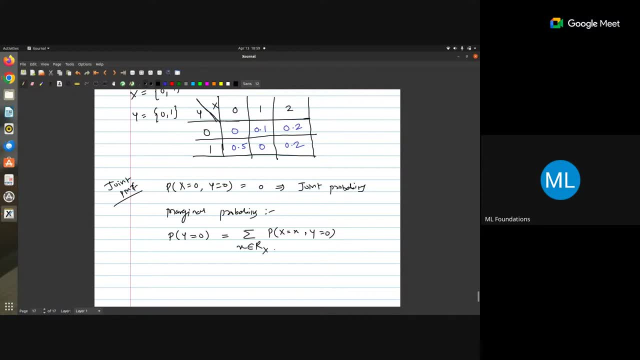 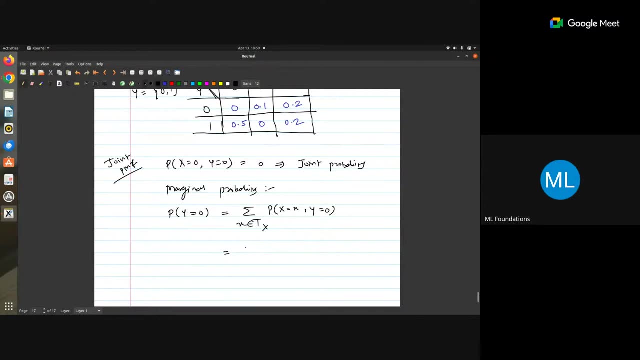 it's the range of x. i'll make this as the range of x. okay, rx is the range of x. you can say rx or tx, something like that. fine, so here, what does that mean? it means probability that x equals to 0 and y equals to 0, okay, plus probability that x equals to 1. 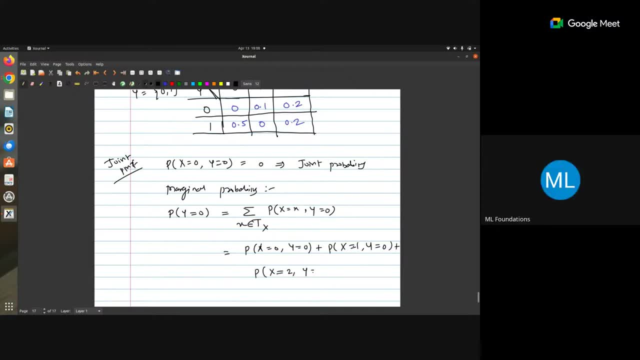 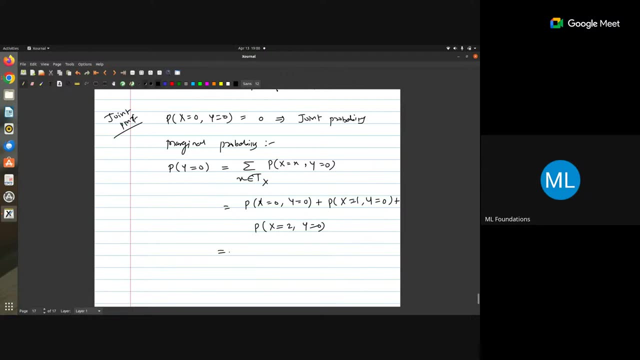 is 0 plus x equals to 2, y equals to 0. so all the uh it is, it is the sum of all the joint probabilities keeping y equals to 0 constant. so what is it here? it's 0, 0 plus 0.1, 0.2, which is 0.3. can you tell me what is the probability that y equals to 1 now? 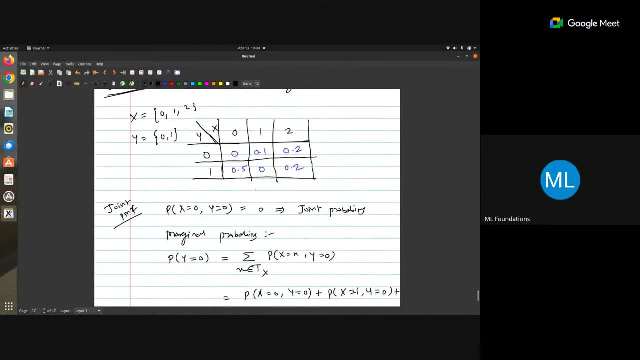 by looking at this table: 0.7. right, so, uh, i'll. and where, where should i write this? so this is, this is 0.3. okay, this is what this is, uh. marginal probability of y equals y equal to 0. yeah, yeah. margin of probability at y equals to 0. 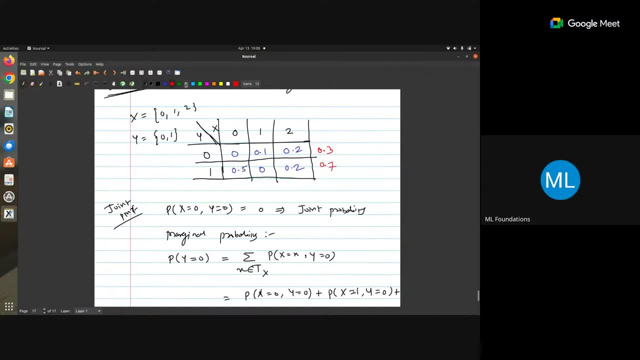 and this is 0.7. okay, what does this number represents? 0.5 marginal probability of x equal to zero. yeah, my name is robert at. x equals to zero. what about this 0.5? one at one. so how? how you define pro, how you find out the probability of x equals to one? 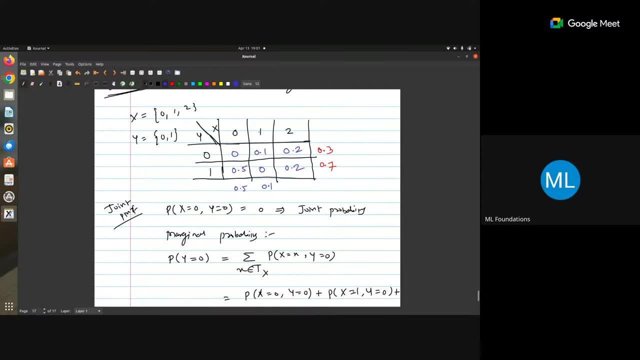 keeping x equals to one constant and summing across the range of y. right now you understand. uh, what is mario? so what? this point one is? it's a joint probability, right? and this point three, point seven, point five, point one, point four are the marginal probabilities. 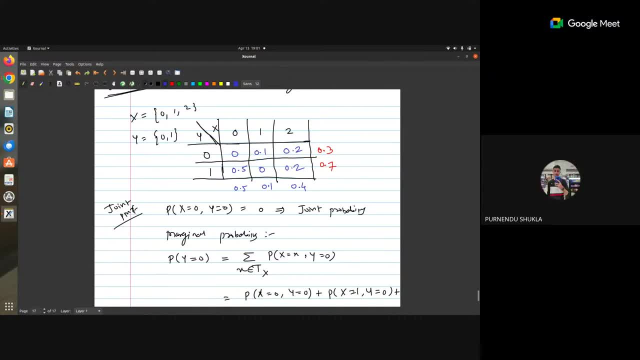 so okay, okay, but here, uh, the pmf table is given, but in gen, in some say large experiment where we have a lot of outcomes, it's not possible to create this joint pmf table. so then, how we will solve? same same principle you have to use, keeping x constant or y constant, and 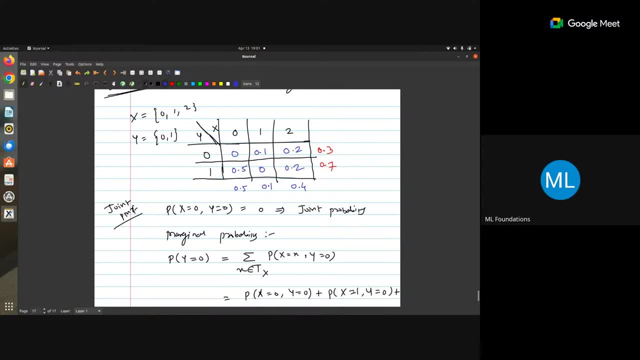 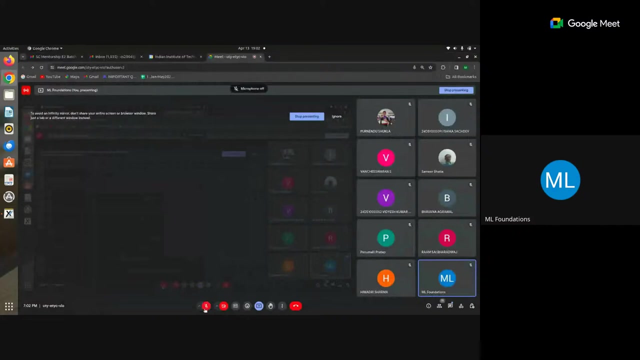 summing over the range of x or y. yes, yes, so then in this case, we will see that the probability of x equals to one over x. is the probability of x equals to one over x? yes, very much, correct. uh, just a minute. i have to take a poll. 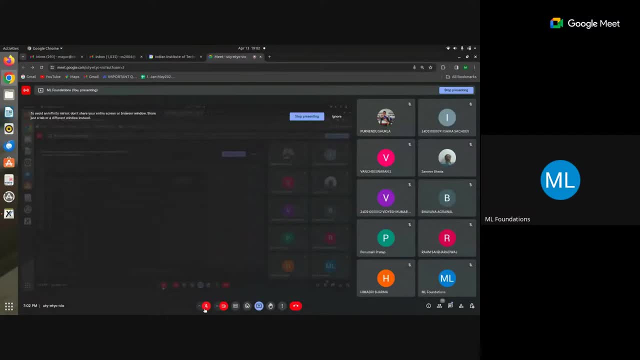 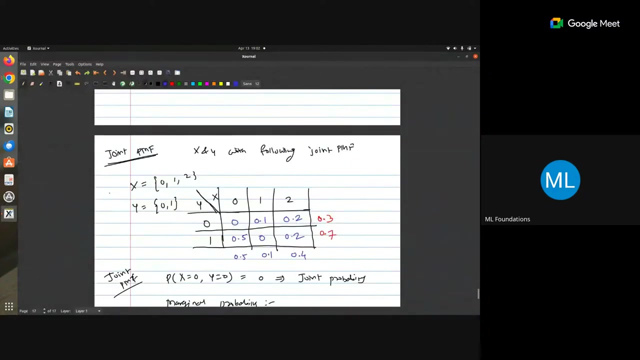 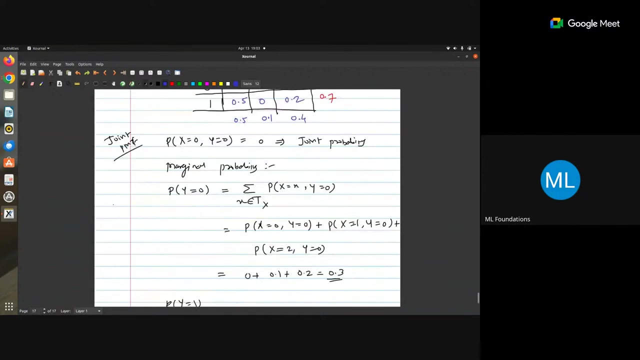 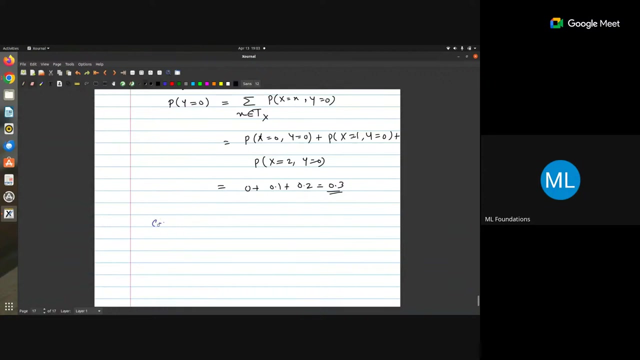 okay, sorry guys, uh, so, uh, yes, so here you understand. uh, okay, we will. we'll talk about that also, like how to find the joint and marginal probabilities there also. uh, again, there is one more term which is called conditional probability, right? uh, conditional probability, so you know what is conditional probability for single random variable, right? 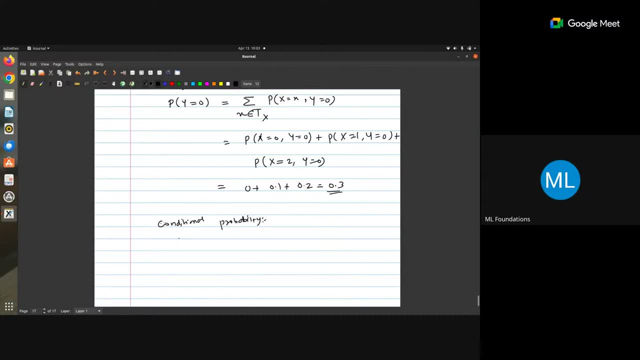 so, uh, let's say, you, if you have uh any kind of you know, uh what? let's say there are two events. okay, probability of let's say there are two events, a and b, what is the conditional probability that event a will occur, given that b is already occurred? what is the conditional probability in that case? 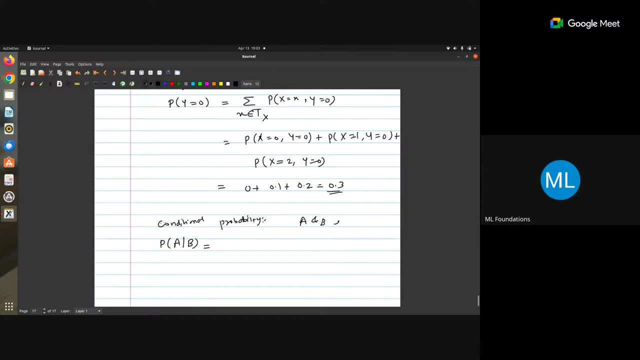 sorry, is it something like a intersection b by probability of b, correct? so it is a intersection b divided by probability of b, right and what? what does this? what this particular statement that we say right way of a intersection b by probability of b? so what does this particular statement? so that means okay, what do you understand? 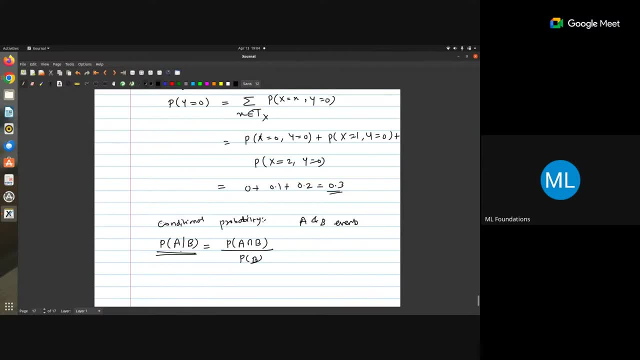 by. so what this? okay, what is the interpretation of this? first, what is the probability that event a will occur, given that even b has occurred? okay, so suppose, uh, let's say i don't know, you can take some real life examples also, suppose you are saying that: 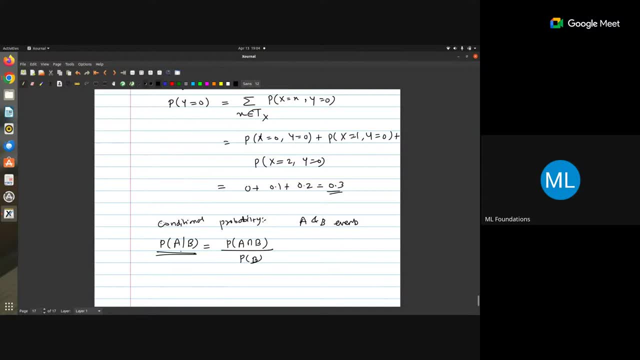 there are two events which are dependent on each other. for example: uh, okay, so some- let's say some chemical reaction, right, if, if any chemical reaction has to occur, uh, some prerequisite chemical reaction has to occur, right? so, if something like that it is there, then in that case, what? we will say? that? what is the probability that? 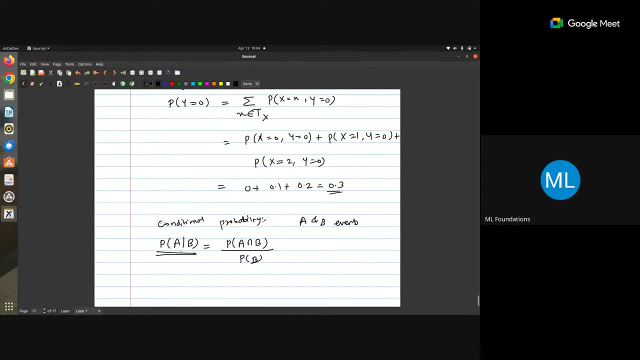 uh, this chemical reaction, A will occur, given that b has already occurred. right, so what itけてey8 perhaps possible that without b, a can possibly suppose, if i have to reach at. uh, okay, there are, let's say, two people, are there, a and b suppose okay, and uh suppose a started from, let's say, uh started. 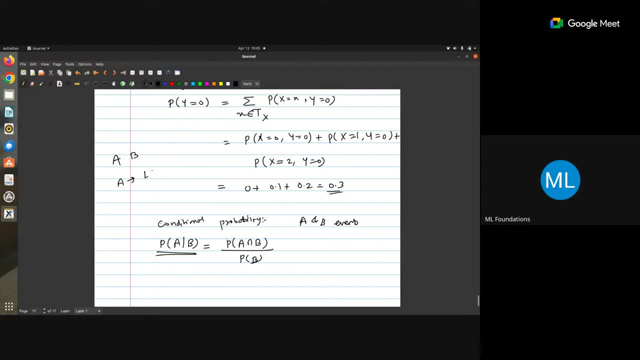 his journey, uh, from, uh, so from particular station, let's say from lucknow, let's say from 10 am, okay, and he, let's say he, he starts his journey from 10 am, uh, between 10 am to 12 am, okay. 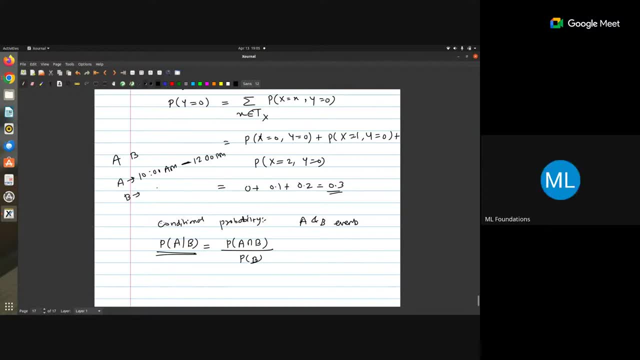 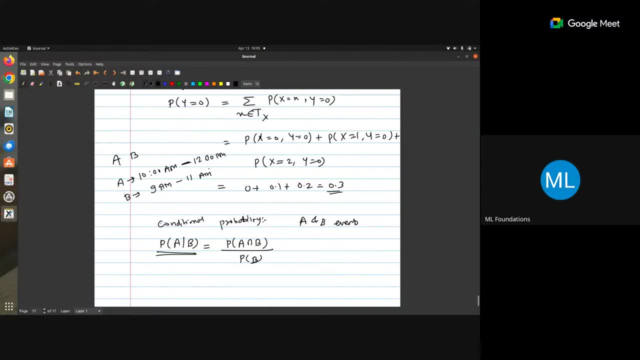 with 9 to 11 am. so what i'm saying is: this is their regular schedule, right, and this, let's say these are uniformly distributed for both of them. what i'm saying is: what is the conditional probability that uh a, a, a has already started from the uh given station, given that b has already? 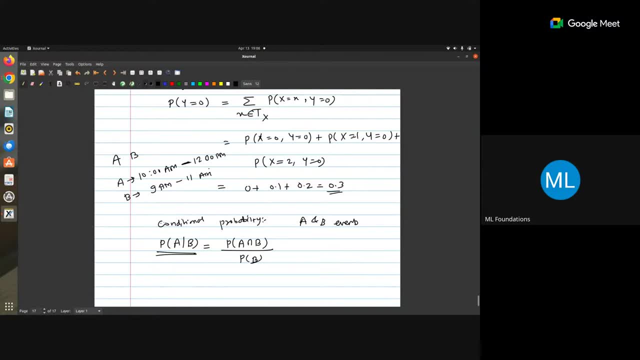 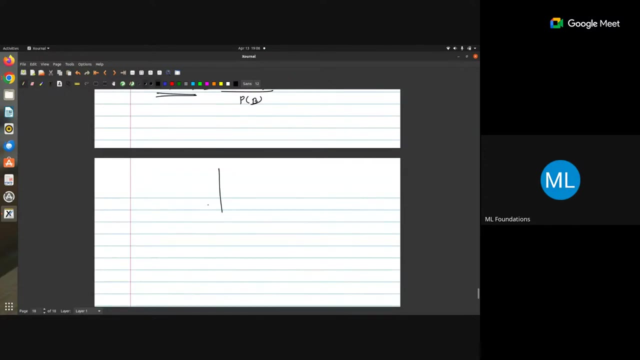 started, or what is the probability that a, a will start uh on that same day, on particular day, at 10 am, given that b has already started? so what if you, if you try to visualize this, this will look like this, that i will take a example of uniform distribution, for example. so suppose uh, this is. 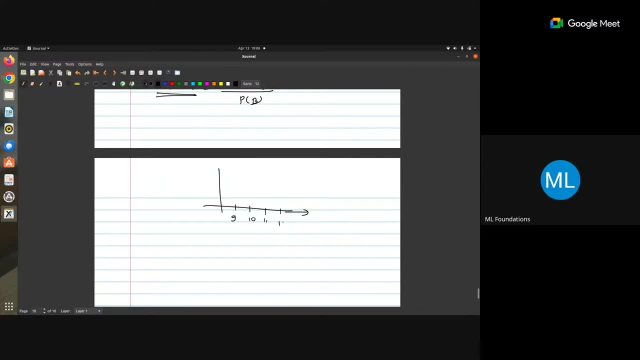 uh, 9 am, 10 am, 11 am and 12 am, so right, so a is a is uh, a can start his journey from 10 to 12 pm and b is starting his journey from 9 am, 9 to 11 am. right. 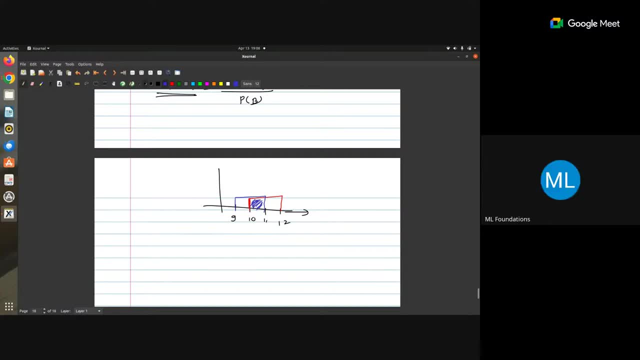 so there, this, this portion of this right, is what this common right or this intersection is called intersection right, p of a intersection. so what i'm saying is, let's say this is a red represents a event, a blue represents even b. so the question is: what is the probability that a has occurred? 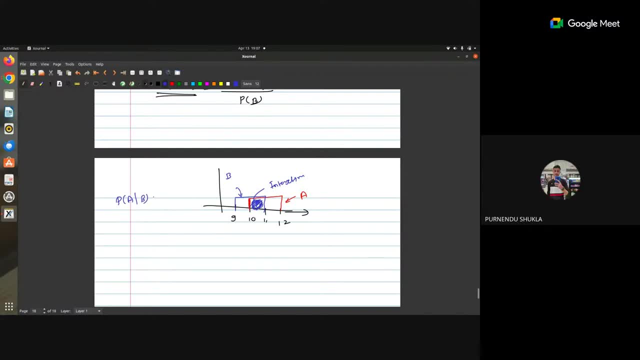 given that b is already, a will occur, given that b has already occurred. okay, so, so what is that? a is a intersection b divided by probability of b, and the reason that we are taking a intersection b is because a is contained in that particular b, correct, so? and that we have to find out, and this: 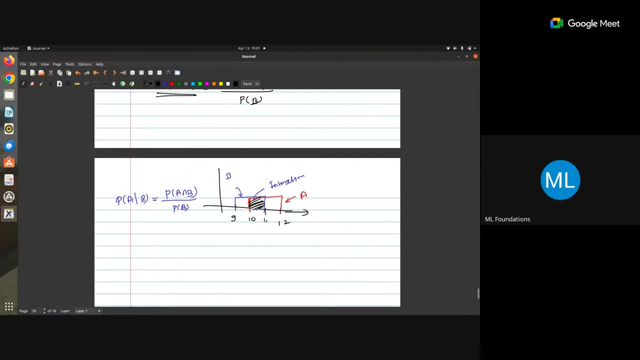 that means graphically, if you see this red color, red marked area divided by this, only b, not the part of a right. so that is. that is because a has to occur and b is already occurring, but a has some parts in that particular b. so common point will be where the 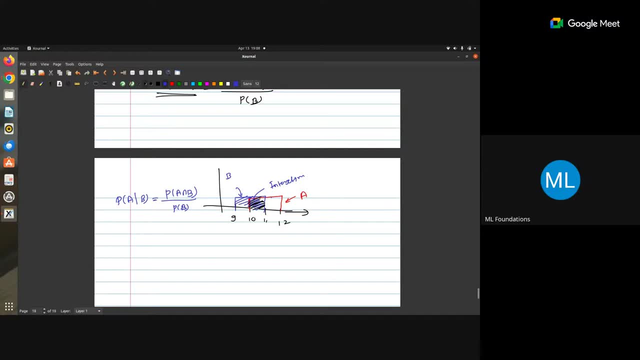 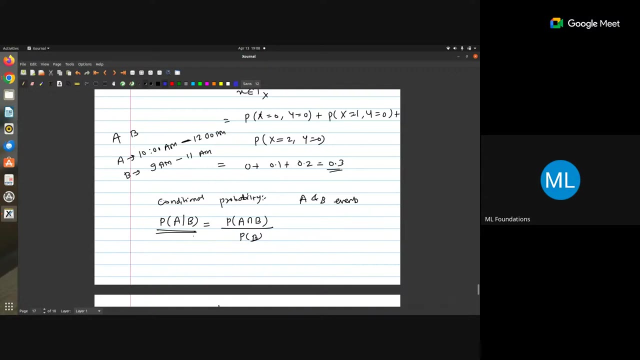 probability may lie correct, right. so that means a and b, both are occurring at the simultaneously, given that b uh already occurred. so that is the complete probability. okay, that is the meaning of it. that is the meaning of conditional probability. okay, so in this case, uh, okay, one more statement i'll write, try to write down here. so what is probability? 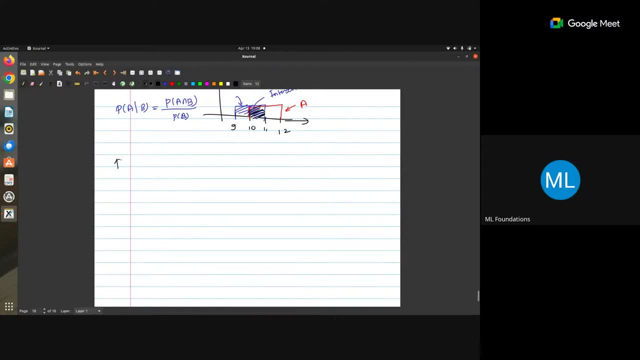 okay, i'll write it again. okay, this is probability of a, b intersection b. then what is property of b intersection a? it is probability of. uh sorry, what is the probability of b given a? that is probability of a intersection b, intersection b by p of a right. so in this case, 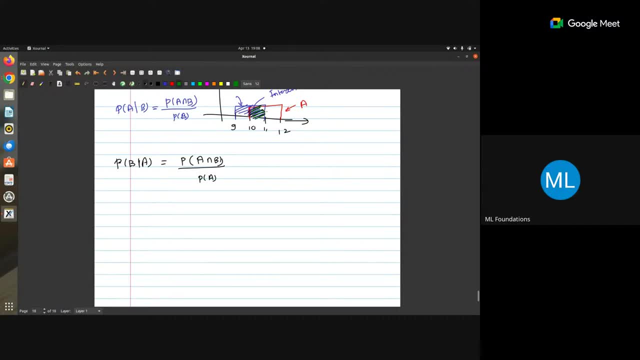 which? which region is there? so intersection region is same. but now we will take a, now this one, right? do you understand? that is the difference between these two. now can't we have like one minus probability of a given b? you can, you can have, but it depends on. 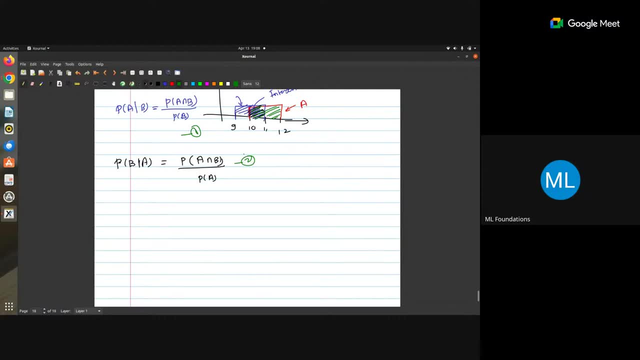 like how uh these events are. so this is the simple example where we know that this is uniformly distributed and they have these things common, right? but every time, whether it is same or no, that we don't know right. here, only thing is common is what, uh or correct a intersection b, that 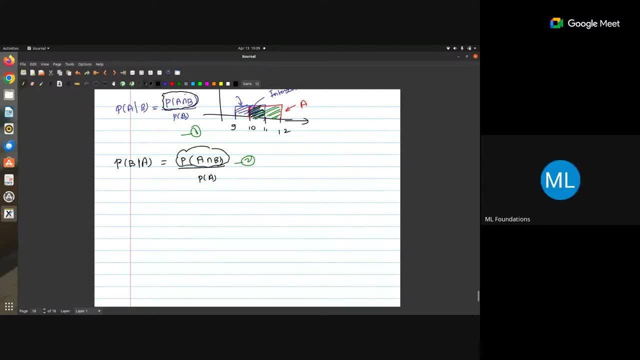 particular reason correct. so from this two equation what we can found out is: can i write probability of a intersection b as from equation one, as probability of a given b, into probability of b right? this from one again, probability of a intersection b. i can write it as: 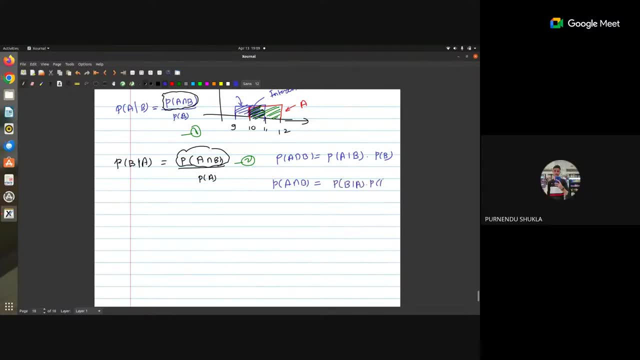 probability of b given a, given a, into probability of a. okay, if you go for the base theorem, this probability of b or probability of a, it is called total probability, right? base theorem where you have, uh, multiple events, uh, at the same time, right? so here we are just dealing with two events, a and b. 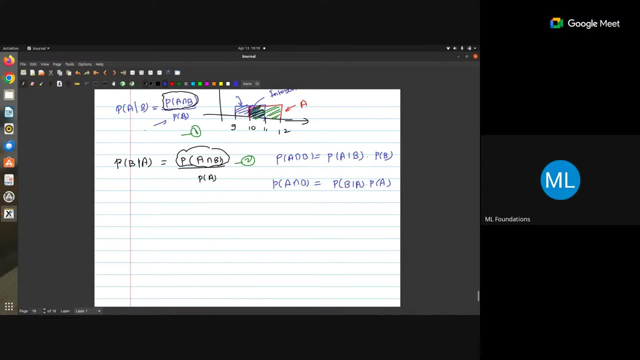 if you have multiple events and there is one event which is common between all the events, then in that case, uh, this is called as a total probability. okay, but that is not required here currently. you just understand this one. so, uh, from this equation, let's say, this is three and this is four. from this, 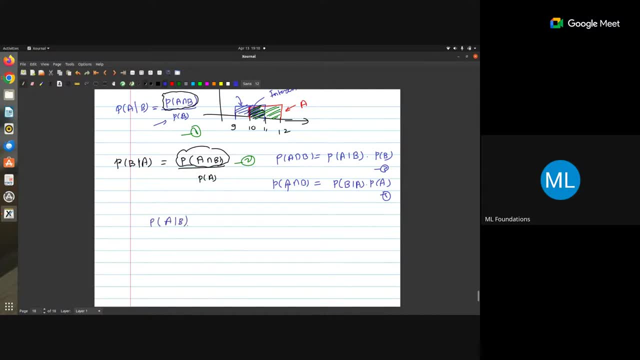 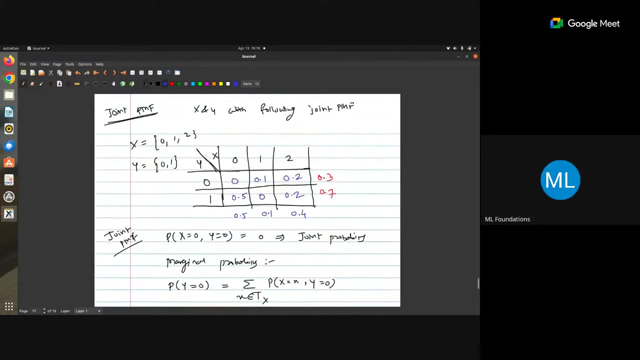 three and four. can i say that, safely, probability of a given b into probability of b is same as probability of dónde le? this is actually nothing but probability that x equals to zero, intersection y equals to zero, right? if these two even so, suppose i say that probability that x equals to zero is event a. 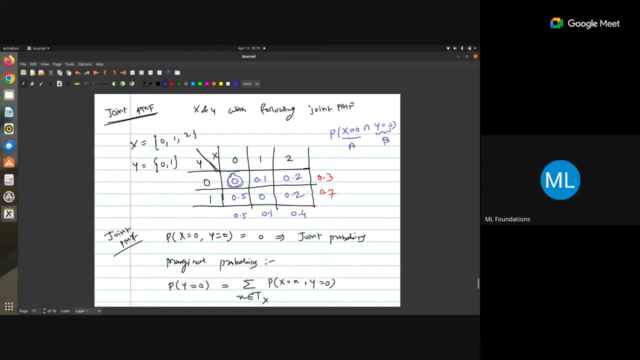 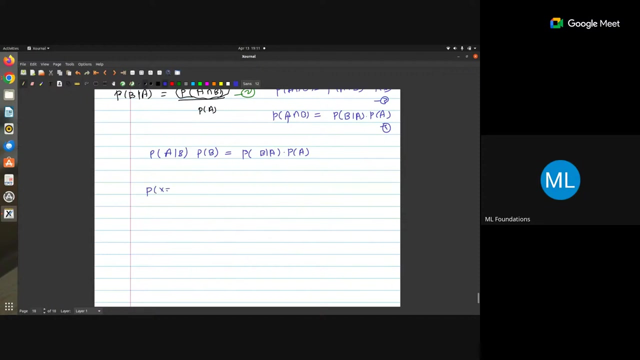 of y equals to 0 is event b. then this 0, this value 0 is giving me what probability of a intersection b, right? this joint pmf is giving me the intersection of this two, right, these two events? okay, so if i wanted to write down: uh okay, can i. let's say probability that x equals to 0. 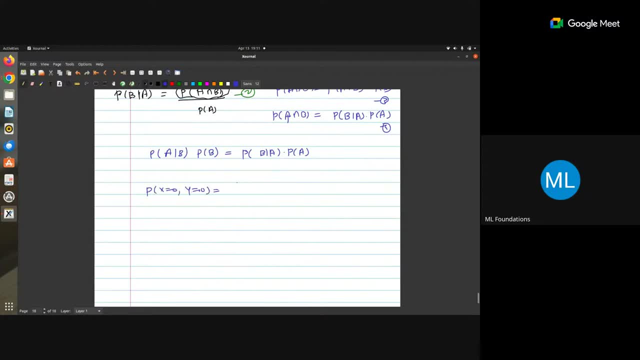 into probability of y equals to 0. can i write down: uh, this has probability that x equals to 0, given y equals to 0. into probability that y equals to 0. is it possible or is it correct? so how? okay? consider this as event a. this has event b, so i can say that probability of a given. 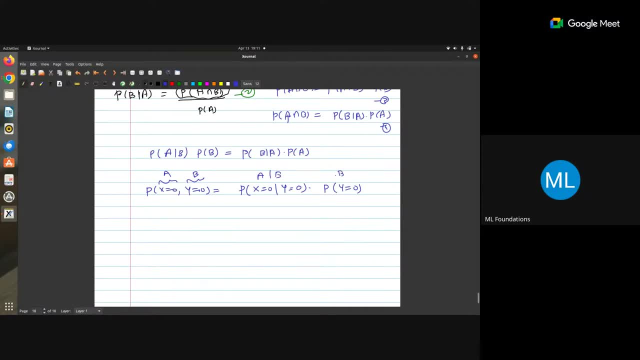 b into probability of b. so is that intersection part here? this, this thing, is intersection, right? yeah? yeah, that is what i told you, right, this joint probability is nothing but the intersection. so i can safely write uh this here, right, but in this case, what is? probability of y equals to zero. uh, showing what is this first. 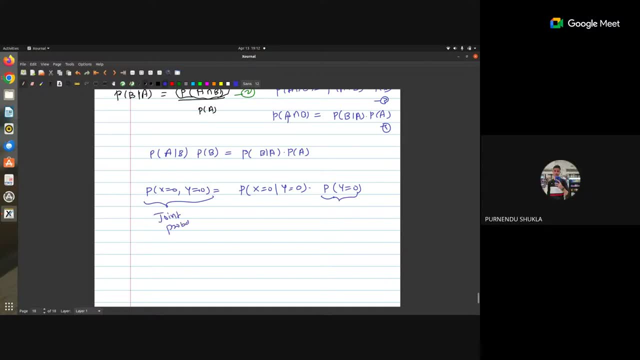 this joint probability so zero. what is this? this is what that is: marginal, marginal, marginal, right, this margin probability, and this is what. so now you understand, uh, the difference. okay, now one more thing. uh, if i wanted to find the conditional probability here, for that x equals to 0, given y equals to 0, 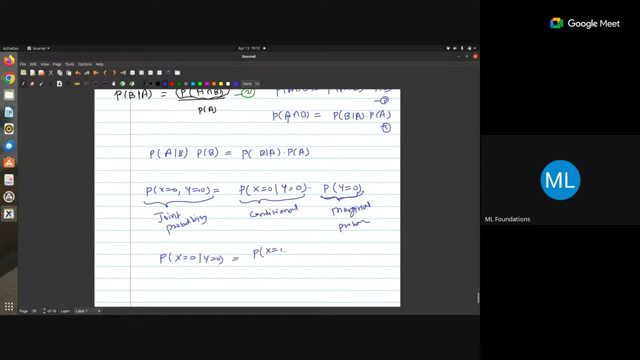 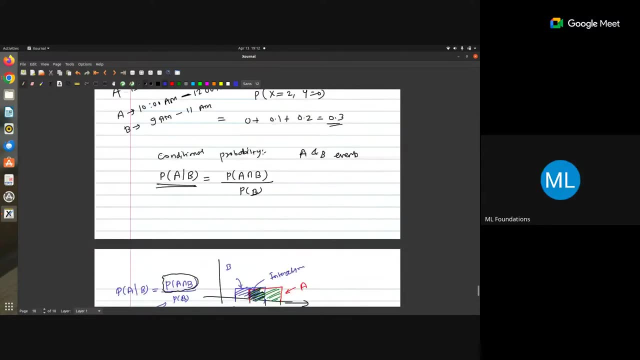 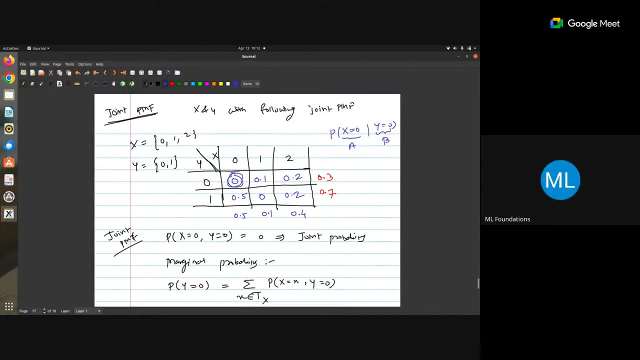 uh, which will be what probability? that x equals to 0 and y equals to 0 divided by the product. okay, so from this table, can you just tell me what is the conditional probability here? here, let's see. Let's say this is 0, right. 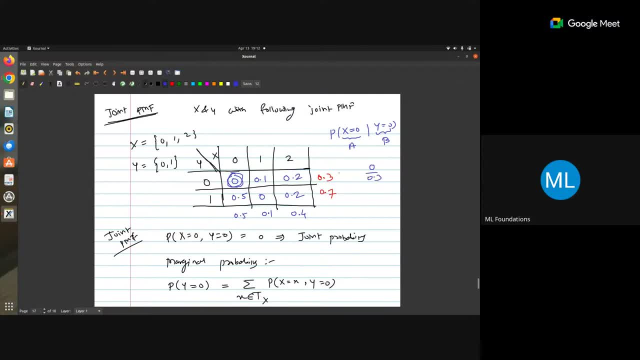 0 divided by 0.3, correct? OK, Y equals: this is probability that. OK, this is what probability that y equals to 0, right, And this is the joint probability, right? Are you guys able to understand this point? 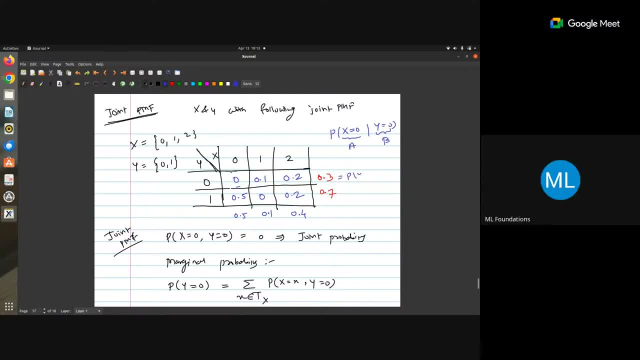 OK. So probability that y equals to 0 is probability that y equals to 1.. And this is what Probability: x equals to 0.. X equals to 0. This is marginal right. These are marginals. x equals to 1 and then x equals to 2.. 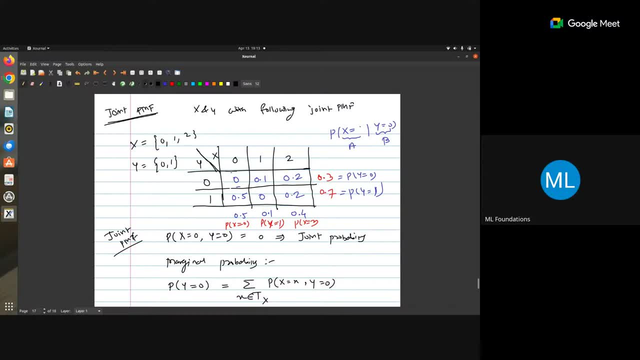 So instead of this, OK, let's try to find out some other thing. Let's say, instead of probability, that x. OK, I wanted to find probability that x equals to 1, given y equals to b. Consider these as events, OK. 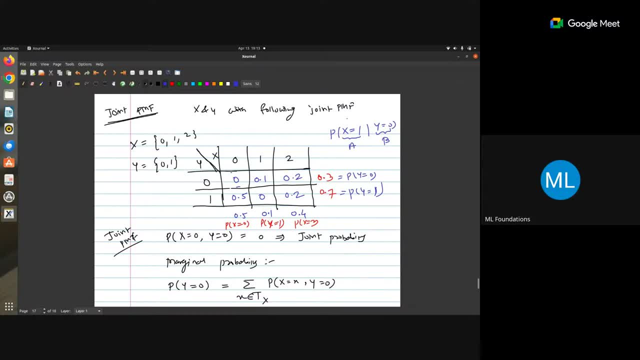 X equals to 1 is one event, Y equals to 0 is another event. So I wanted to find probability that x equals to 1, given that y equals to 0. So how do you find that So generally probability that A intersection? 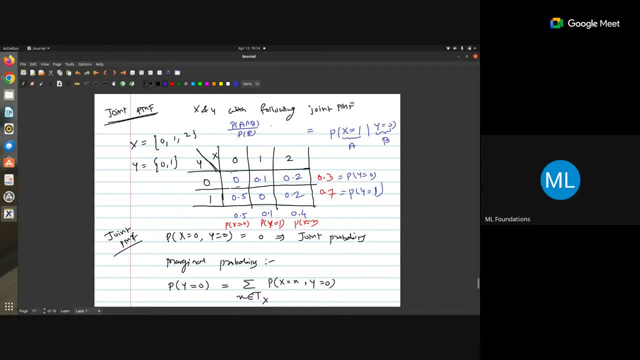 B divided by probability of B right. So, with this logic, what is it? Probability that x equals to 1 intersection, y equals to 0.. Y equals to 0.. Which value is this? 0.1.. 0.1. 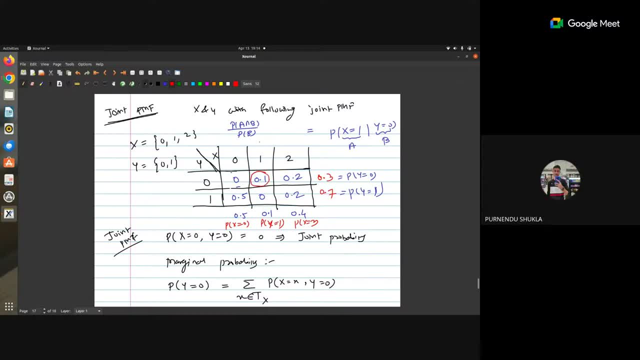 0.1.. And divided by Probability, Y equals to Y equals to 0.. So 0.3.. So this is 0.1 divided by 0.3, which is 1 by 3.. OK, 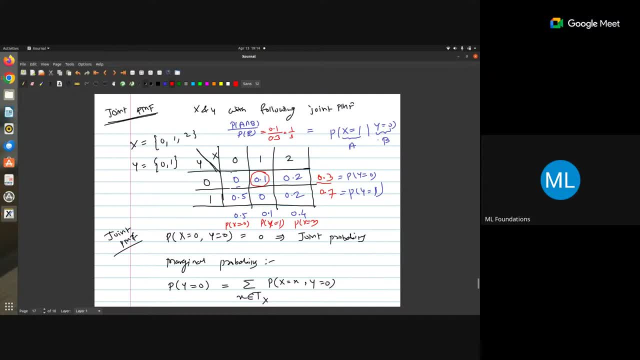 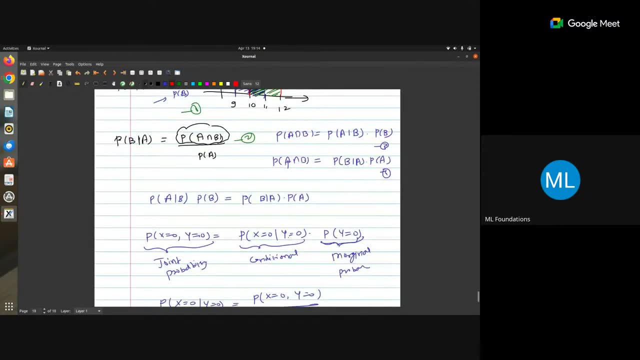 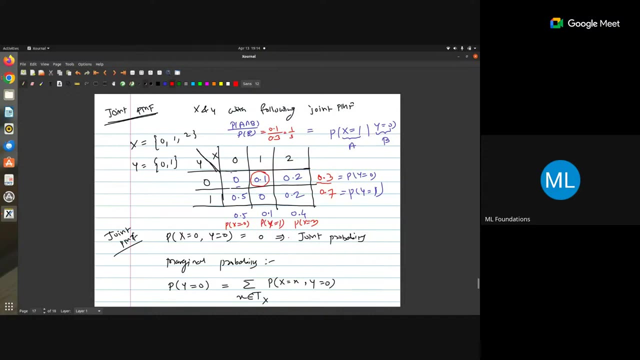 OK, Another approach of solving this is what? Because I already told you guys that this can be equal to, or maybe: OK, this is fine, This is fine, This is the way I can solve it. But OK, Suppose I wanted to find: OK, I think we have already discussed everything. maybe. 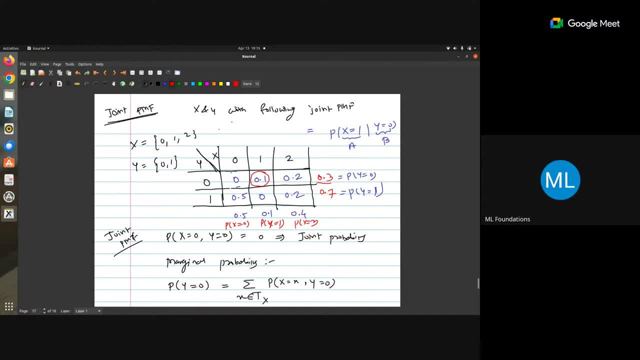 But OK. But if I don't have the probability mass function table here and if I have given that probability that x equals to 2 and y equals to 1 as 0.2, OK, and the marginal- that means probability that suppose x equals to 2 is given to me, x equals to 2, which is, let's say, 0.2, is. 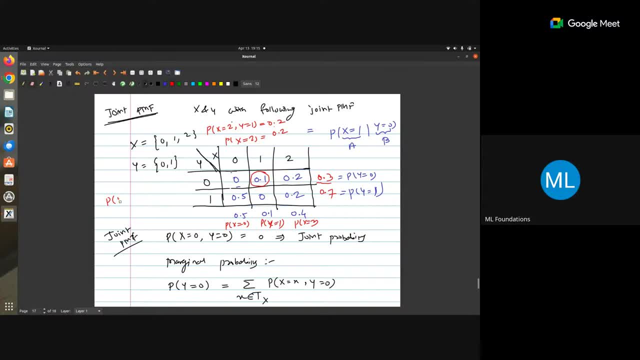 given to me. What is the probability that x equals to 2, or maybe x equals to OK, y equals to 1, given that x equals to 2 will be. x equals to 2 is 0.2.. 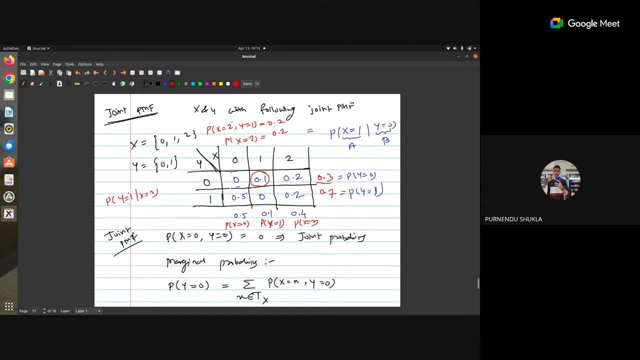 So denominator goes to 0.2.. For numerator: 0.2 by 0.1? No 0.2 by 0.. This is not related to this table. OK, This is a separate thing. OK, This is 0.2 divided by 0.2, right? 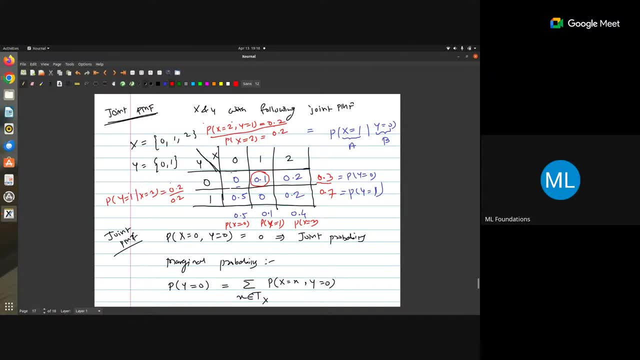 Actually this is like directly, this right which is equal to 1, correct? OK, It was not from this table. If I have to take it from this table, then it should be 0.4, because probability that x equals to 2 is 0.4 here in this table. 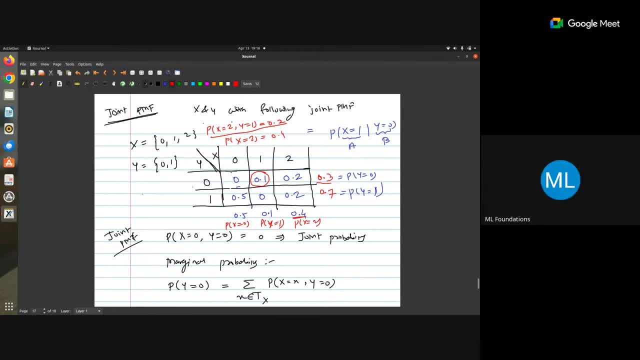 Then the conditional probability that x equals to 2, given y equals to 1, is 0.2. Understand, Actually, this is not actually very difficult to understand here, because if you see what is probability that x equals. So if I wanted to find probability that x equals to 2, given y equals to 1, or maybe y. 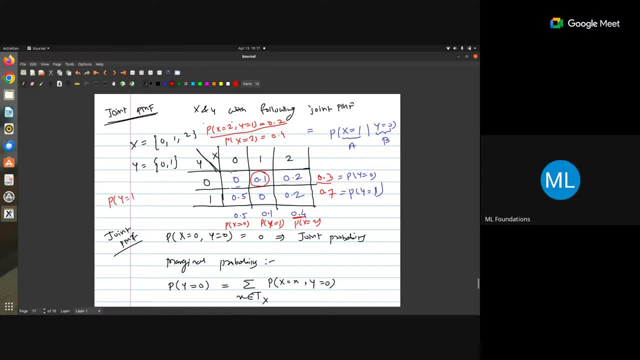 equals to 1, because if I wanted to find y equals to 1, given x equals to 2,, then I have to first of all marginalize this: What is x equals to 2?? Which portion For this table or the table? 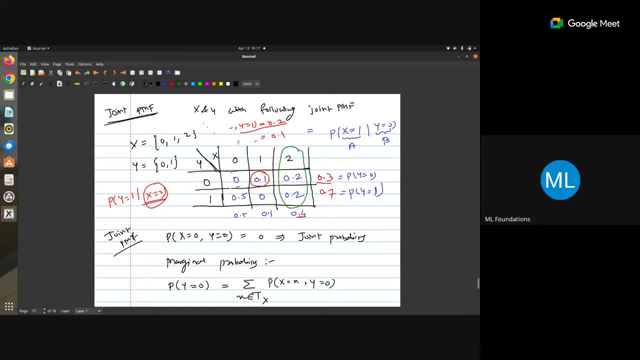 0.4.. 0.4.. This table Right. So I have marginalized this first right. x equals to 2. I have marginalized. Now I have to find probability that y equals to 1, which is this one. 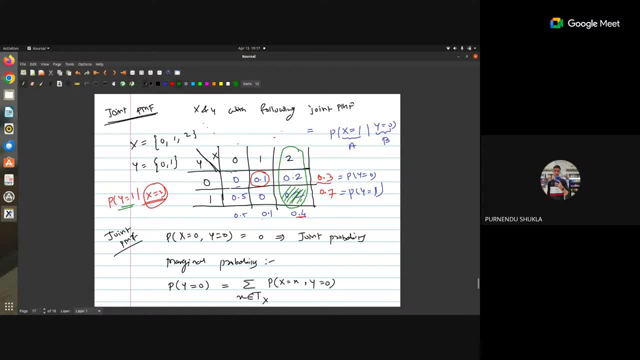 0.2.. No earlier question that you asked. Yeah, that was different. That was different. So how you solved that means you just did like 0.2 by 0.2. Because that is the formula right. 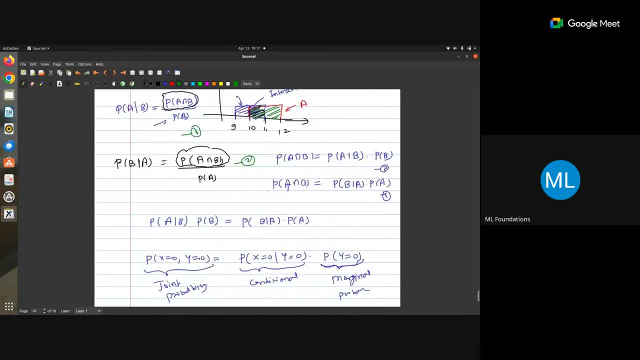 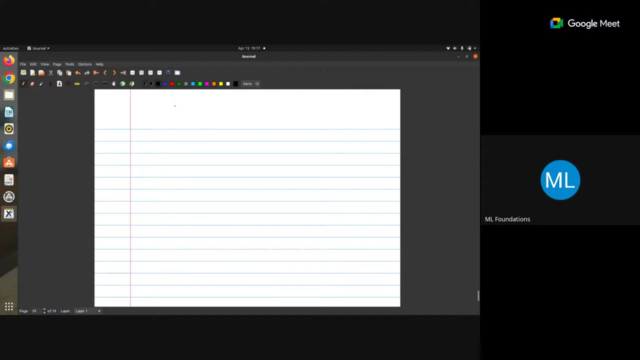 Yeah, OK. So this is how, let us say we let us solve some problem. Maybe I will give you one more table. I wanted to find you guys the values for it. OK, x, y is given. OK, Maybe I will give you some other thing. 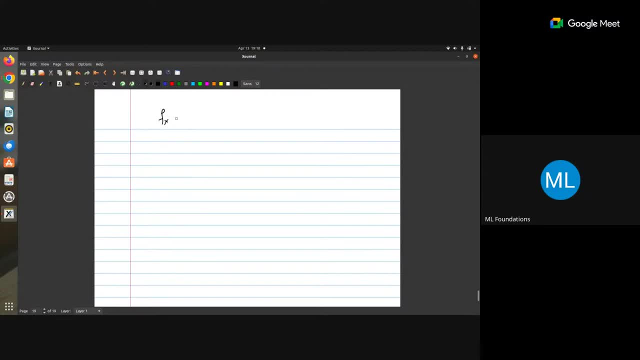 Suppose the fx of x is equals to 0.2.. Maybe if I subtract the fx of x, y, y equals to 0.2, then what is the fx 0.2.. 0.2.. This is 0.. 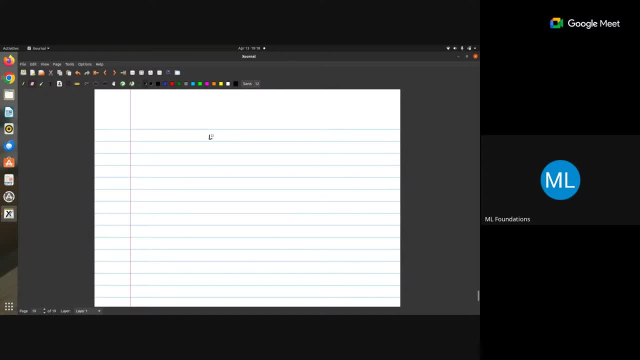 This is 0.. 0.2.. y is equal to 0.2.. This is 0.. 0.2.. x equals to 0.2.. So 0 is the fx for 0.2.. So that was 0.2.. 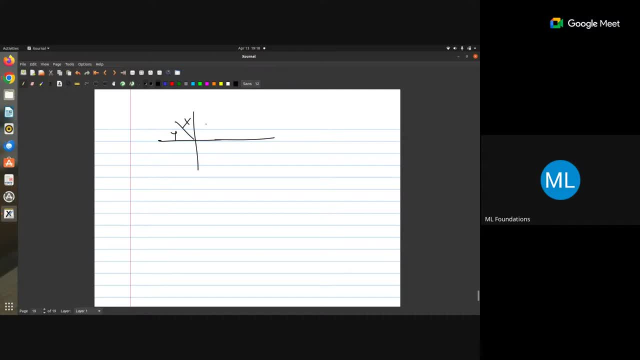 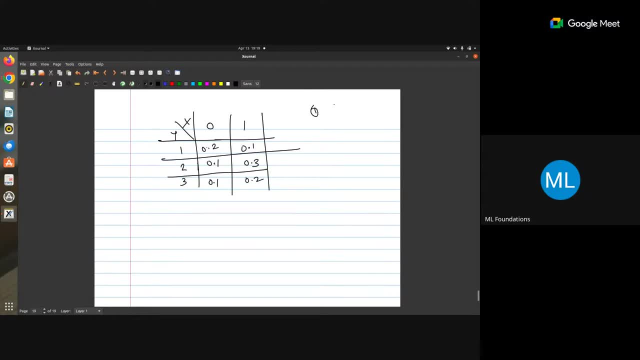 okay, I wanted to find you guys. first is marginal probabilities. second is conditional parties or all marginal on all condition. so take like two minutes to solve this and you, you, you, you, you, you, you. what we want to do is we want to. what we want to do is we want to. 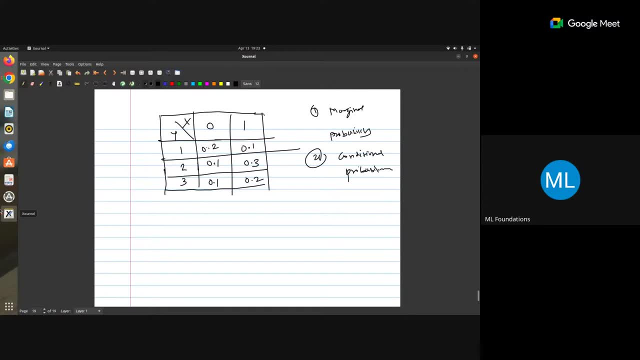 what we want to do is we want to make sure that the okay, so all the conditions, right, like, okay, can you just tell me one by one, and i'll ask you guys what is provided that x equals to zero? these are the marginal properties, right? the formula is summation: yeah, 0.8 point, yeah. 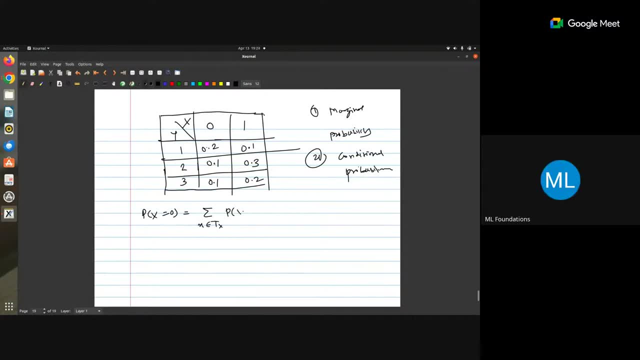 and provided that, uh, x equals, okay, so uh, it should be y across t, y. and provided that x equals to zero, y equals to y. right, that should be 0.2 plus 0.1 plus 0.1, which is 0.4. what is? provided that x equals to 1. 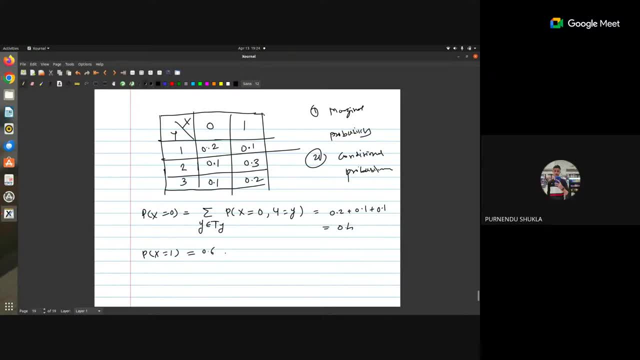 it is 0.6, 0.6, so you can under. one more thing you have to uh understand is the addition of probabilities across the range of x, right, the marginal probabilities. it should be equals to 1, right? so this, you see, this is 0.4. 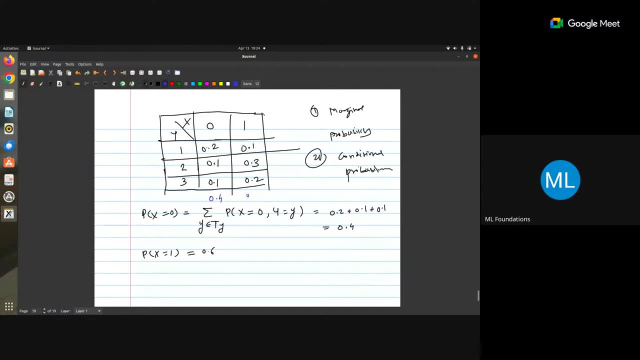 and this is 0.6 and that should be equals to 0.1. what is marginal probability? that y equals to 1, 0.3. here it is 0.4 and here it is 0.3. and if you add all, 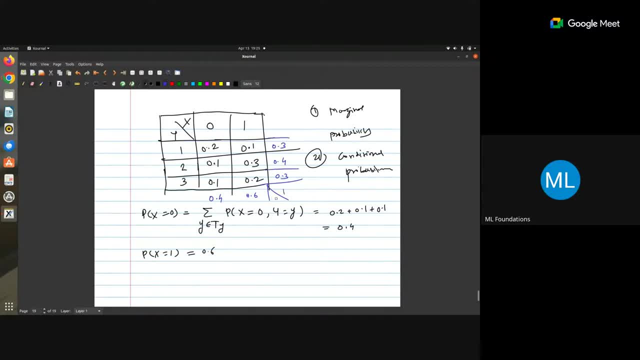 these things. across y, it should be equals to 1. okay, this is one, one more property. okay, what is the conditional probabilities? uh, what are? uh, like some conditional road. let's say, probably, that x equals to 0, given y equals to 1. 2 by 3, sir, 2 by 3 is nothing, but yeah, right. 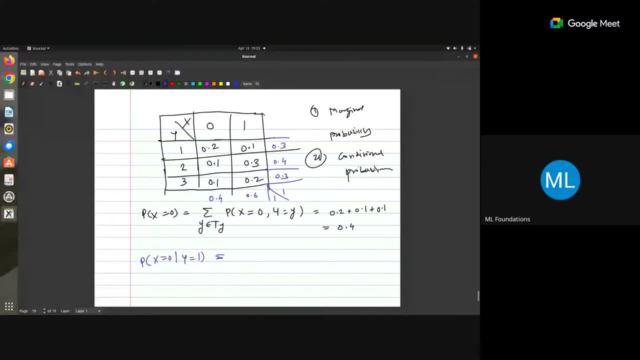 0.2, 0.3, 2 by 3, when x equals to 0 and y equals to 1, which is 0.2 right, and margin is across this range, right. so which is 0.2 divided by 0.3, which is 2 by 3, right, similar to what is, provided that: 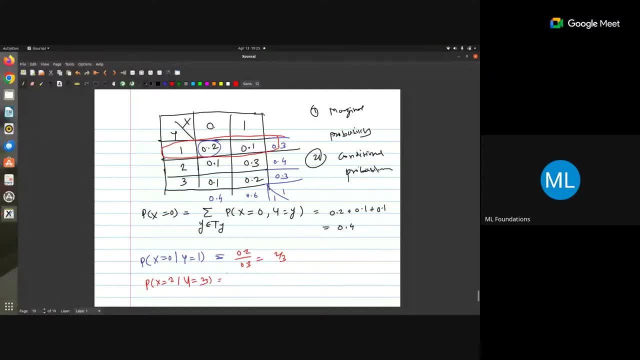 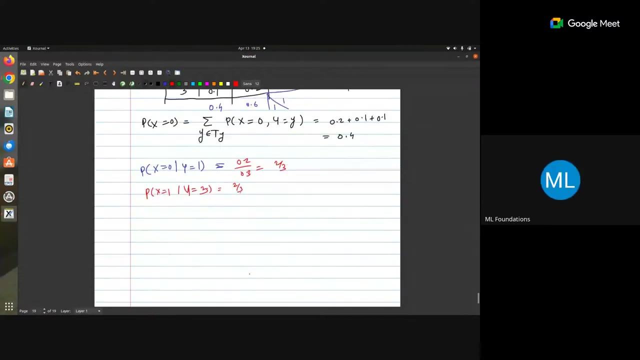 x equals to 2, given y equals to 3, so not 2. 2 is outside the range. x equals to 1, y equals to 3, 2 by 3, 2 by 3, right, okay, so you understand this point. so now, uh, let us now, let us just see how the 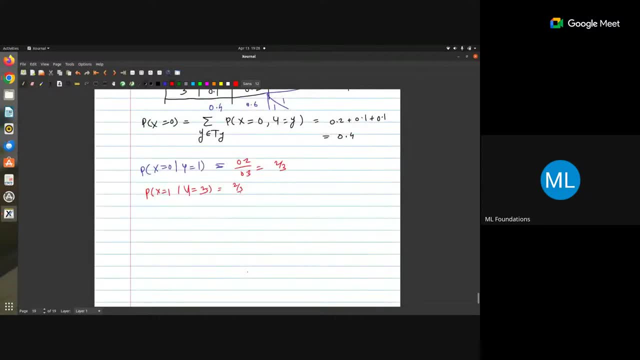 say, I wanted to use this same thing for the continuous random variables. So in continuous random variables we use the same technique. The only difference here is what In continuous random variables, instead of summation, we use integration, right, Yes, 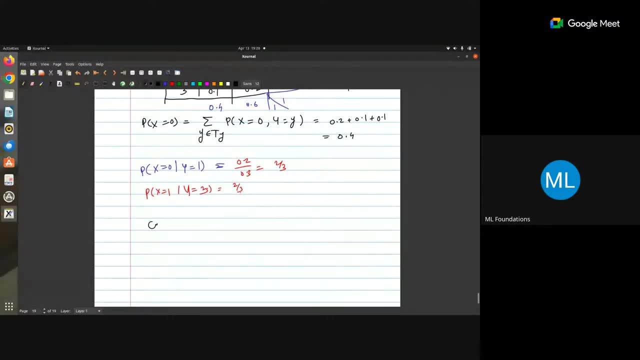 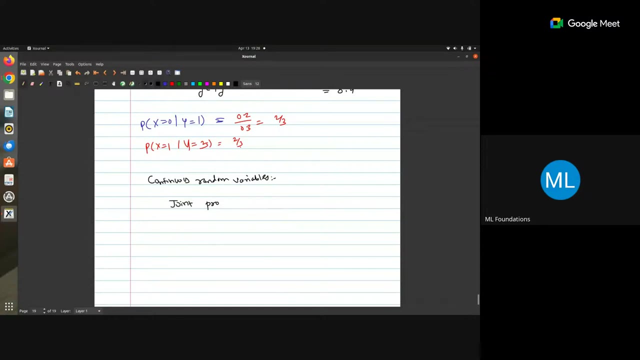 And in continuous random variables. OK, in continuous random variables the joint probability is defined by fxy right, Or defined or represented by: OK, This is joint probability is represented by fxy of x, comma, y. OK, So suppose if it is, some function is given right. 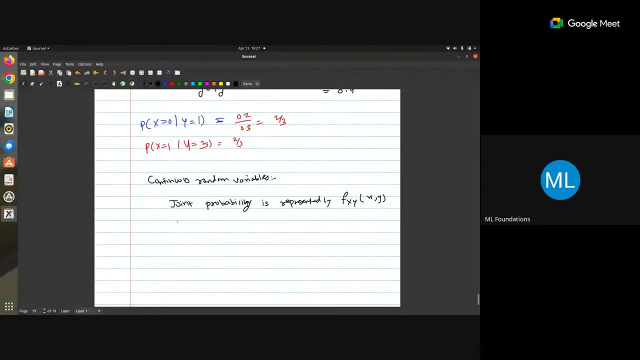 So fxy is basically a function, which I can say that this is a joint probability. What do you mean by joint probability? It's an intersection between two random variables. Or I can say that: What is the function, What is the probability that these two, the values taken? 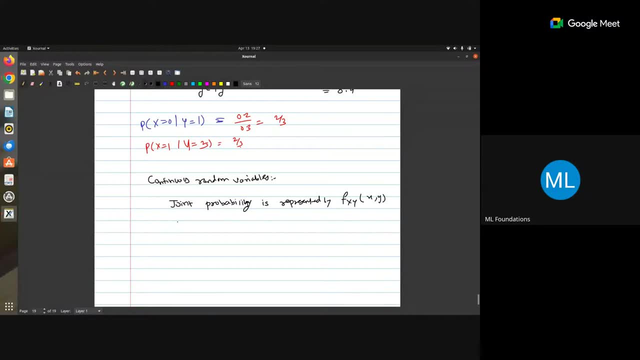 by this random variables, which are, you can say that these two events occurring simultaneously. right, That is a probability. OK, Then, in this case, the marginal probability which is denoted by fx of x. this marginal probability, fx of x. 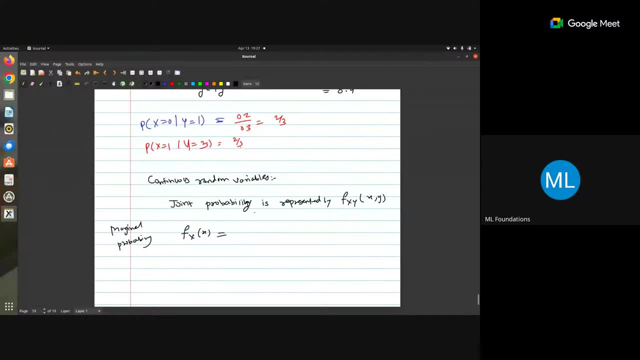 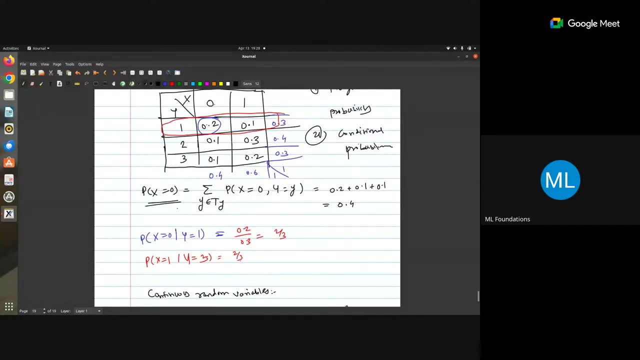 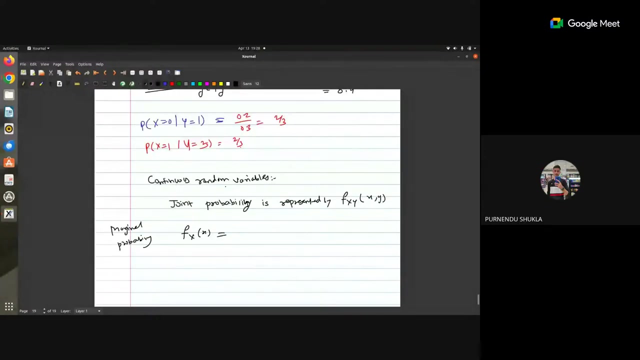 is given by what. So here, what was the? How did you find out? the marginal probability of x equals to 0, treating x as constant and summing over y right, Correct. So in this case, here, what did you? 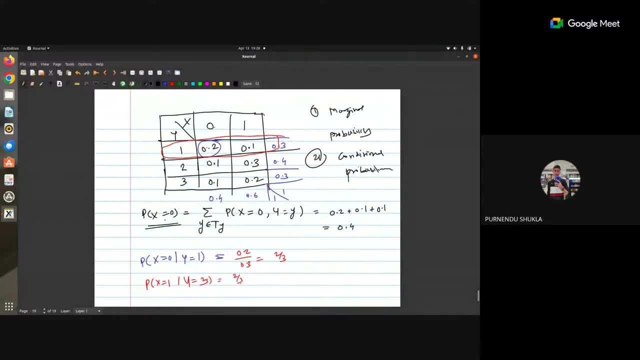 do for finding the marginal probabilities. We did a sum, Yeah, but by treating x equals to 0 as constant, right? Mm-hmm? OK? And summing over the range of y when I wanted to find the marginal probability for x, right. 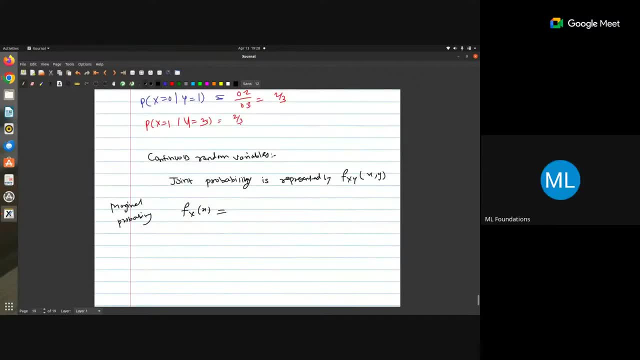 So here, if I wanted to find the marginal probability that at some x, what I have to do, I have to sum over, Integrate over all. Sorry, integrate over y, All y, All y, And what I have to integrate. 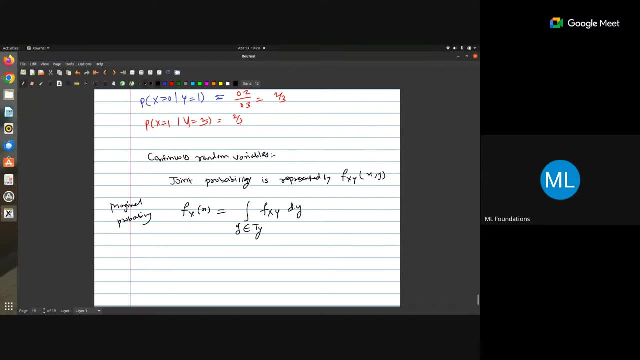 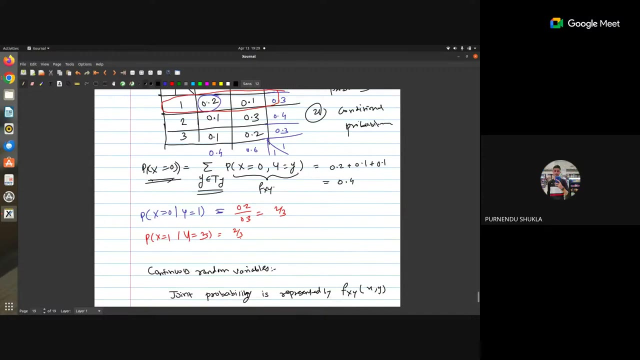 fxy, dy. Right. Why should I use dy? Because I'm integrating over a range of y and treating x as constant. Here also, you can see that. So in this case, only how we will solve it right. What happened? 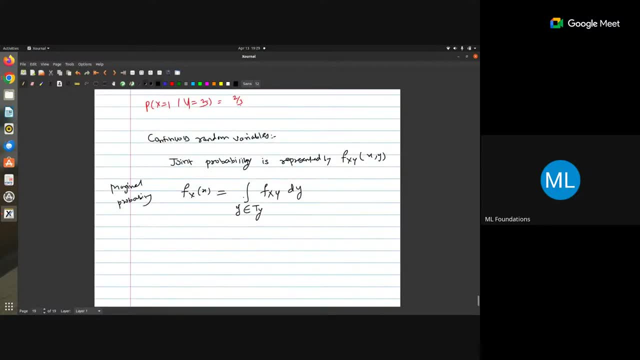 I'll show you. I'll show you. I haven't taken any example yet, so I'll tell you how to solve this anyway. So OK, but you understand this point at least. I fixed y. Yeah, I fixed y. And if y of y is x as constant, sorry, treating y as constant. 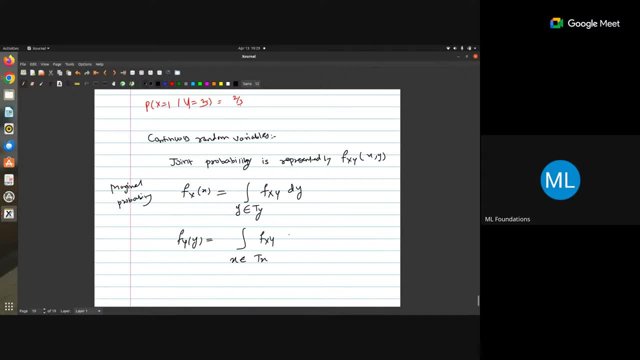 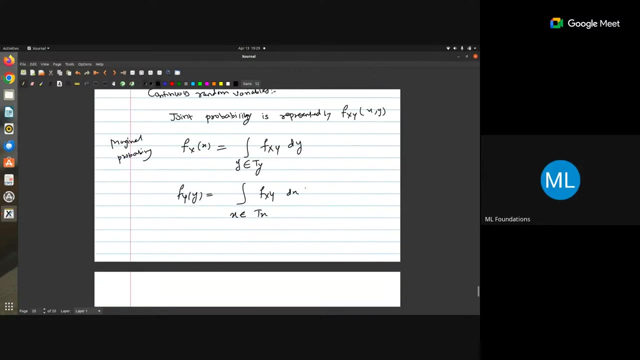 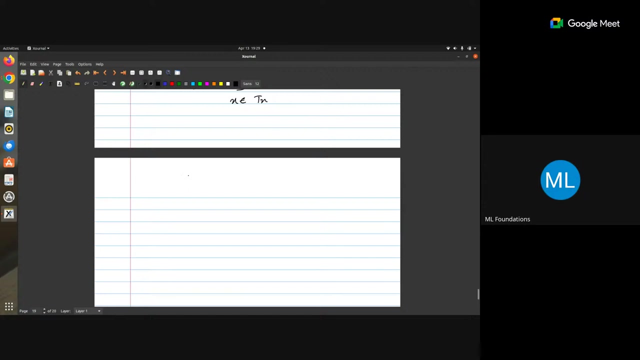 and summing over the range of or integrating over the range of x. OK, This is the definition of marginal probability: dx, dx, Right, Mm-hmm, OK, Yeah, Yeah, OK, Then conditional probability in this case will be what? 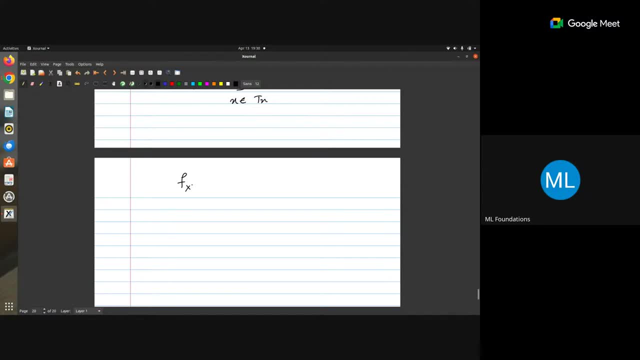 Then let's say: if I wanted to find the conditional probability of x- let's say x- at some x given y. Or I wanted to find the conditional probability of x given y equals to some small y, How should I find it out? So conditional probability is: 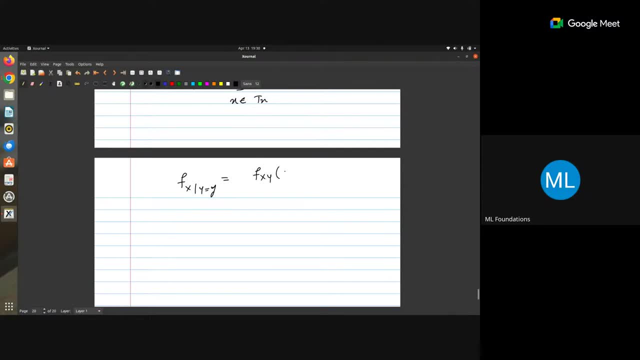 Yeah, But the joint probability divided by Marginal, Marginal right, Mm-hmm For joint, how will we solve? it OK, so can we have any example from maybe practices in mind or something? Practice assignment. 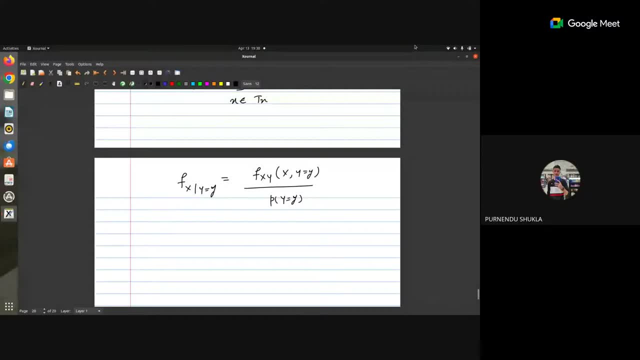 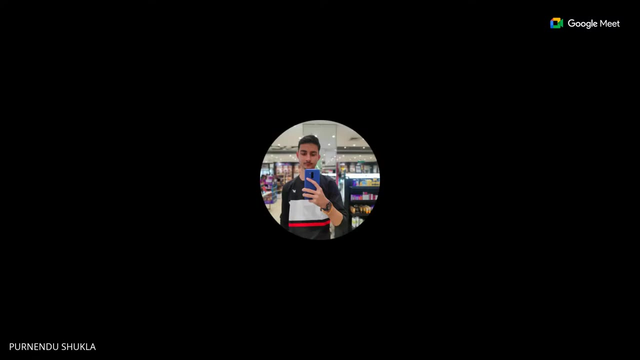 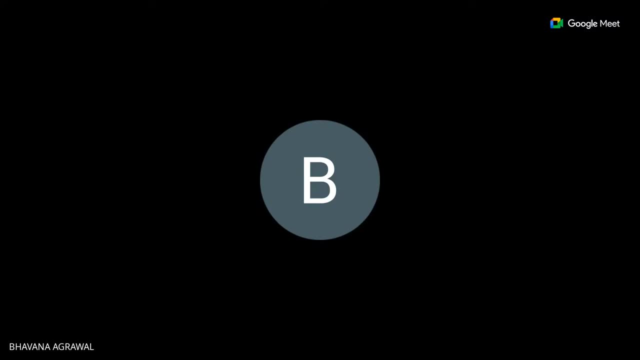 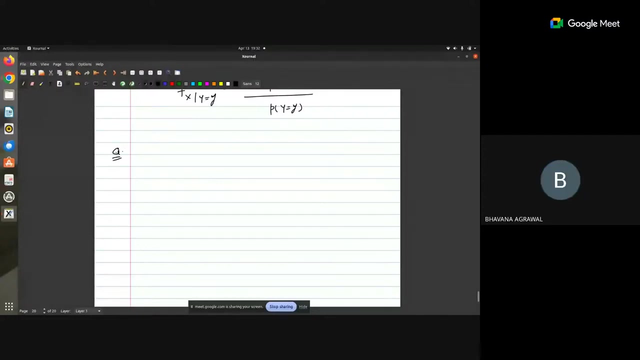 find probability of X less than equal to 2 by 3, given that X is greater than 1 by 3. okay, so can you just tell me what is the problem? let X have following PDF. then find probability of X less than or equal to 2 by 3. 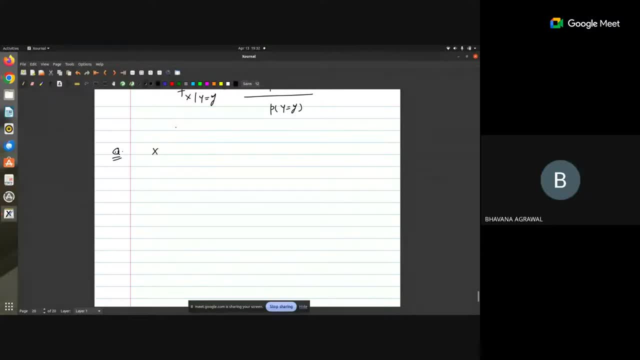 okay. what is the PDF? PDF or is FX of X- 3? X is square for 0, X is 0 to 1 or 0. otherwise, this is okay and what we already I'd find out is fine. probability of X is less than or equal to 2 by 3. given that X is greater than 1 by 3, this: 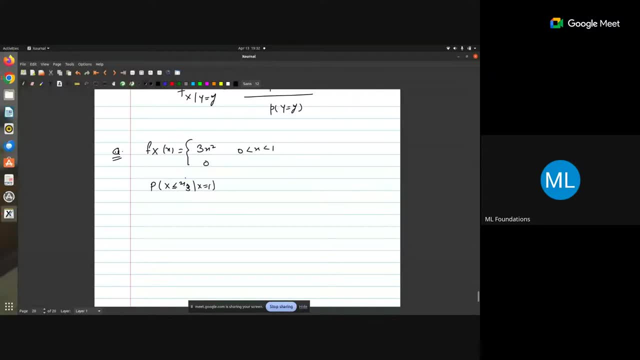 is not a joint, this is not joined to 1, right, this is normal. okay, let's let's take one example here itself. but we have sorry, this question that we wrote is a conditional question is conditional quality question. let me just try to come up with some. suppose this kind of is a. 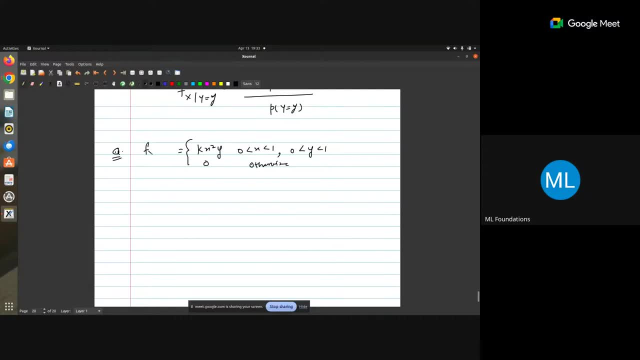 uh, joint probability distribution given to you. okay, say, x, y of x, y, this k, x square y, and i have to find the marginal probability and the condition probability, for example, suppose. so in this case, how to find out this? first of all, i have to check, i have to find the value of k. yes, so how to find? 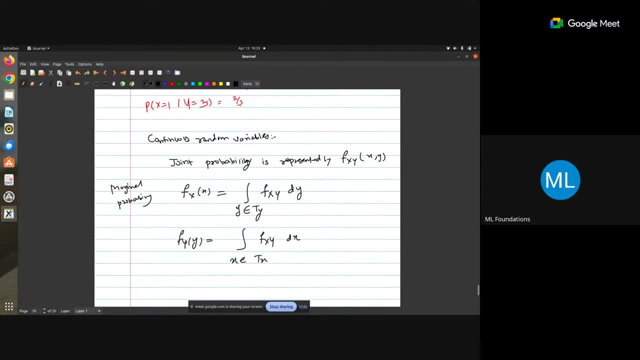 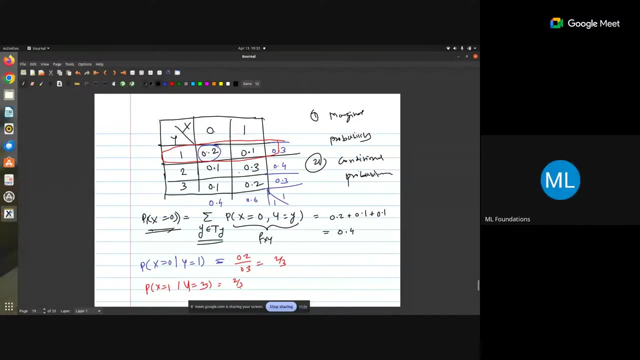 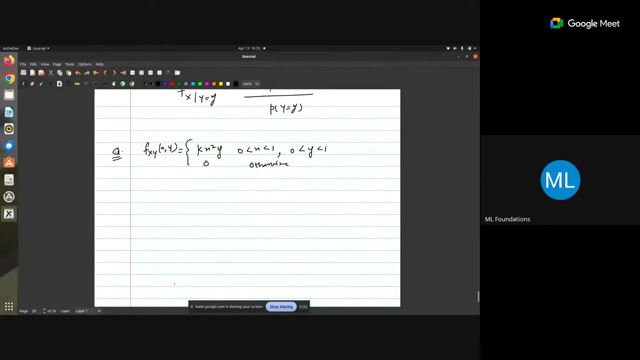 the values, because from pmf we have seen that the all the joint probabilities, right, the sum over all the joint probabilities equals to what one? okay, so i'll use the same thing. and what does that mean? so there you used to have- uh, i used to do the sum. here you have to use the integration, right. 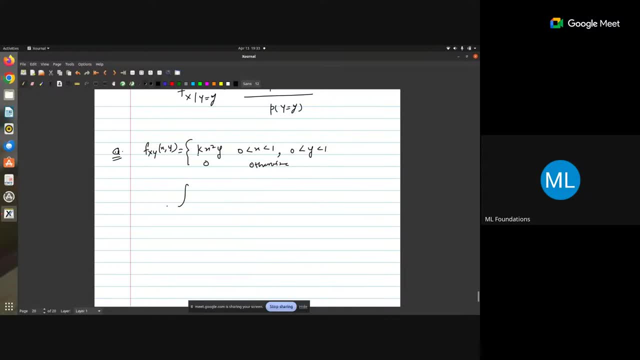 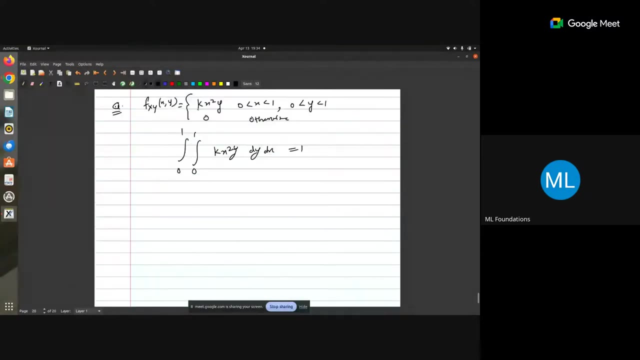 and integration over the range of x, which is zero to one, and zero to one for y, fx square uh, y. so there is fxy of x and it's a dy dx and that should be equals to one, right, okay? so k x square y dy into dx, it should be equals to one, uh, now let's say what is the. 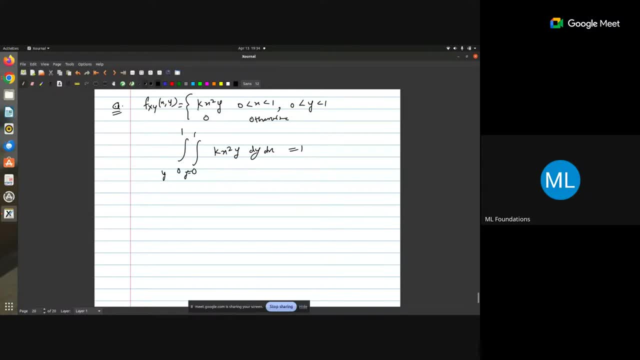 integration. so this is y equals to zero to one. this is x equals to the constant right, k is a constant. we have to find out. yeah, that is okay, so we can just take: let's say out, uh, and let's say x equals to zero. first of all, i have to integrate with this to y, right. 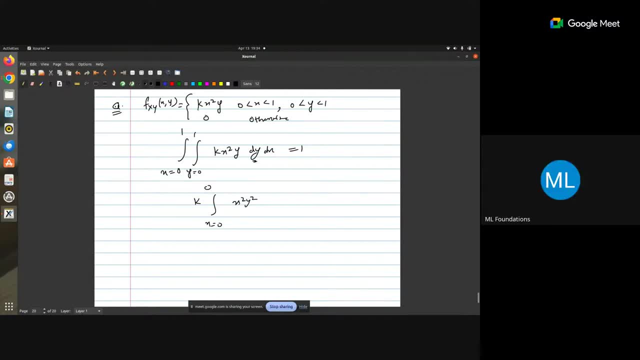 uh. so then it will be square. y square by two, from zero to one. dx equals to one and again uh. so x square into what is it? uh, one minus zero. so x square is equal to six. zero to one, right um and k is equal to one. so this x cube by six, right from zero to one, okay, one which gives me k equals. 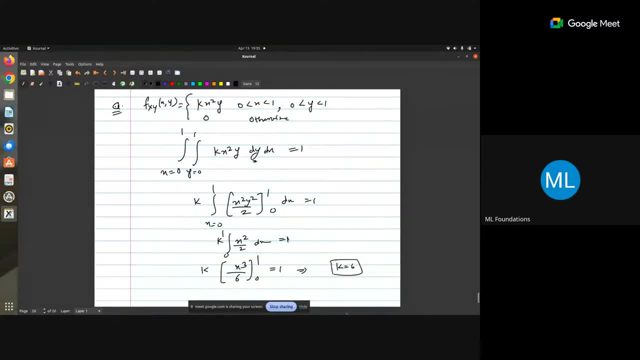 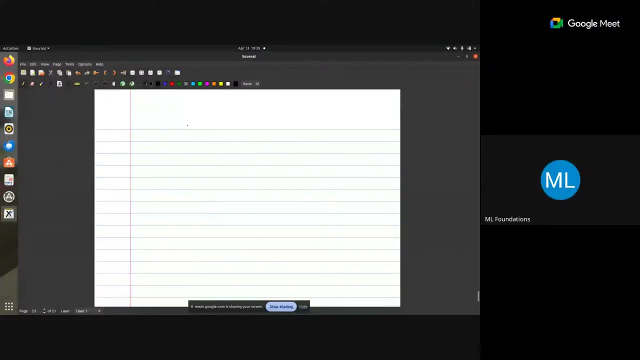 to six, right, so my joint density function here is six x square. yeah, so f x y of x comma y is becomes six x square y. uh, where the range of x is this, range of y is this zero. otherwise right now i have to find out. uh, the marginal of y. okay. 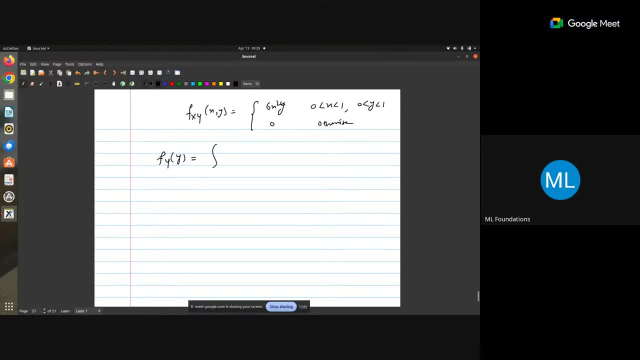 for what? what i have to do? i have to integrate over x, right, like this range of x: yeah, from 0 to 1, f x, y d x, which is 0 to 1, 6 x square y d x. now, this is 6 x cube by 3 y, 0 to 1. 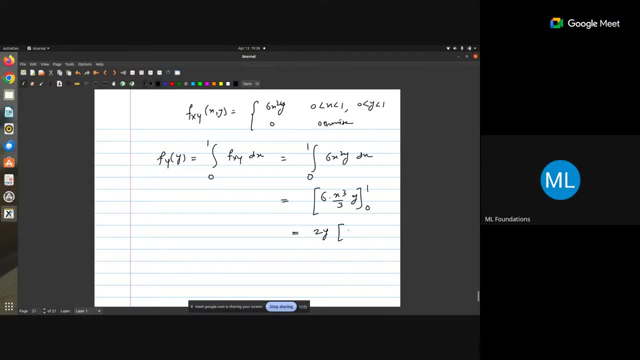 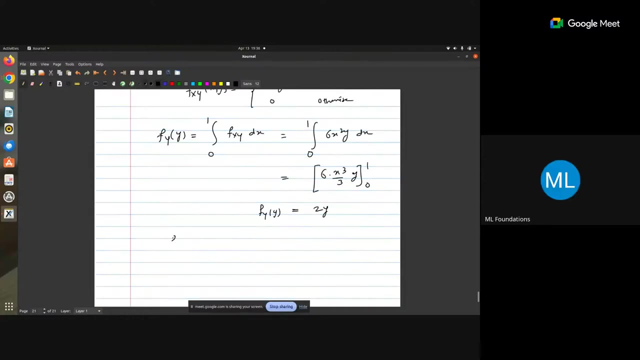 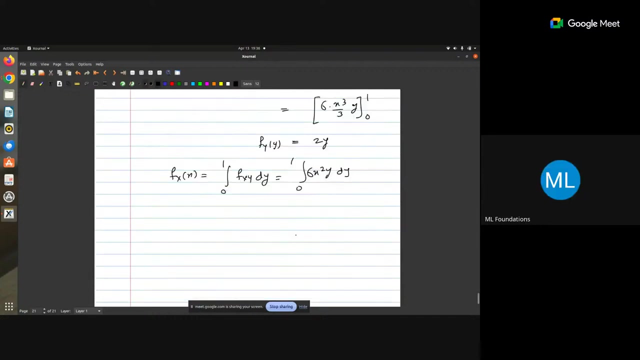 so there is nothing but 2 y and 1 minus 0. so that is 2 right, 2 y right. this is my marginal density, correct? this is my density for y. similarly, what is marginal density for x? this will be 0 to 1 f x y of d y. so that is 6 x square y, d y over the range of 0 to 1, and that. 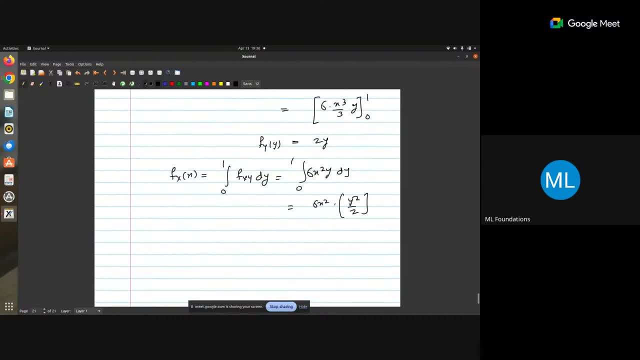 that will be 6 x square, y square by 2, from 0 to 1, and so that will give me 3 x square. so you can see that f, y of y is marginal, density of y is a function of y and the marginal density 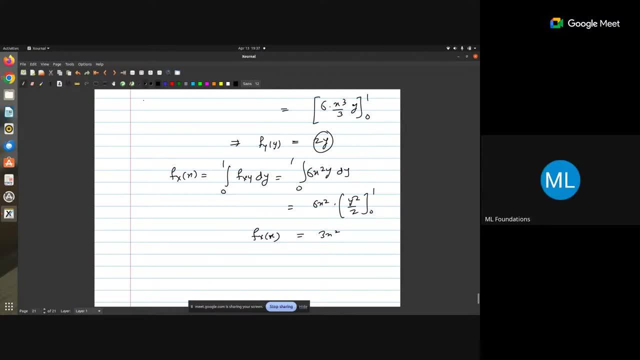 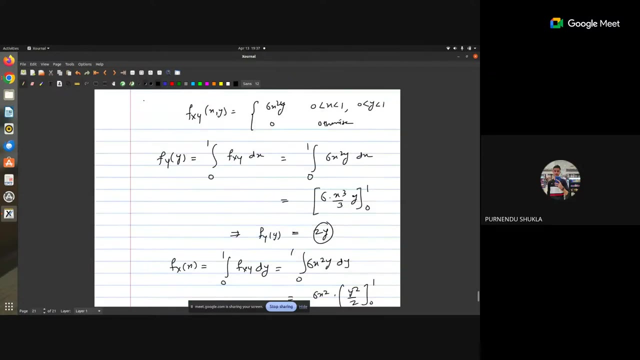 of x is a function of x, so you can understand that if we tweak, that means whatever range is there. say, let's take n up to less than it means. can you scroll a little bit up? i want to change a little bit. say: for 0 to x to 1, okay, but for y, 0 to y to n, some value and 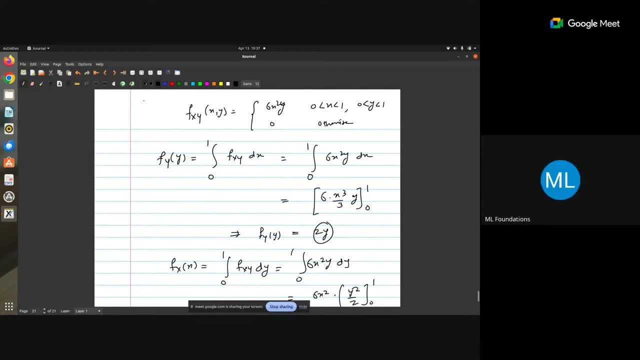 in that case how our approach will change. it can cannot be n right, like it should have some value right, or it may be infinity, and n cannot be like you cannot have something, uh, some variable. we can't have no range can range cannot be in a variable right, then that will make another like. 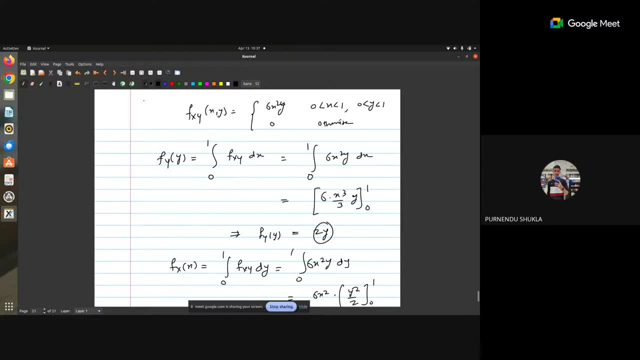 find the value of k or n for n where? where? no in the range? how can you have the way where the support is clearly clearly understandable? right, you cannot define a support. right, support should be there. it can be infinity, but it should have some value. right, it cannot be zero and not something it can. 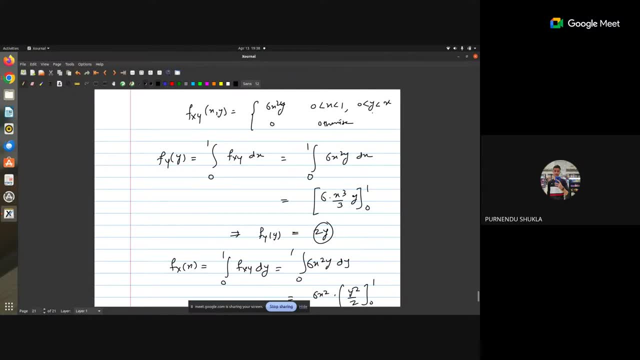 have this, this also. zero to x also is fine. that thing, that thing. zero to x, that is okay. this is also fine. it's like just integration. you can do it instead of y. we can do like zero to x. yeah, you can do that right. so that is, then it will be a. it will also have a function of x and it will be a. 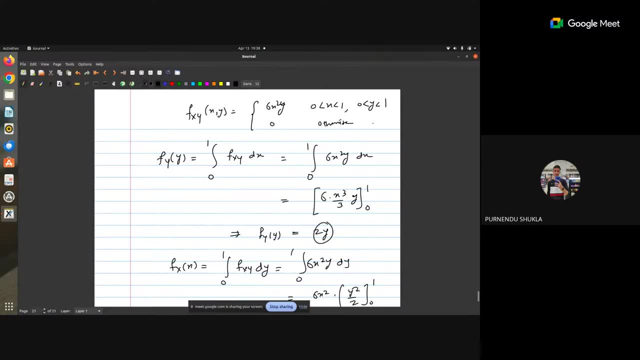 function for the marginal density of y or for x. we will have, uh, x part also there, right? yes, yes, okay, so no, i'm, i'm not going into that because we, uh, we have to finish the transform random variables, right? so that's why i'm just once, i'll finish these topics. maybe we can have some. 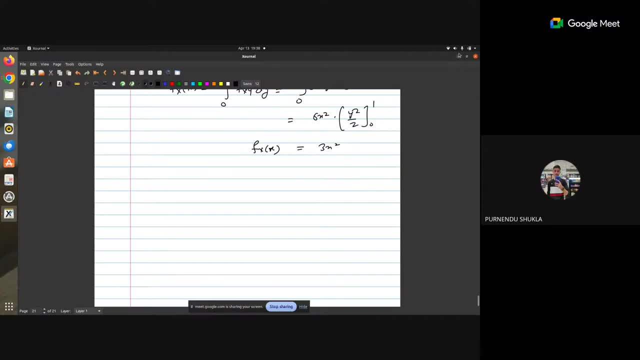 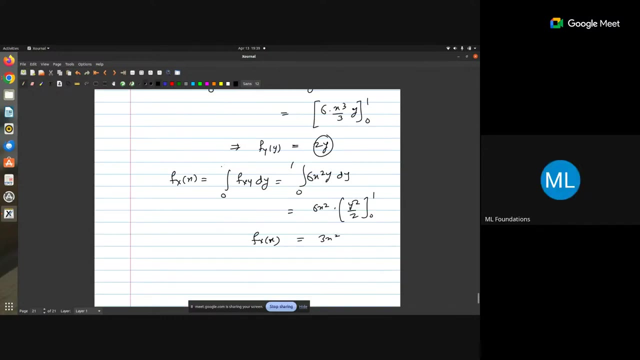 little more time. i'll try to solve the problems. okay, the value is y, 0 to x. then we put the value of x- now not here- from zero to one. if it is there, then you have to. uh, but this is not the case here. okay, that time it will be. 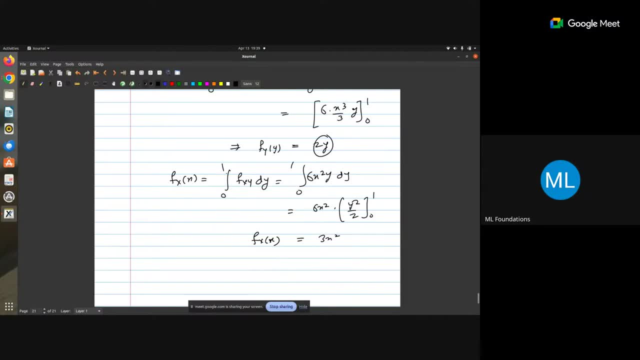 the kind of problem will be different than this one, then you will not be able to find maybe the marginals there, right, because here it is a dependence. so i'll talk about dependence first and then you can understand what is dependence and what is the independence, right. 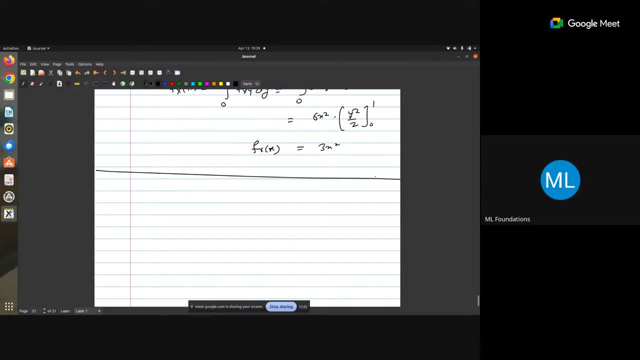 okay, so first of all, uh, let's say if, if the two variables, x and y, if they are independent on each other, or if they are not independent of each other, how to find that, if the joint density of two variables is equals to the product of their marginal density, if this is the condition? 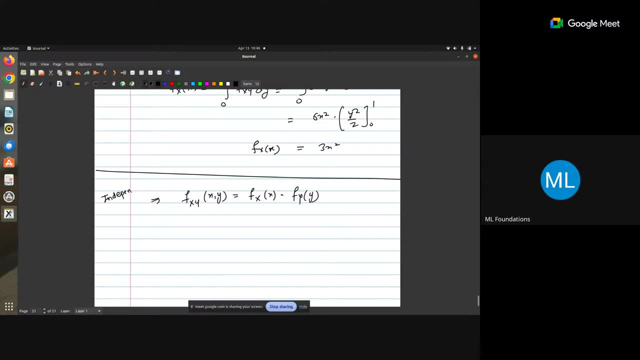 is that this condition is there. then the two variables. i can say they are independent of each other, equal, then independent and not equal. and dependent, not equal. if they are not equals to each other, then they are dependent. they are dependent. okay, this holds true for this also. the 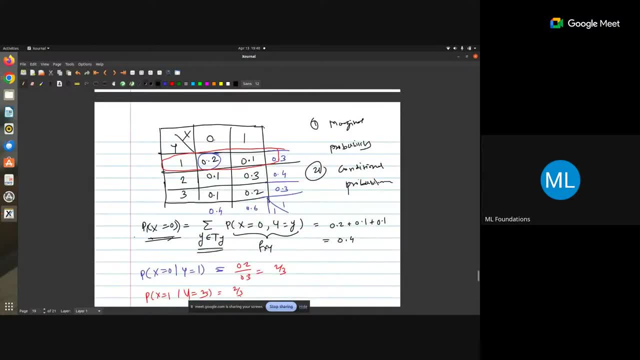 pmf. so here, can you just tell me, uh, whether x and y are dependent on each other or not by using the same definition? no, sir, it is dependable. dependent, okay, how you, uh, how you can find this, like, let's say, 0.3 into 0.4, right, if i multiply? 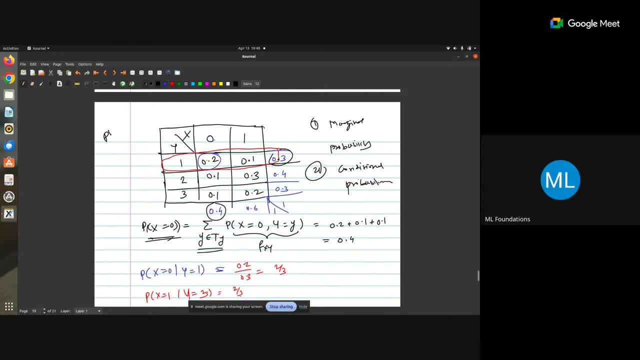 this. uh, what does that mean? uh, i, i'm multiplying provided that y equals to 1 into probability that x equals to 0. the multiplication is giving what 0.4 into 0.3, which is 0.12, right, and that should be equals to of what probability that y equals to 1 and x equals to 0. that means this probability. 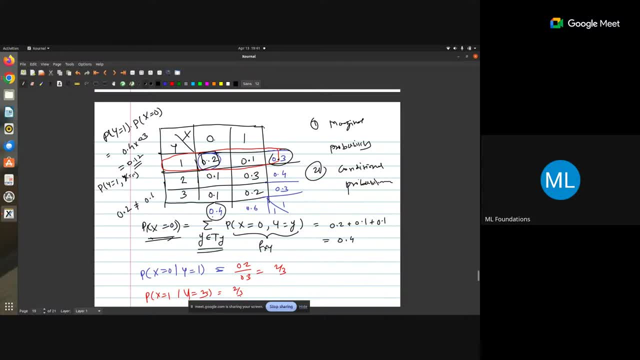 0.2. so 0.2 is not equals to 0.12. that means they are dependent. they are dependent, okay. so that means in pmf table you have to check for each and every value of x and y. then only you can find out the dependence there, okay. 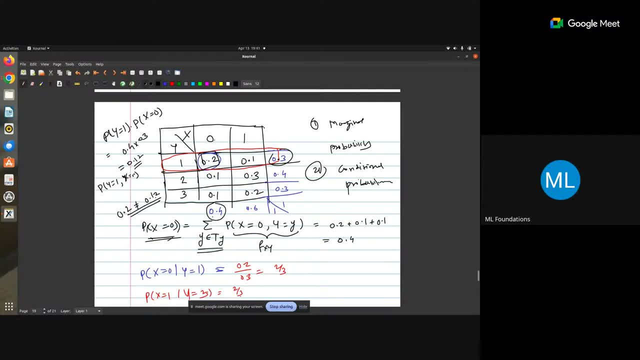 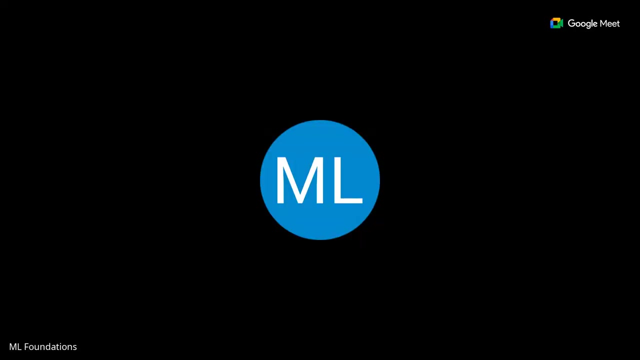 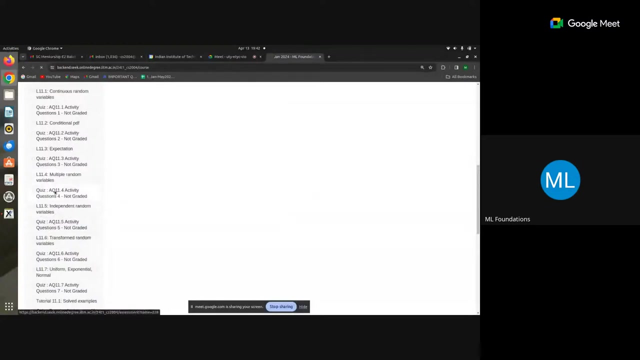 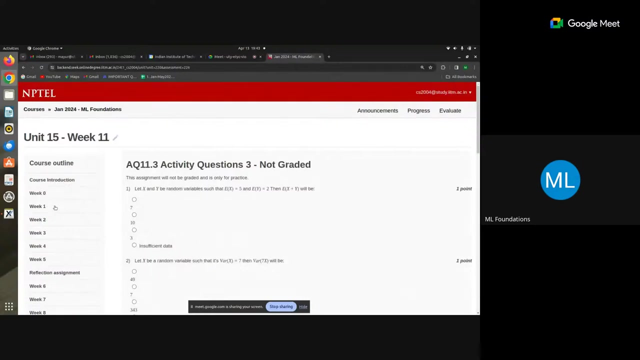 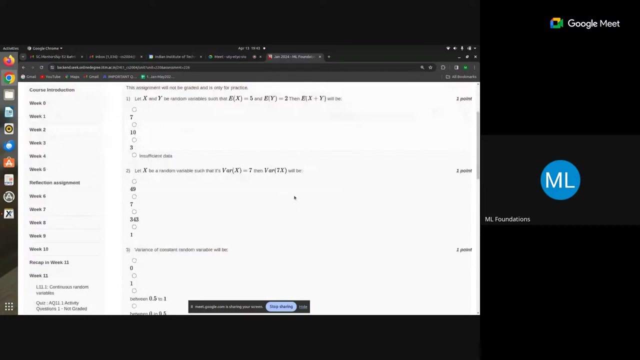 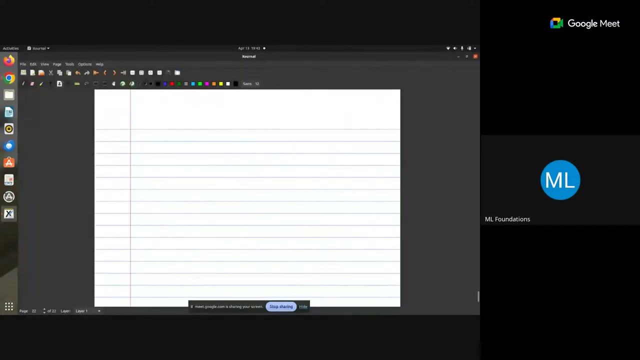 so okay, so, yeah, uh, so this is, uh, dependence, independence, okay, uh, so let's see if you have any. let's see if you have any, let's see if you have any expectations, expectations, expectations said so, there are some properties, uh, which we have talked about. so if there are two random variables, uh, they know what is the expectation of if there are two? 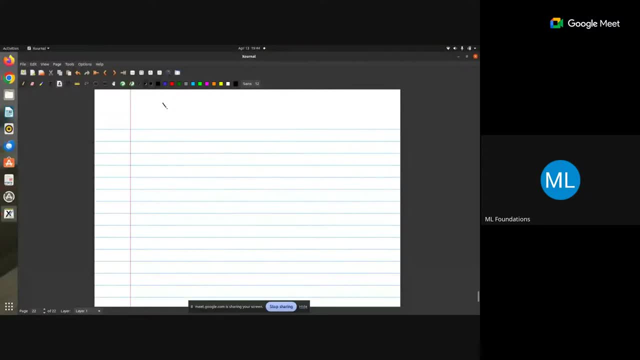 two independent random variables. right, ok, if x and y are two independent random variables, then expectation of x plus y can be written as: what expectation of x plus expectation of y? ok, ah, but in this case how to find what is expectation of x in if this two are continuous? 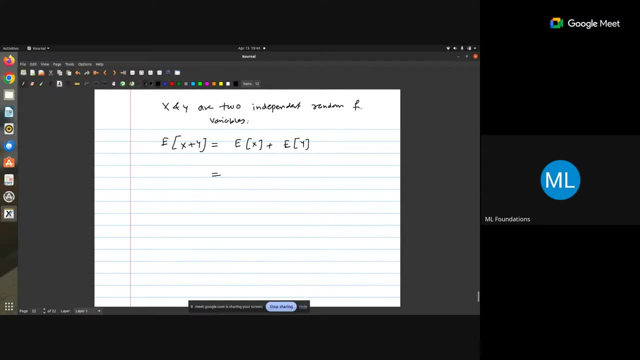 random variables, ah, and you, you have given the joint ah density of x and y. the expectation of x can be written as what integration, integrating over that range of x, say x, or the range of x, ah, into what x? into f, x of x, right? so f, x of x is what marginal, marginal and ah, you know how to find. 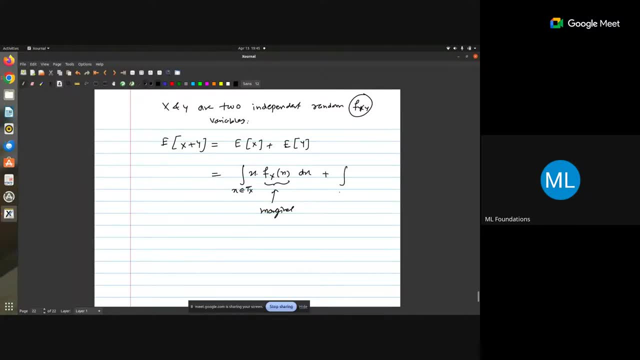 the marginal density correct. so this is ah. y belongs to t, y, and here it is y into f, y of y d y. so f x of x can be found out from, and here it is y into f. x of x can be found out from, integrating over y, f x, y of x, y d y. 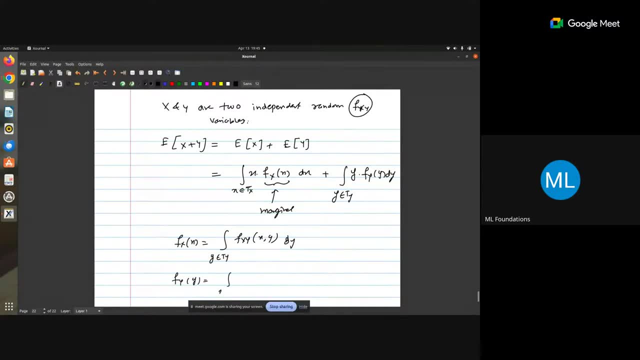 right? and f? y of y can be found out from x, right? so if i want to, if i ask you to find what is the expectation of x by giving you the joint pdf, then how will you deal with this? uh, i hope that we have everything, okay. 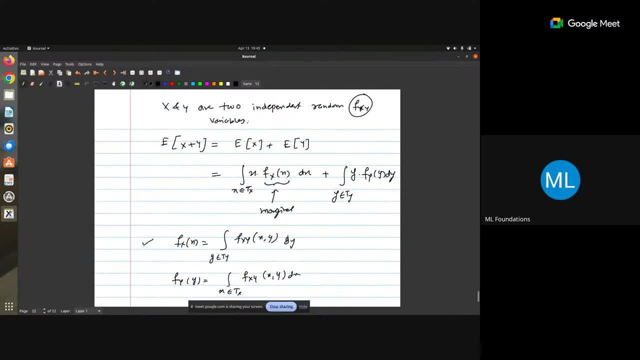 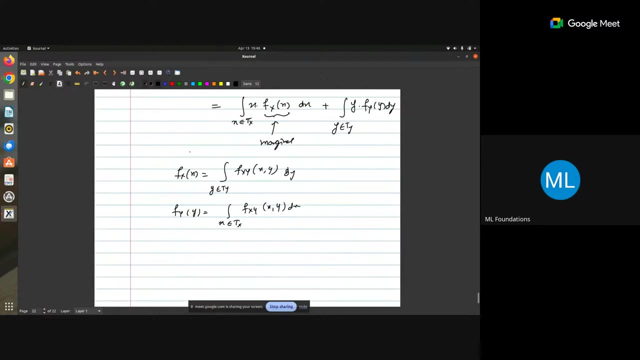 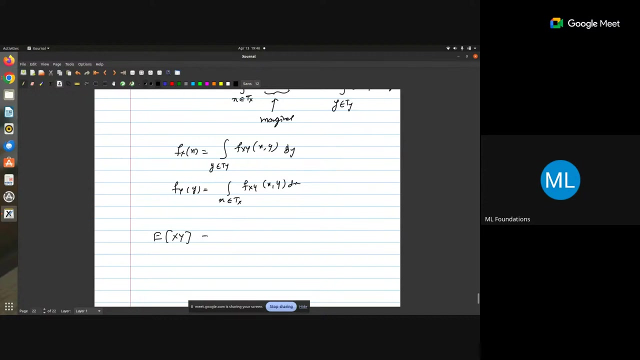 proceed you just? first of all, you will find out the marginal density of X and then you'll find out the expectation by the regular formula, right, okay? okay, one more property of expectation of. if I wanted to find expectation of X into Y, so if they are independent, I can write it as expectation of X into expectation. 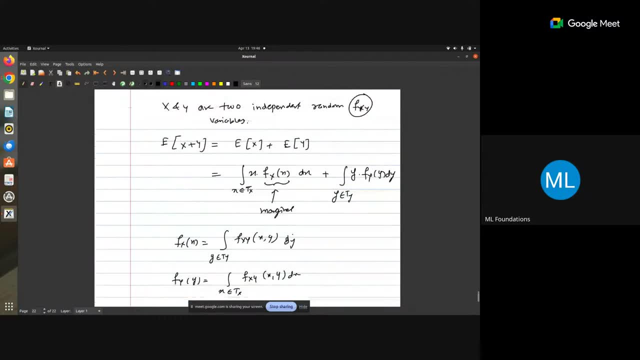 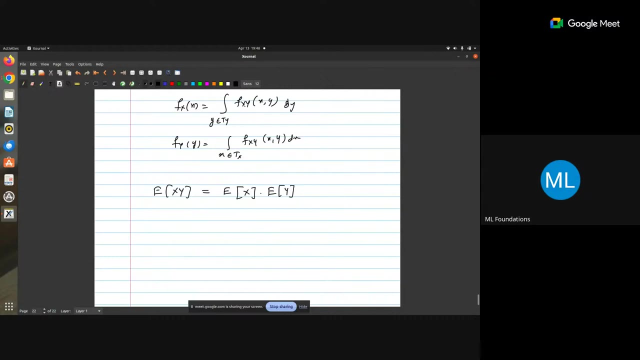 of Y. okay, so this property- expectation of X plus Y- this is fine. this will work fine for a dependent random variable also. but expectation of X and Y will not be equals to expect of X into expectation of Y if X and Y are dependent. so this property only holds true only for 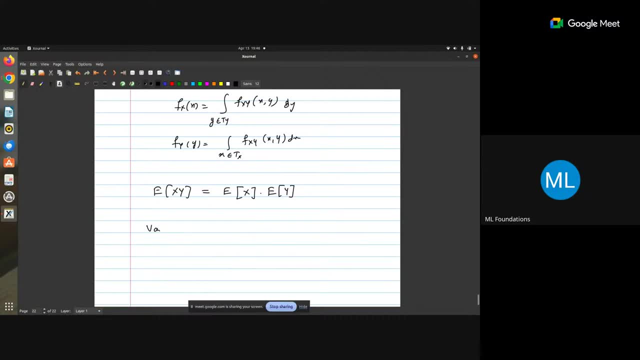 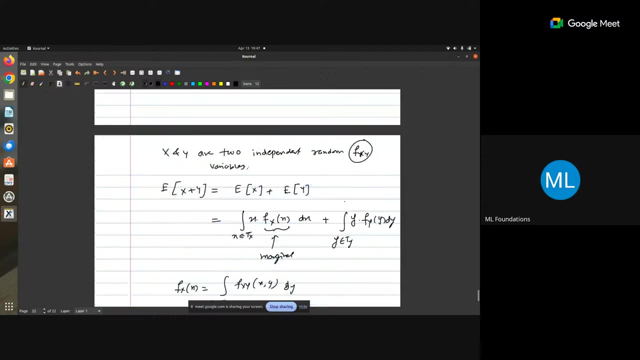 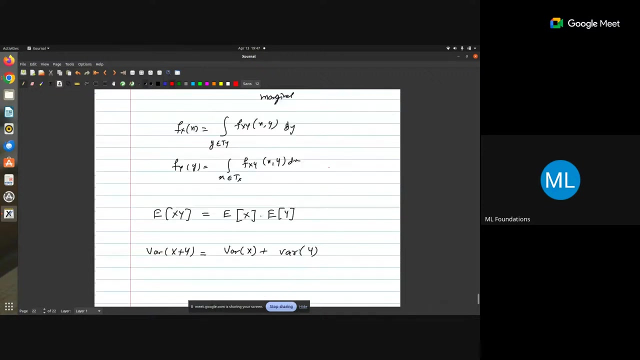 independent random variable. similarly, if I wanted to find variance of X plus Y, how to find the variance of X plus Y? it is nothing but variance of X plus variance of Y when the, when X and Y are independent of each other. okay, so all these properties are for independent random variables, okay. okay then what about this? 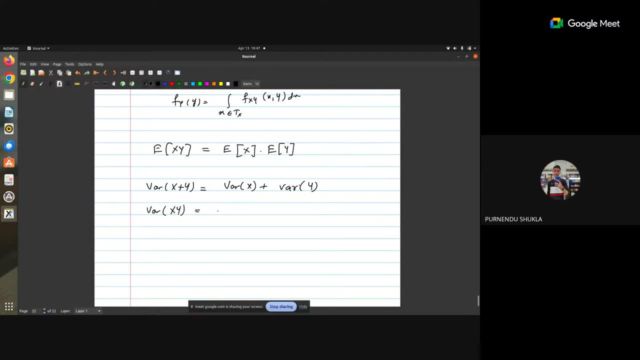 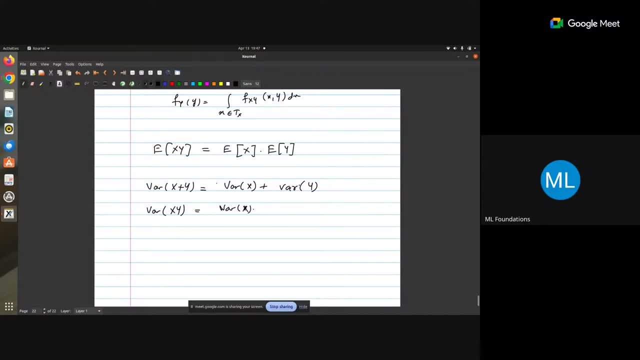 there is one more formula for variance, which is what this is not. maybe I'll just okay. how generally will be? okay, various formula is already there. you minute, I'll just find it, because here, in continuous case, what I have seen is tax to is like it depends on the distribution itself. what type of 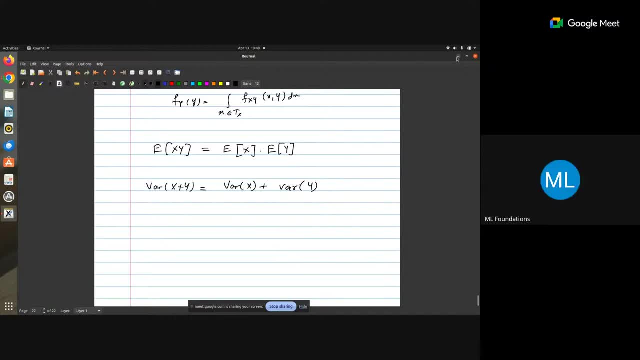 distribution: yeah, generally, no, no, generally. we need not to calculate variance in continuous because it's already given sometimes and but it's not a different. like, variance of X plus Y is for only for discrete case and in dip means only. this formula holds only for independence. random, no, no, no. yeah, this will okay. this. 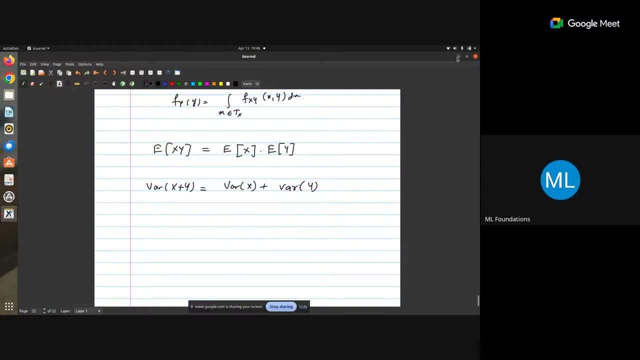 will work for independent. that is fine. but the thing is you can find out variance for continuous case also, because what is variance generally for any random variable? it's just difference from the mean. so E of X, yeah, so generally variance of X can be calculated project. so how you calibrate for this one. 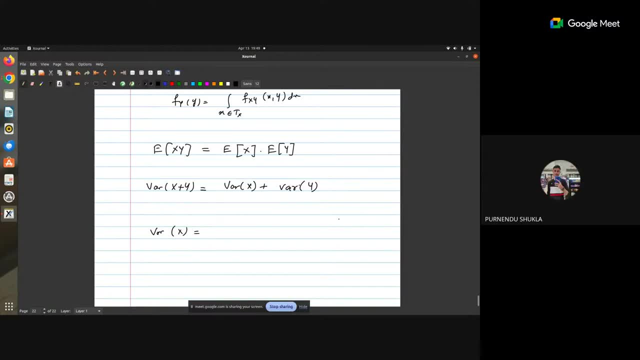 discrete case, this be used like E of X square. that is one formula. any other formula or maybe intuitively? how will you find out? are you status squared difference from the mean minus the data point, whole square divided by M, rather than that? I don't. okay. we have a formula actually. maybe just give them it. 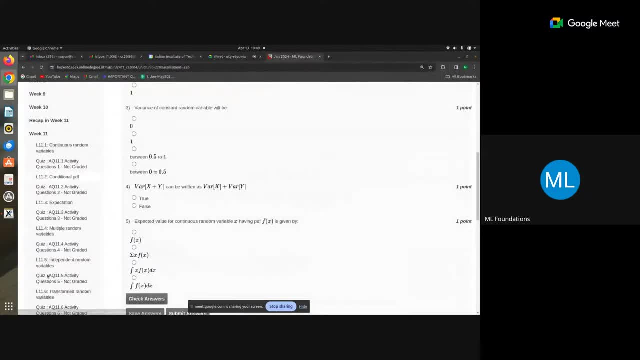 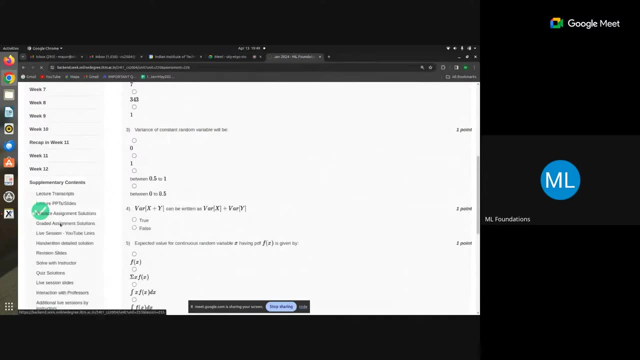 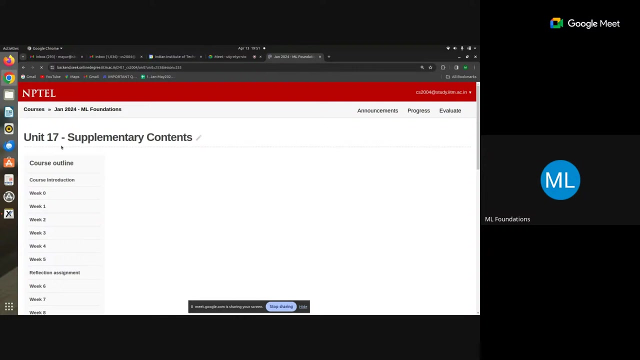 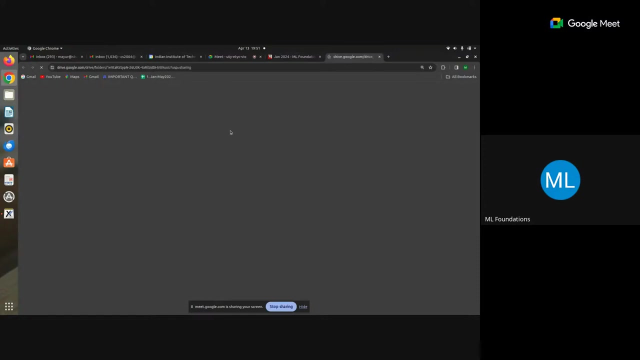 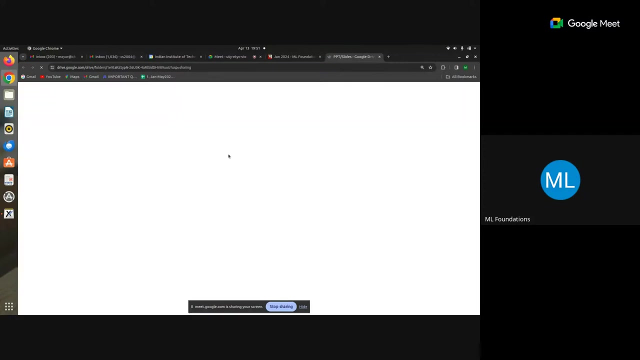 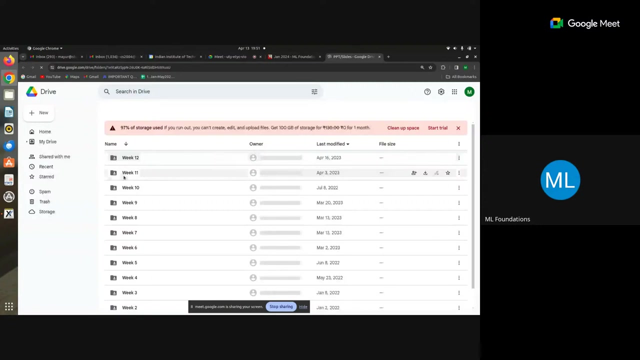 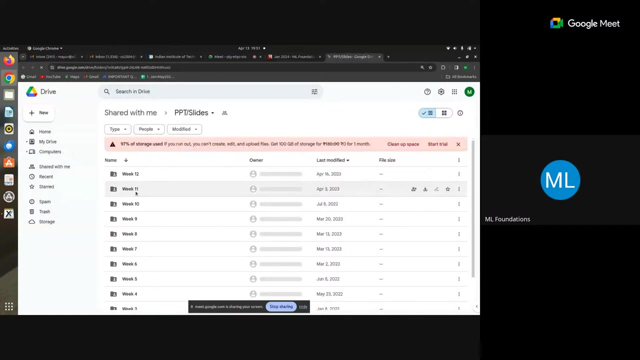 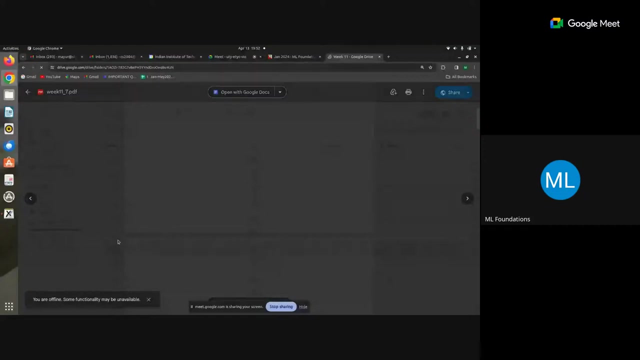 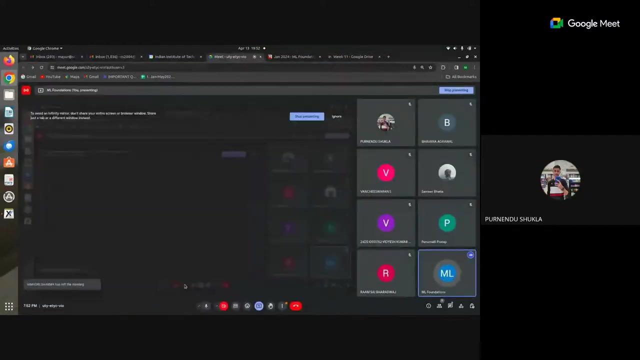 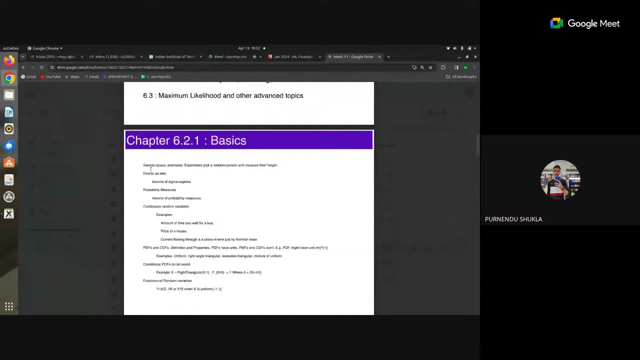 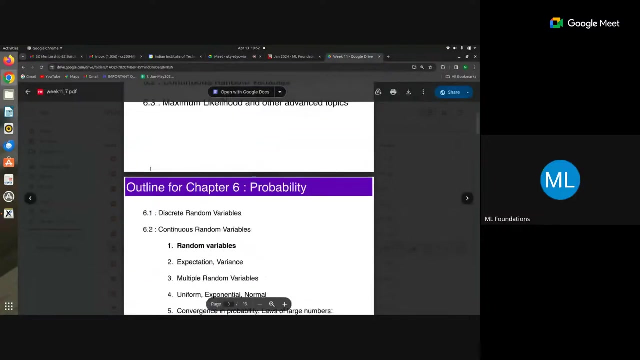 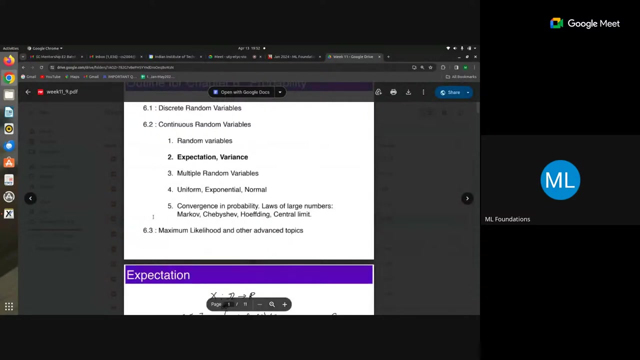 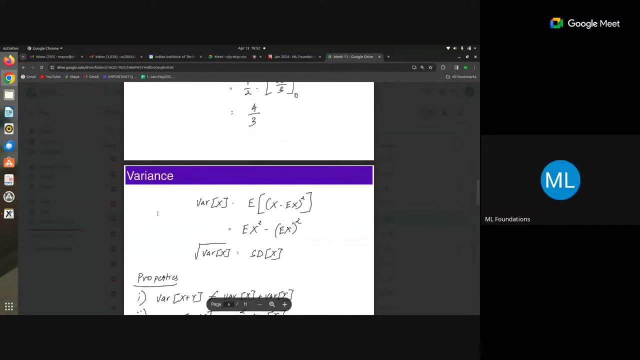 is a little bit before that we use this one. well, you, you, you, you you. Thank you very much. Thank you very much. Okay, so I think seven, eight Expectation is there. I agree, Variance for discrete case we have, but for continuous. 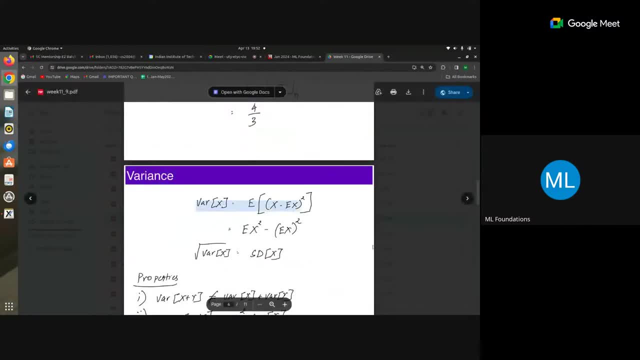 See, this is fun. Okay, so basically, what is it? Variance is generally like for normal data set. how you find out the variance? You just Subtract the mean from the variable- Whatever I said- And divide it by n, right? 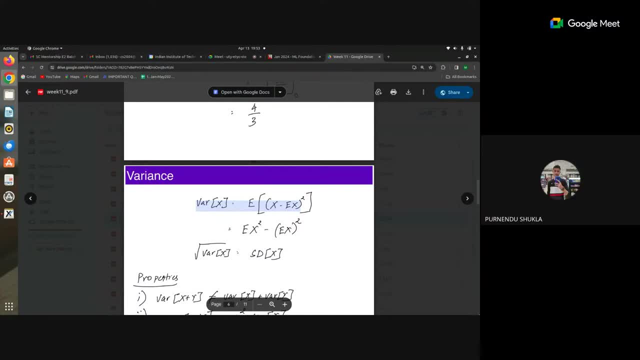 Dividing by n means what You're taking, the average of it, Average of it. So this is how you have to find the expectation of, And basically it is same again: Expectation of x to whole square. and you can solve: use the same method, right? 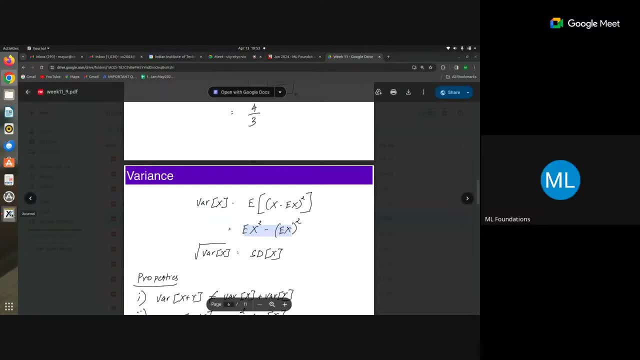 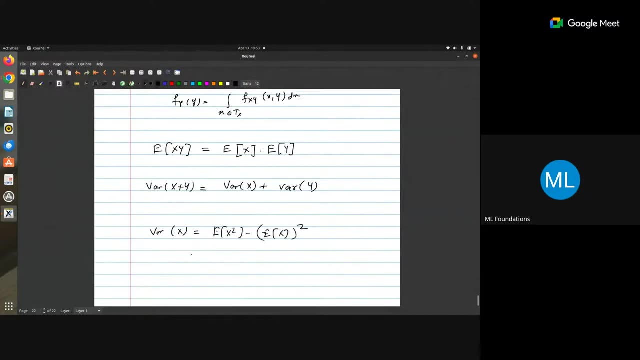 There In continuous case also Yes. So how will you find out there The expectation of x square minus Expectation of x to whole square. So how will you find x square, integrating x square? So over this range, right, Some range. 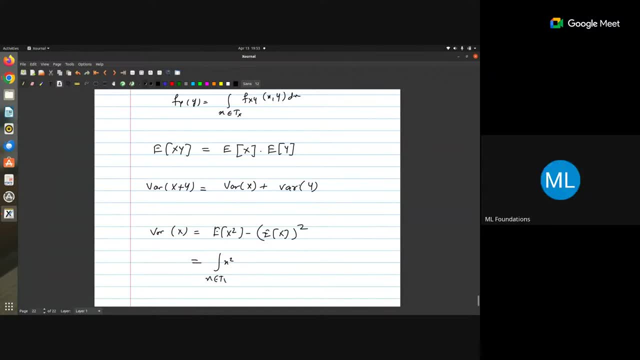 x, dx. Yeah, Let's say dx and x of x, dx, minus integrating x. Same thing. Okay, This square term where it will go then Here Here, Okay, Here Here, Let's see, And then we will make a square of it. no, 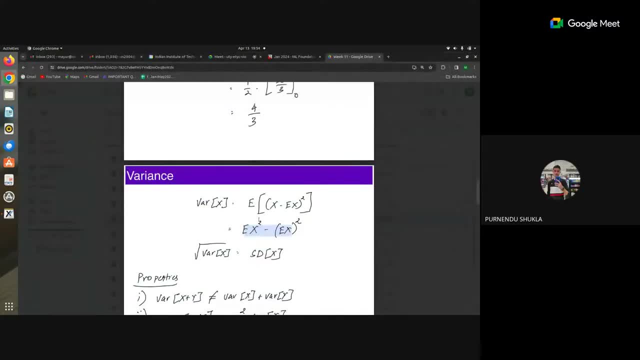 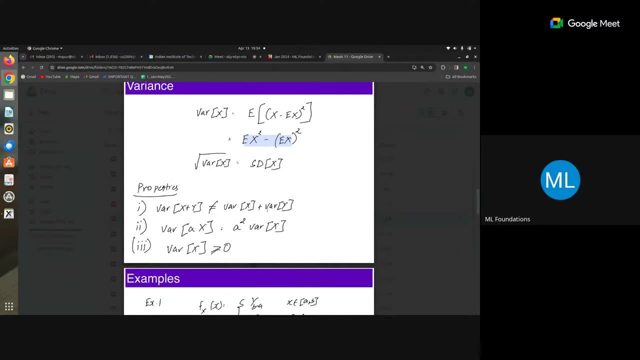 That's not a problem. After calculating that integration fact, then only I will do that square. Yes, Yes. So these are some properties of variance. Variance of x plus y is not equal to variance of x plus variance of y unless they are independent. 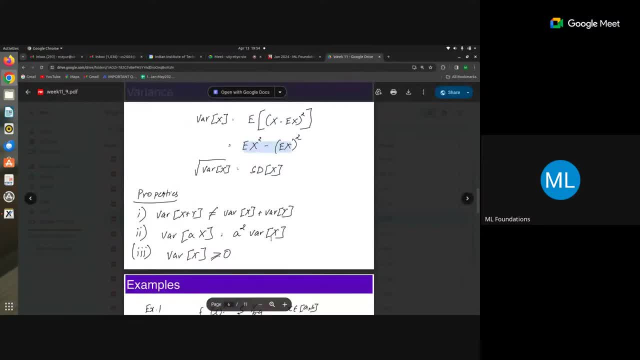 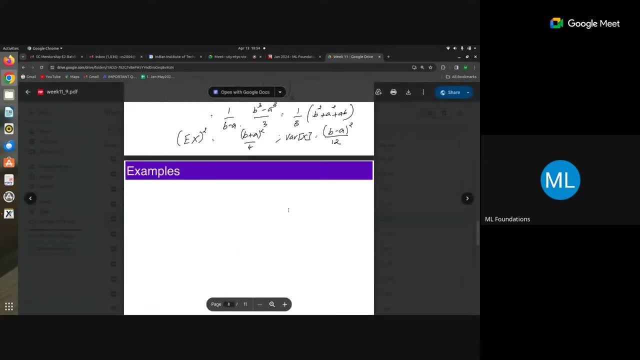 Okay, If they are independent, you can have this property as well with yourself. Variance of x equals to x, square into variance of x, So you have this uniform. Then you know. see, this condition was so. we have already found out here. okay, so a lot of problems are there in the lecture, so you can. 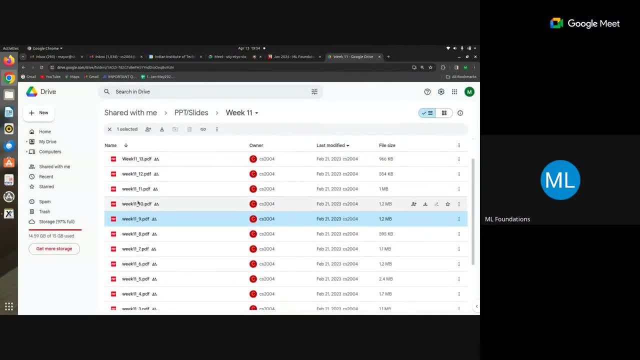 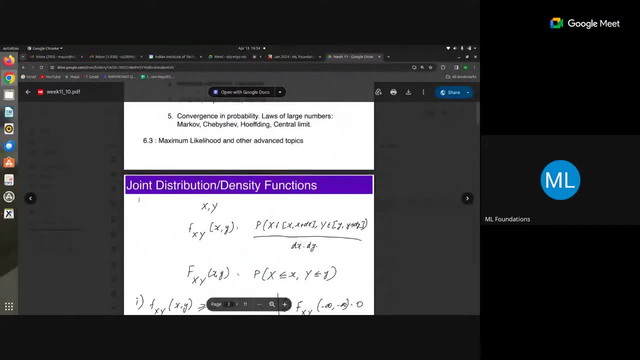 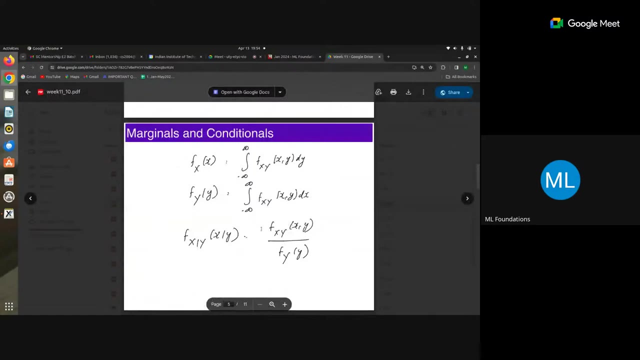 go through those problems. uh, maybe, if you want, at the end- once once i'll finish- transform random variables. if you want me to solve some problems, i'll solve it. okay, so these are joined in city functions. yeah, marginals and conditionals: okay, basically these are the formulas which i already 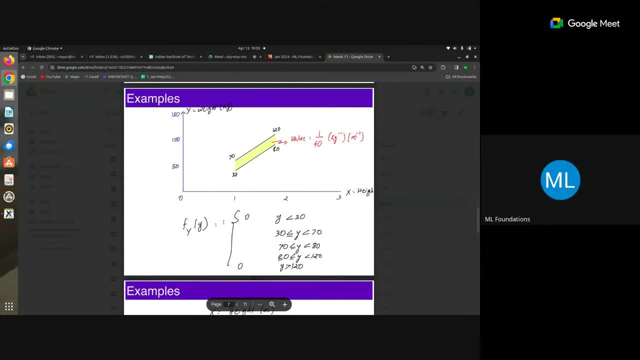 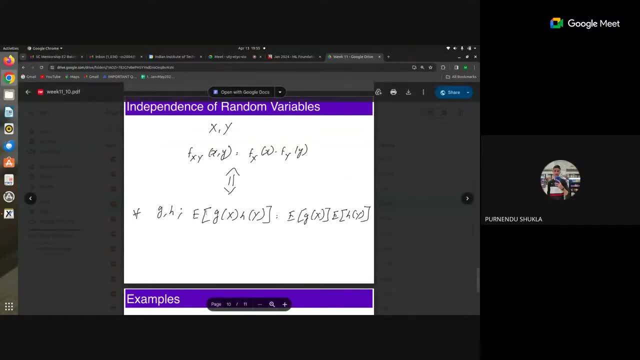 uh, which you are explaining. yeah, so this is independence. is what um, this one x of x into f, y of y joint is equal to product of marginals? yeah, and you can see that if they are independent, then expectation of this will be expectation of geofix into expectation of what's that is. 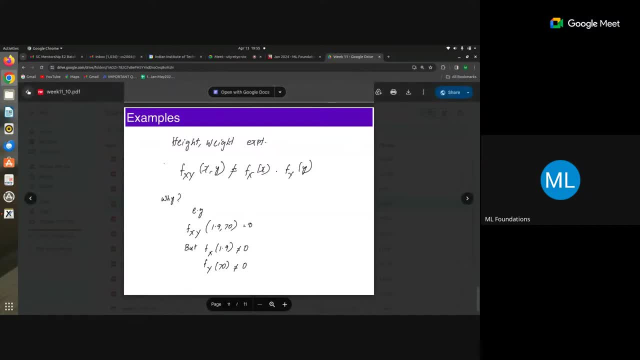 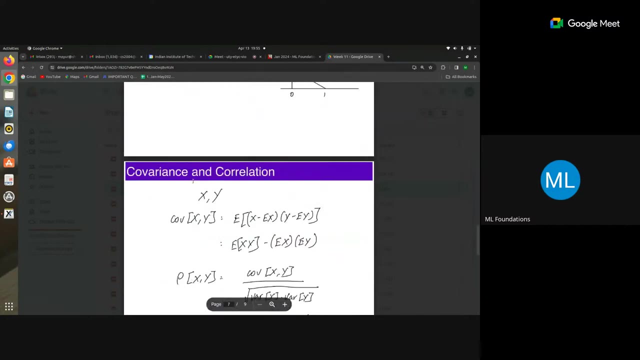 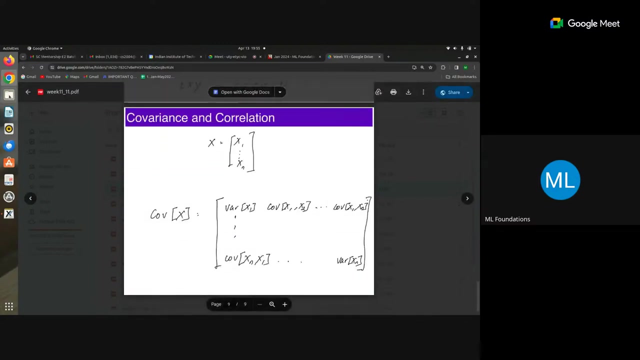 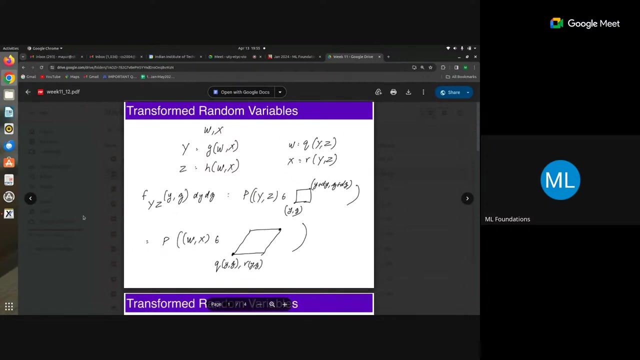 also possible thing. uh, okay, this convolution theorem. okay, this is some of independent random variables. maybe you guys can uh, this is this is the way. this is from where you are actually going into, you know, uh, the independence thing, sorry, the transform random variables. okay, maybe i'll just okay. first of all, i'll go through this part. okay, transform random variables and how. 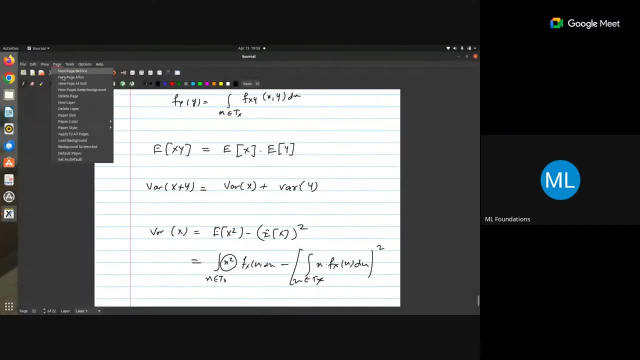 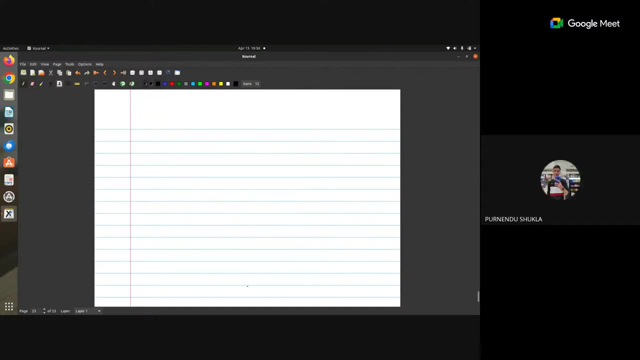 to solve this. so basically, you guys have got the idea right. what is the single random variable, how to find the expectation conditional distribution for that and after that, uh, going for the two right, two random variables. sir, can you show the previous slide? i'm just sorry. so previous slide can you show please? previous: you show variance of x. 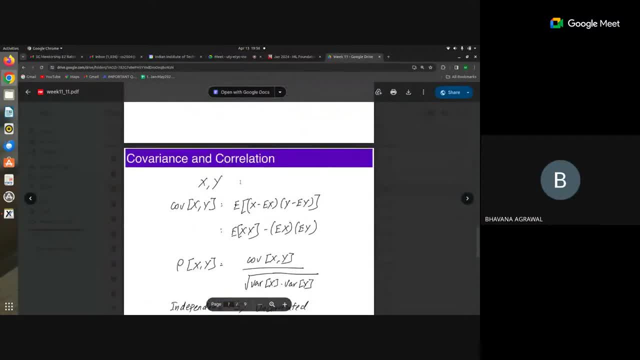 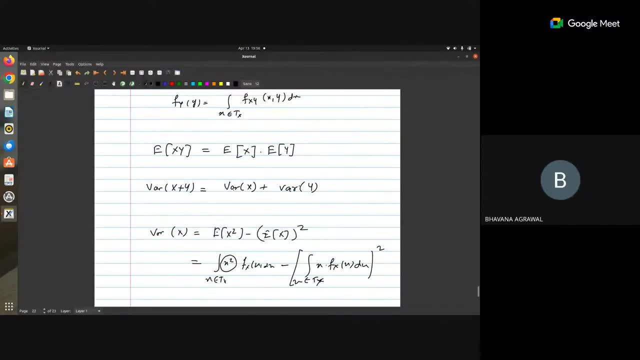 um, this one in it, your handwriting too. oh, my this part, sir. okay, we doing the holos card, okay, yeah, this is okay. right, this same thing. you don't have to do anything. the basic uh principles are applicable here also. okay, so transform random variables. uh, so we have seen, actually, uh previously how to transform. 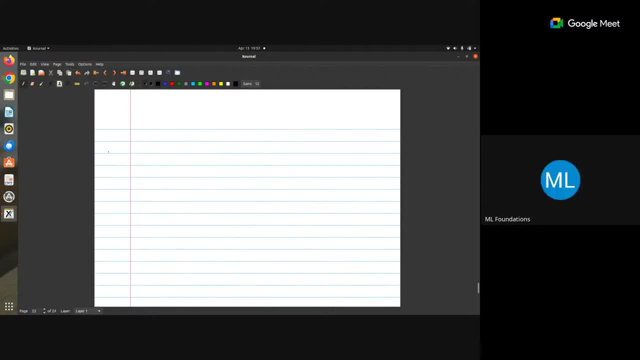 the single random variable site. yes, oh my gosh dude their random variables. they mean all random variables. yeah, that was good for us. what are the transformations we have seen previously, like linear transformation, for example. so i have told you in the previous lecture itself: we have seen: 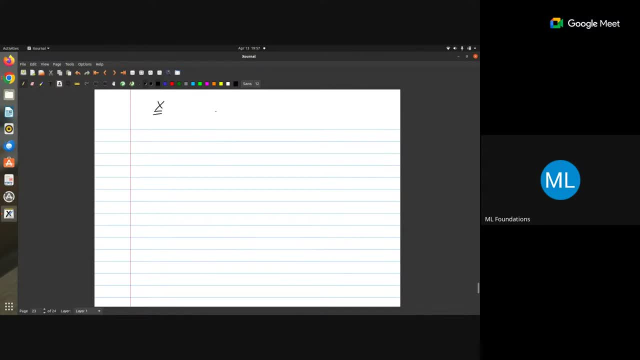 that, uh, if x is some random variable, the function of x, like 2x plus 3, is what. this is what. this is also a linear transformation, right, but this is for a single variable. let's say, you have, we. we already have seen this kind of uh questions previously also. like y equals to x, square is a. 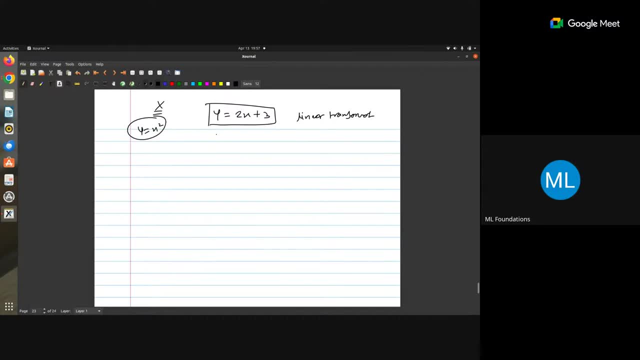 function of random variable, right. so y is basically what it's. it's a function of x, 2x plus 3 here. here it is: f of x is equals to x square, right. so these are the functions of random, but these are the transformations also, right. so x was actually basically is having some distribution. 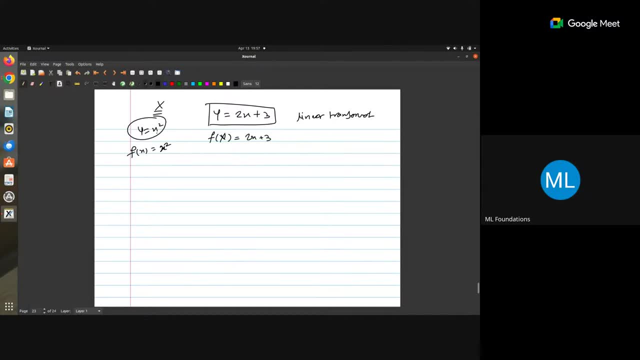 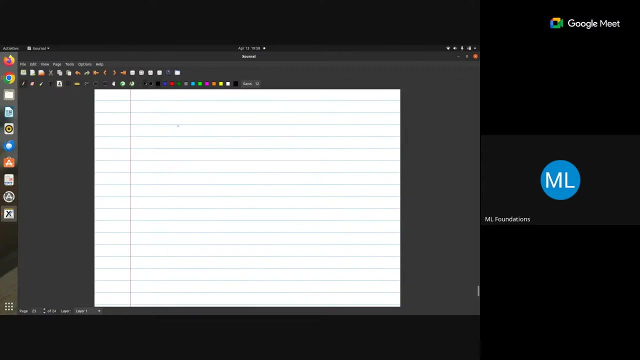 and if i transform it to some other variable by applying a function over it, what i'll get? i'll get some other distribution right, some other probability distribution. similarly, if i wanted to transform two random variables, if i wanted to see the transformations of two random variables, how? 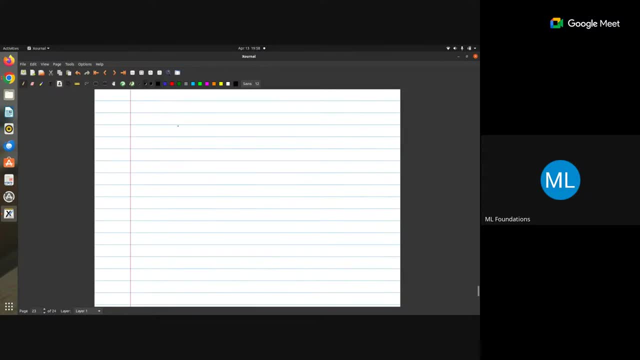 will i do that. that is what uh the. so not every uh two like each one. every two random variables can be. uh can have the transformations right. so let's say we have two random variables, x and y, with joint probability or joint uh pdf. as let's say, fxy of x, comma, y. right, this is okay, you have two random variables, xy. 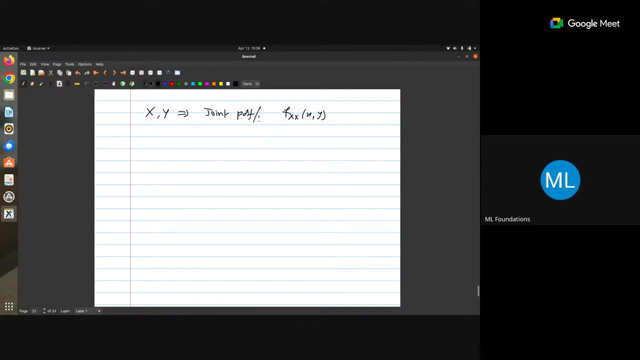 with joint pdfs, or pmf pdf, or let's say, pmf fx, fxy, of xy is okay. now, uh, let us define, uh, the transformations. the transformations are basically, let's say, the functions of, uh, two random variables. okay, let's, let's say, uh, let's okay. 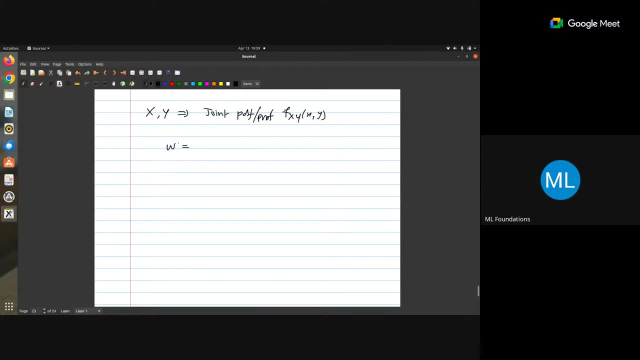 then let's say: i have defined some new random variable, w, which is a function of. let's say this. i'll write this as: let's say r, r, of suppose, x, comma, y, okay, um, I have defined some new random variable, w, which is a function of: 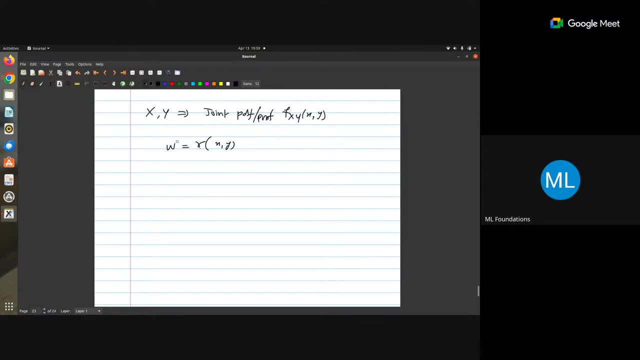 let's say r, r, of suppose, x, comma, y, okay. and let's say we have uh, okay, no, no, sorry, I'm not sure. uh, just in case. okay, fine. so let's say x, y and y are there with joint pdfs and let's say x and y are there with 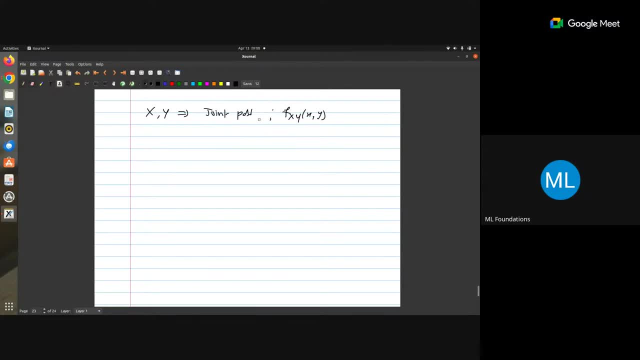 joint pdfs. and let's say x and y are there with joint pdfs. and let's say x and y are there with pdf or pmfs. let's say uh, i'll think about this as pdf currently. so let's say pdf, or uh, pdf of x and y is given as f, x, of fxy, of xy. 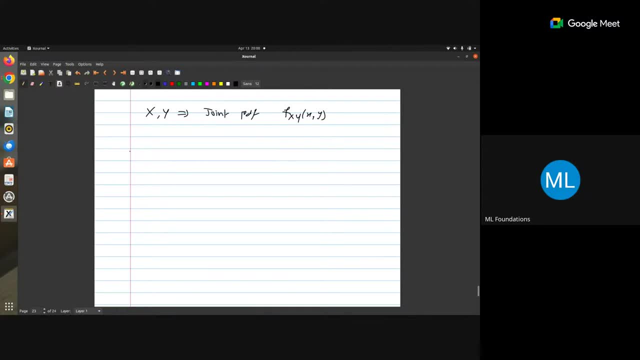 now I defined two other random variables which can be. so, let's say, x is a function of w and z, so w and z are also two different random variables. okay, w and z are, uh, two different random variables, random variables, but x is a function of this two. 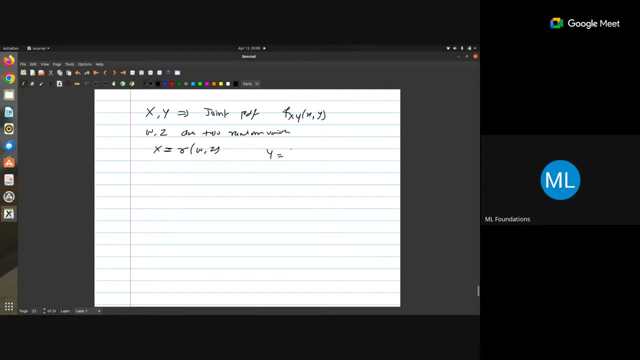 w and z and y is also a function of some other function of, let us say, g of w comma z right now. this is, or maybe I will say it is, h of w comma z and this is g of w comma z right now. I wanted to find 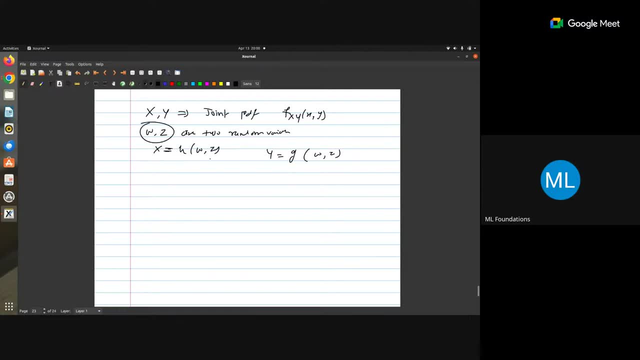 the joint density of this. okay, so let us say I will say this joint density of this. I will represent, as I suppose, r sir, what is h of w comma z? it is a function of function. it is a function basically. x is a function of w comma z. 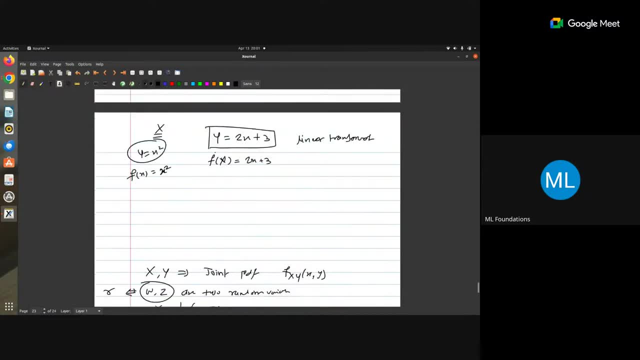 so here you can see right in this example, you see, when y is equals to 2x plus 3, here, basically, f of y is what it is a function of. sorry f of y, let us say, y is what y is basically, is a function of x. 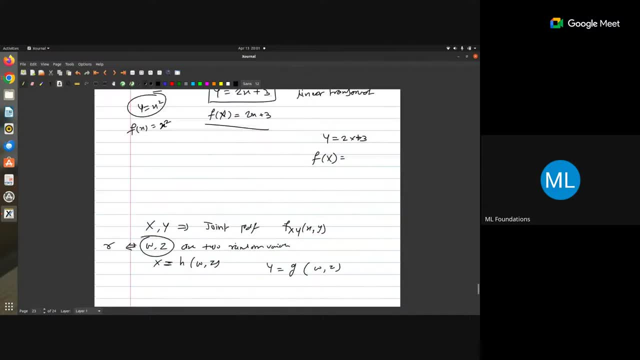 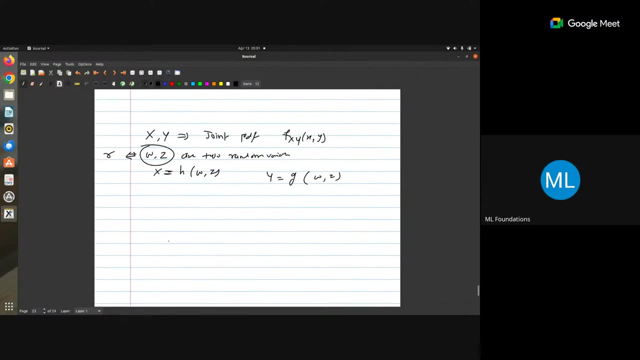 right here. what I am saying is: x is a function of this. two random variables, w, comma z. I will tell you. okay, I will give you an example. you will be able to appreciate it much better. so this is a general definition I am just talking about. if I wanted to find the joint. 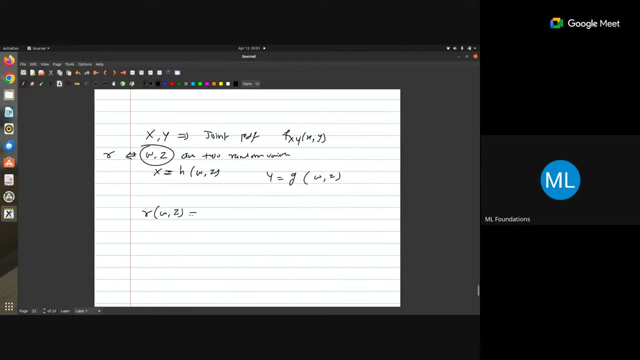 density of this w, comma z. how will I find it f of? let us say f of. so this is f x, y of x, right? so let us say this is f x y. I wanted to find this w and z in terms of joint pdf of x and y. 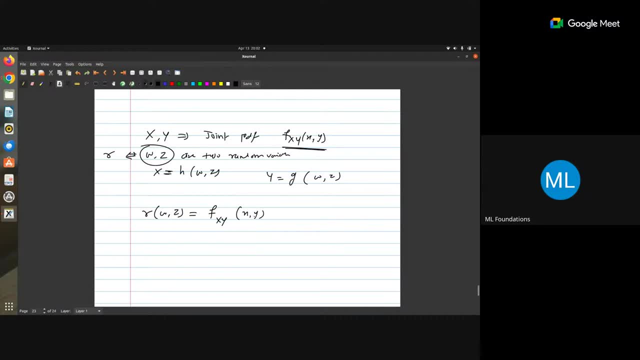 okay, so f, x, y of x, comma y, I have to find. so I have to write this function of joint density of w and z in terms of f, x of y. so how will I find it out? is instead of x. I will put what h, h of. 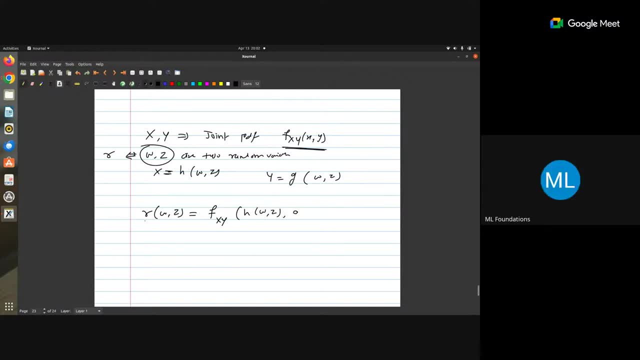 w comma z, and instead of small y I will write g of w comma z, right and into jacobian. okay, so this, j is a jacobian, jacobian and j is basically, and this, this is what absolute value of jacobian. so j is basically del r. 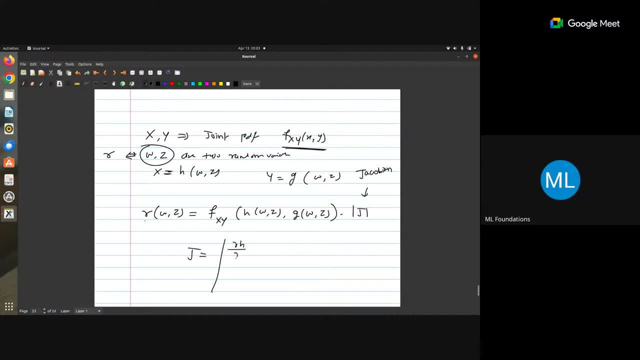 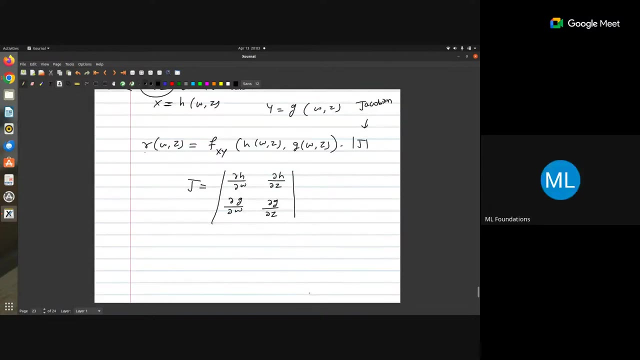 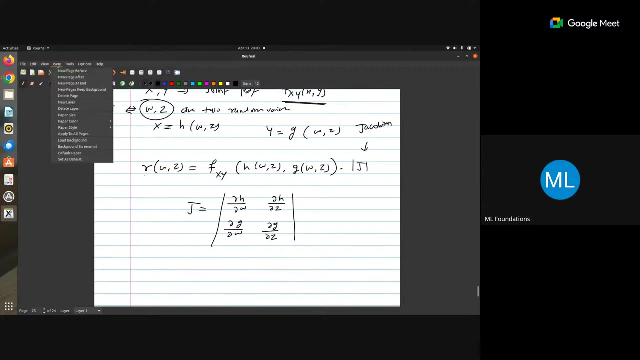 or del h of del w, del h of del z, del g of del w, del g of del z. okay, it is a determinant, determinant of these values, okay, so I will just give you an example and we will try to see that, and after that you will be able to see. 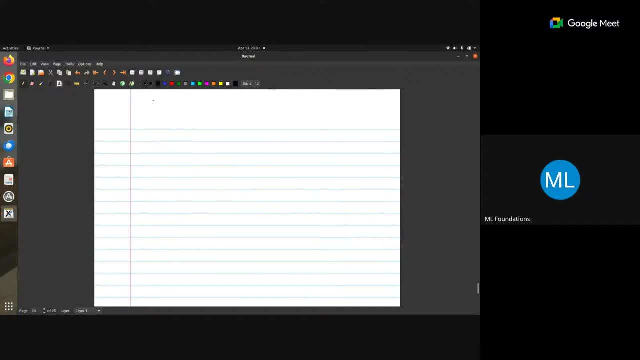 you know, may be much better you will understand. so suppose there are two random variables, x and y, with joint density function f, x, y as 1 by 6. ok, so it is a constant joint density function where x is from 0 to 2 and 1 is from 0 to 2.. 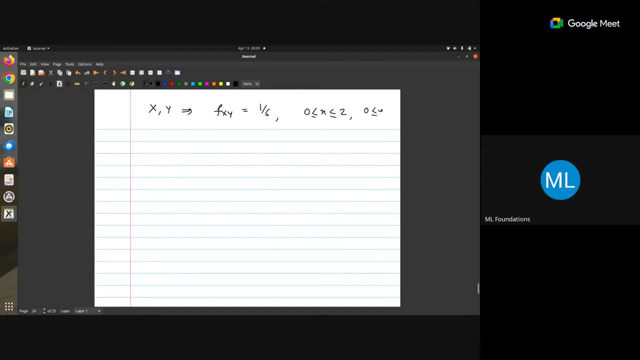 and 1 is from 0 to 2.. y is from 0 to 3, ok, And we need to findjoint joint pdf of w and z, right and where. what is w here? w here is, let us say, x plus 2y, ok, and z is suppose it is 2x plus y. ok, So are. 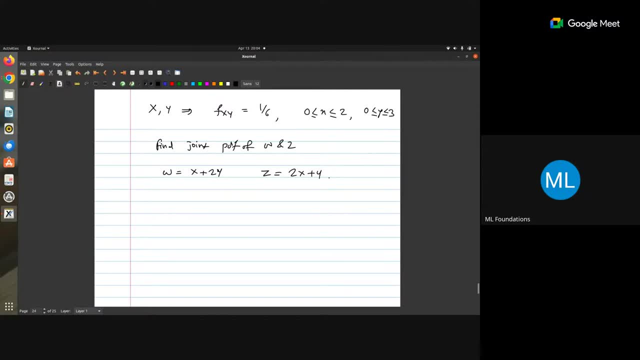 this: w and z are invertible, Invertible in the sense. can we write x in terms of w and z? Yes, sir, we can. Yes, right, So how willyou do that? let us say: this is function 1 and this is function 2. ok, ok, So. 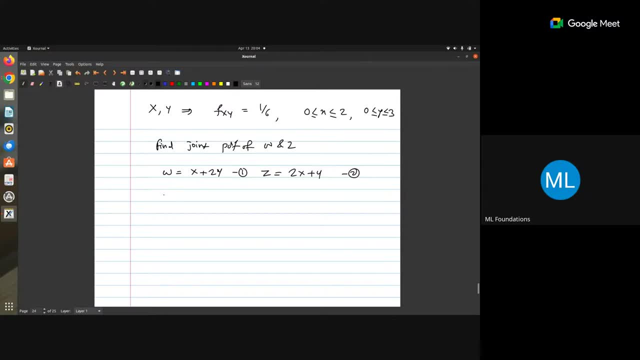 what I, what I should do to find x. I will multiply2 the function, the equation 2, with 2 and subtract it from or subtract equation 1, right, So we can even divide equation 1 by 2.. Yeah, So there are ways. 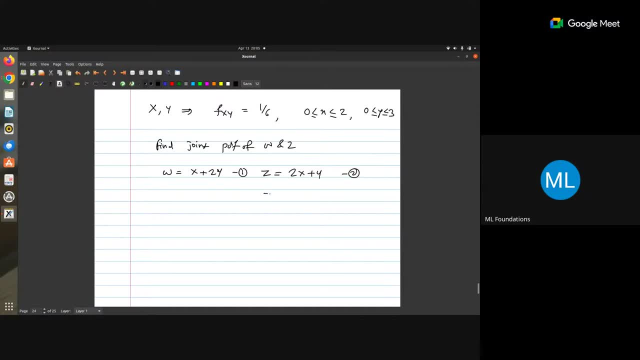 So let us say I will. I will just multiply this equation 2 with 2 right, So z. so this will become 2, z equals to 4x plus 2y, 2y. I will subtract equation 1.. 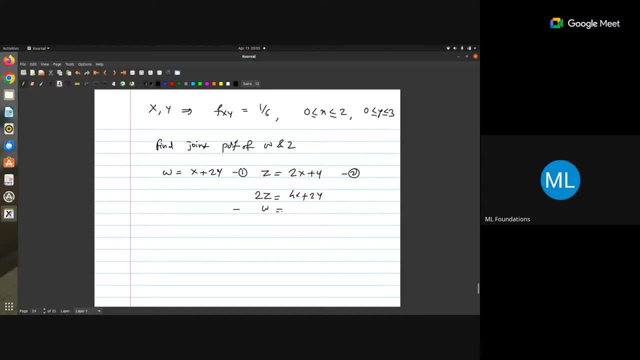 2y. This w equals to x plus 2y 2y. So when I subtract, that means this becomes minus, this becomes minus, this becomes minus right. So this will be 2y 2y. 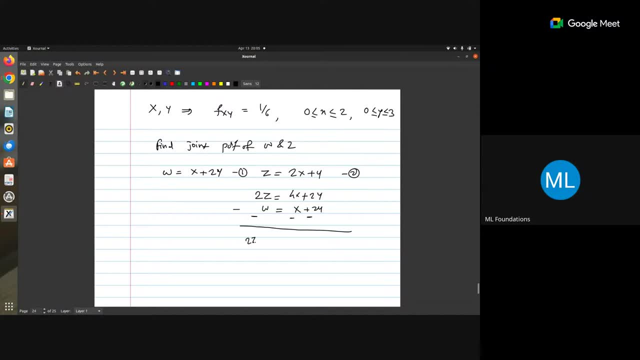 2y, 2y, 2z, So this will be 2z minus w equals to 3x, 3x, So x will become 2 z minus w upon 3.. Is it ok? ok? 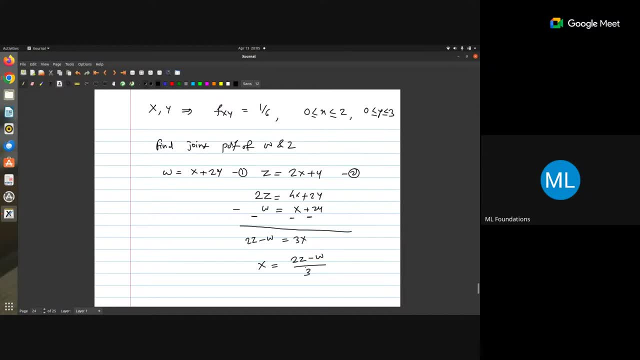 Ok. Similarly, if I wanted to find y from this, So y will be equals to To find y- what should I do? No, let us say I have to. let us see if I can find y from this. Yes, sir, Ok, I will. 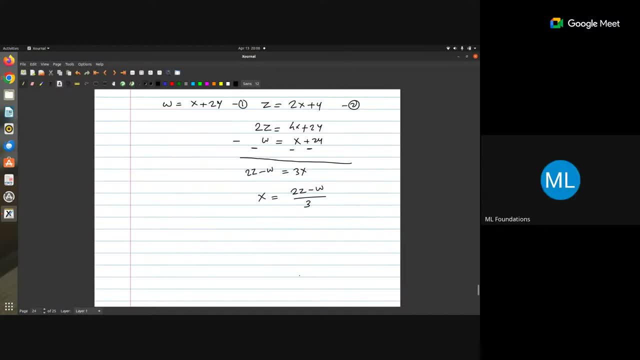 So what should I do now? this is: x is equal to 0.. Yes, sir, So that is what I said earlier, right? Yes, sir, Let us say I will subtract this: 2y, 2y, 2y. 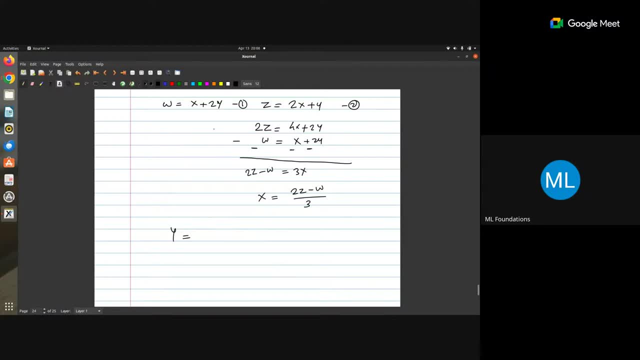 2y 2y, 2y, 2y, 3y. No, I think I can. I have to. so I'll multiply this equation by 2, so this becomes 2 W equals to 2 X 2 plus plus 4 Y, and I'll subtract Z, so Z equals 2, 2 X 2 X plus Y plus 4 Y, so this: 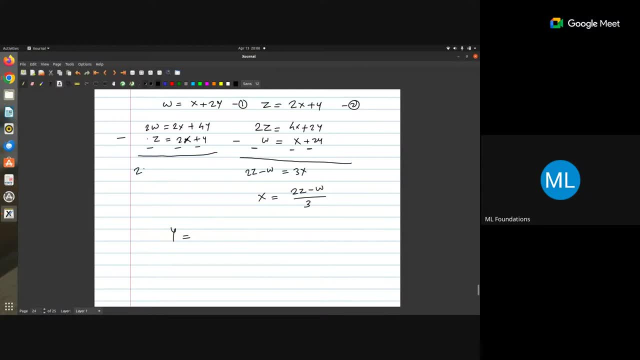 this will become minus here. this is 2 Z. sorry, 2 W minus Z equals to 3 Y, so Y will become equals to 2 W minus Z divided by 3, 3 is ok. is there any issues? no, sir, okay, now I okay. so consider this has some value of. 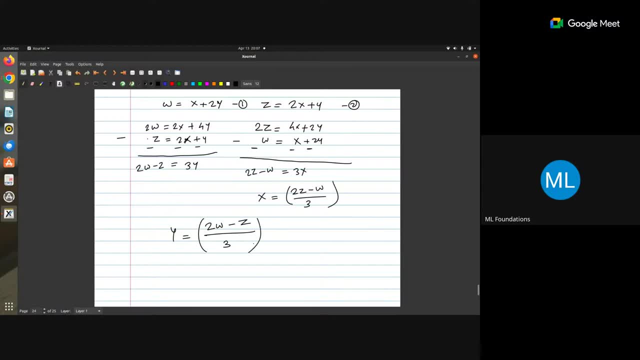 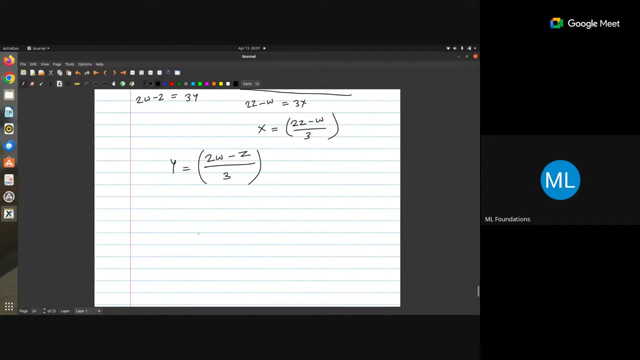 X, right, and this has some value of Y, right. these are, these are some values, right? okay, now to find the joint pdf of w and z, what i have to do is i have to find the jacobian first. okay, so what is the jacobian? so i have to, uh, so let's say: this is what this is, function, our function, h. 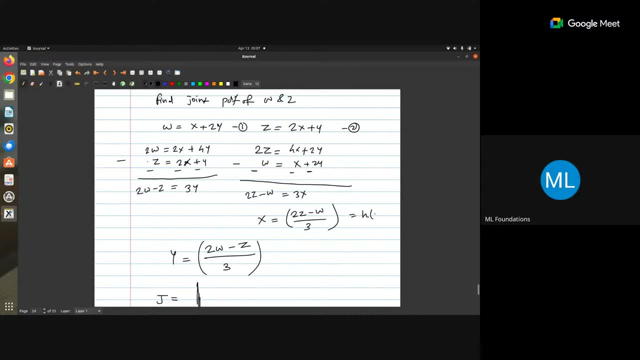 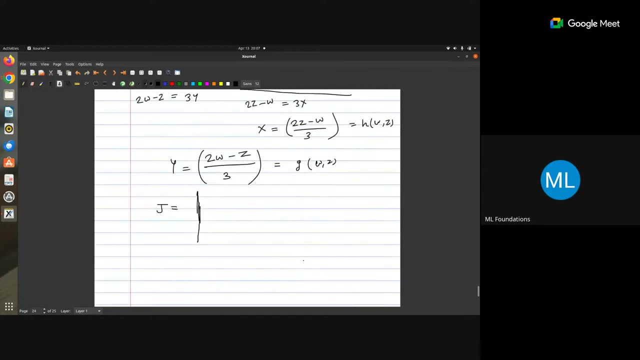 okay, let's say this is h of w comma z and this is g of w comma z. what i have to do here, i have to differentiate with respect to w, with respect to z, here, uh, del g of del w, del g of z, right, and what i, what i'll get here. 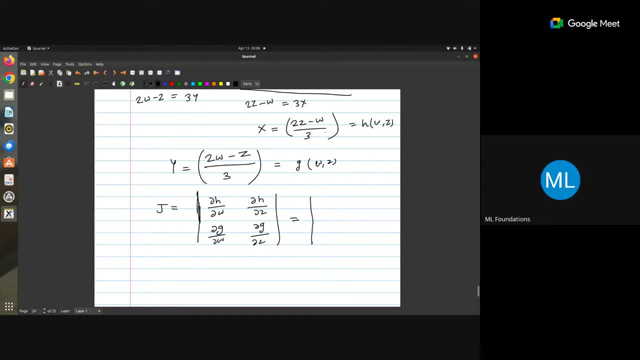 is: this is h of w comma z and this is h of w comma z and this is h of w comma z. and this is: are those partial derivatives? yes, partial derivatives. so what is uh what i'll get here if i differentiate this with w. basically, this is what uh here. okay, so i'll get uh, we can get it. 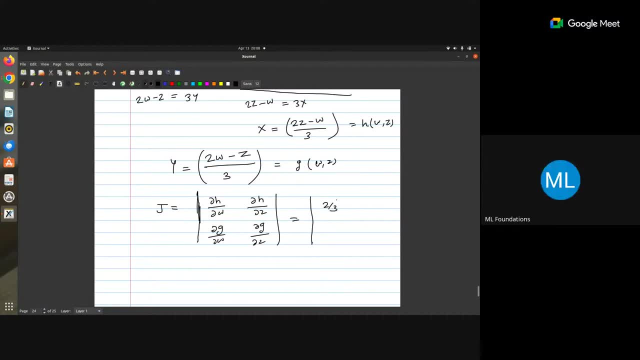 like three minus two. here it is two by three. no, sorry, minus one by three, you are. uh, this is h of w z, right? so with respect to w, if i differentiate it, i'll get minus one by three del h by del z is what. two by three, two by three here. del g of d w is what. 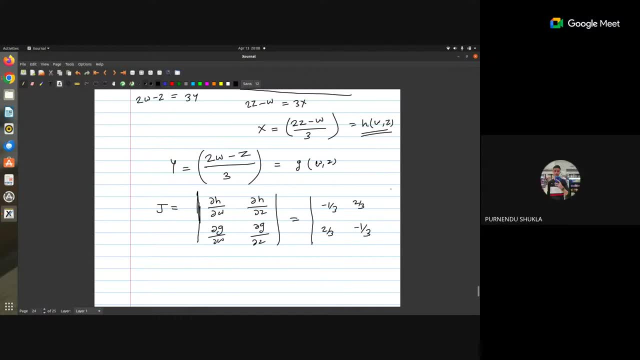 two by three, two by three, and here it is one minus one by three. so determinant of this will give me a jacobian. so this is nothing but one by nine minus four by nine, which is minus three by nine minus one by three. okay, but uh, when i wanted to transform, i have to take this: 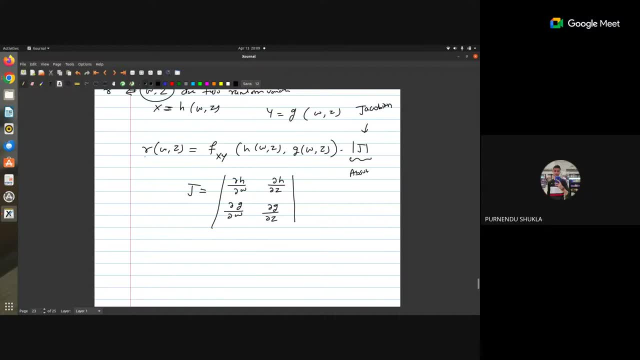 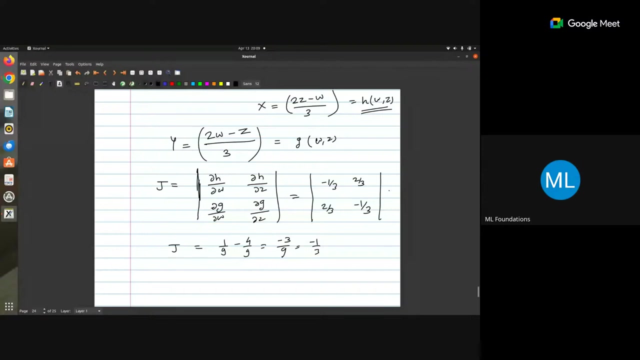 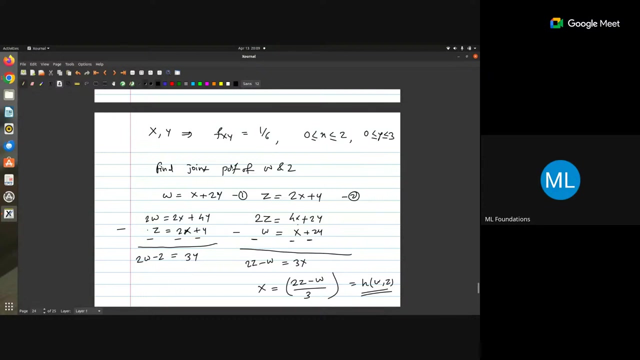 absolute value. okay is, yeah, is it? is it okay now? yes, sir, okay, so, uh, actually, these are in multiple functions. you have to understand, like how we are going to understand, like how we are going to understand, like how we are going to to invert the function. you just uh see any lecture on invertible functions. okay, 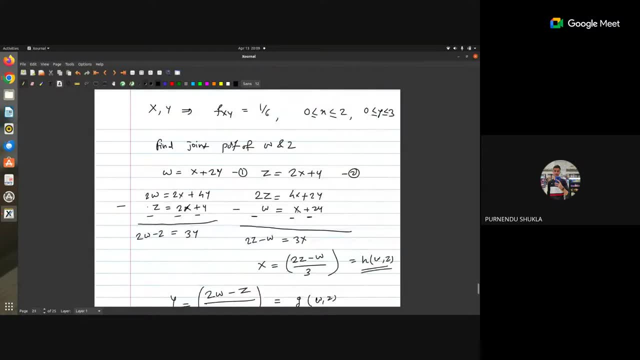 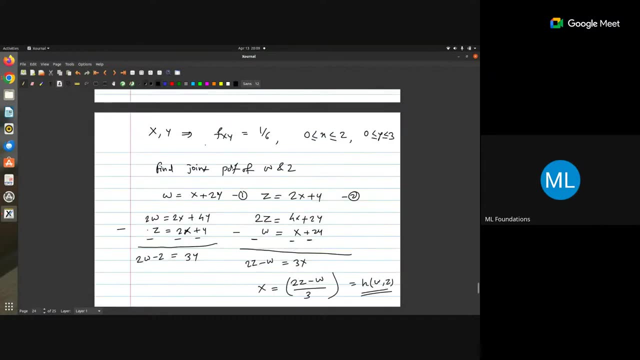 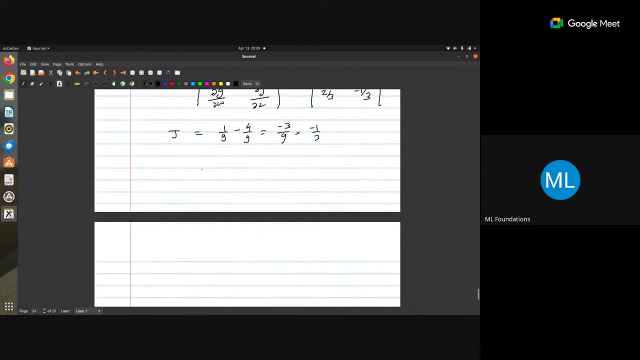 sir, is it necessary that, like calculation for x and y is necessary? yes, yes, so yeah, if they are, if they are not invertible, we cannot uh get in terms of you know, w and z, then determinant will be zero. yeah, so if, if the determinant is zero, we are not able to uh go back to, you know that. 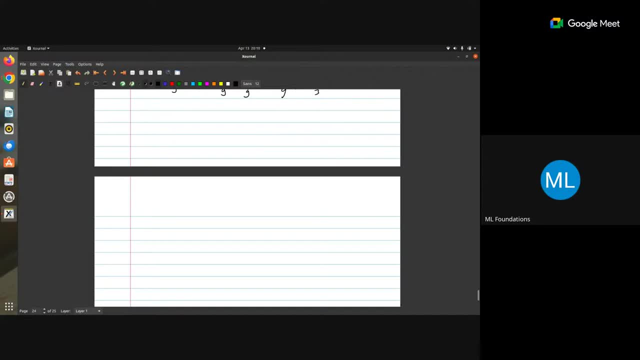 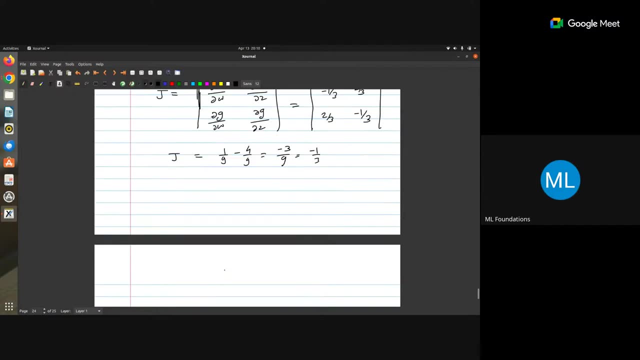 means i am not able to represent x in terms of w and z. if i am not able to do that, that means it's not invertible. okay, so now i wanted. okay, so the joint density i wanted to find right. so now, f of so i wanted to find joint density of w- z in terms of. 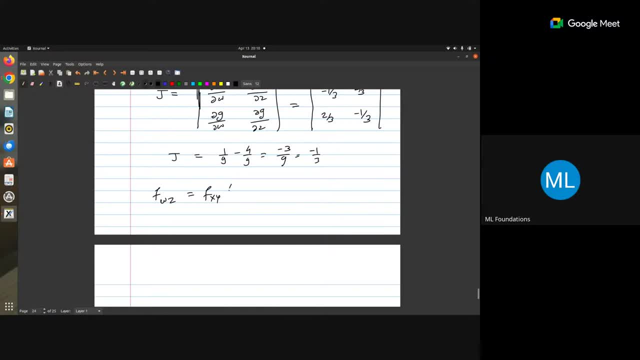 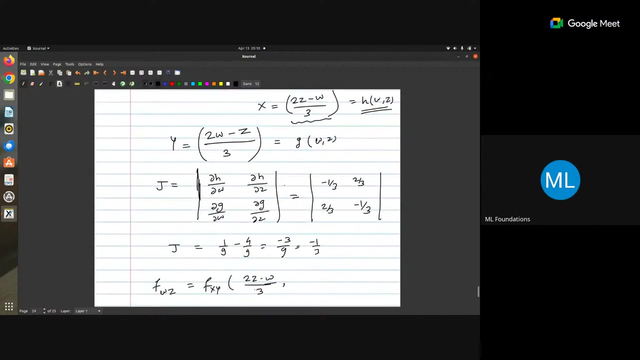 f, x, y, because they are invertible. i can do it. so instead of x, i'll do what here h of. so what is it? this one, right? so i'll write 2 z minus 3 by, sorry, 2 z minus w by 3 comma g of w, z is. 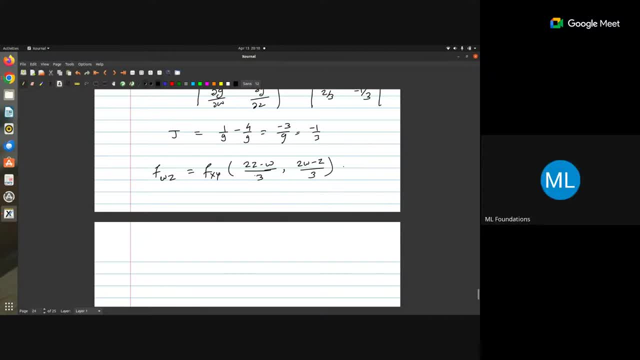 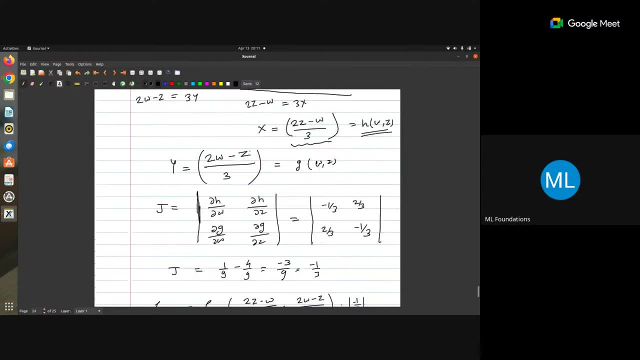 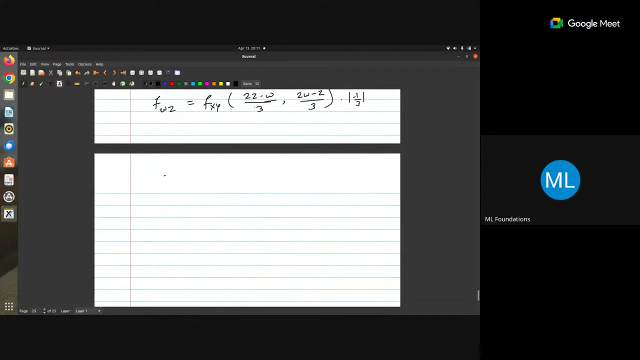 2 w minus z, minus z, upon 3, into mod of jacobian, which is minus 1 by 3. but what is f x y, f x y of x y by 6, sir? so f w z will become 1 by 6 into 1 by 3, which is 1 by 18.. okay, so, uh, what? now? the the important. 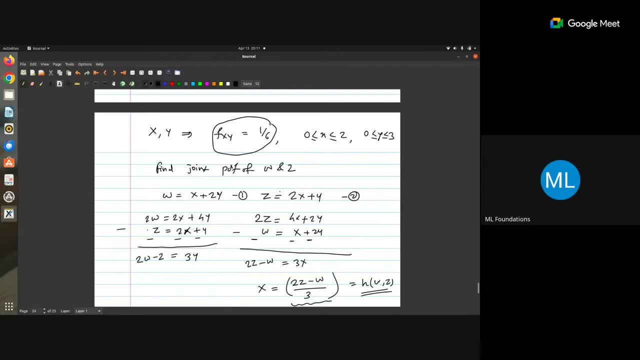 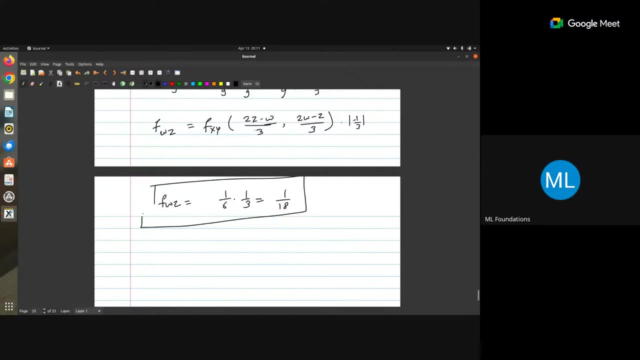 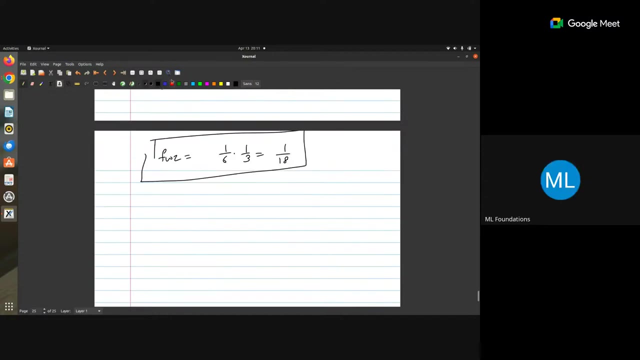 part is: we'll visualize this one. okay, we'll. we'll try to visualize how the support has changed. so this is actually the joint density of w and z, and we are able to find out. uh, you mean both openings together, correct, correct? that is what we have learned today. right, so now, uh, so we also multiply it, or we minus. 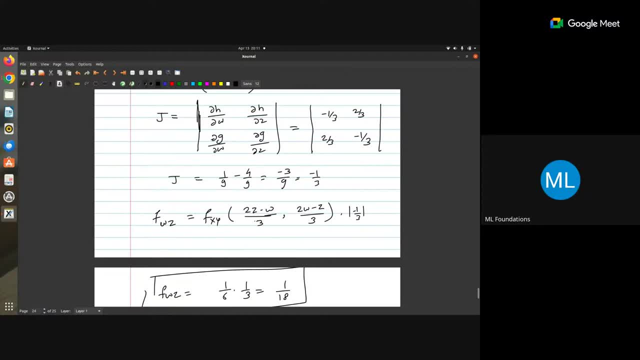 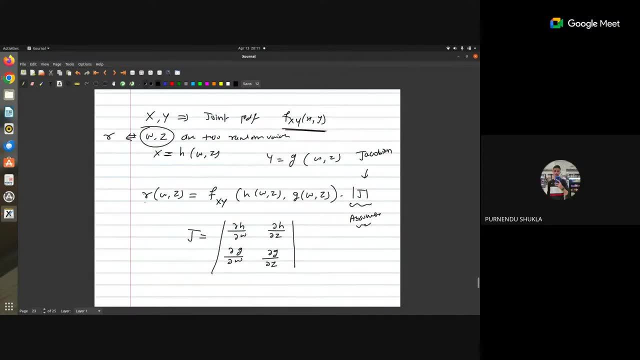 multiply, multiply right into jacobian, right? that is the definition here. uh, i have written here, right, mm-hmm. okay, so basically, in means what i understood from this is like you have some random variable as a function of some, uh, some other values, yes, and then you want to find: 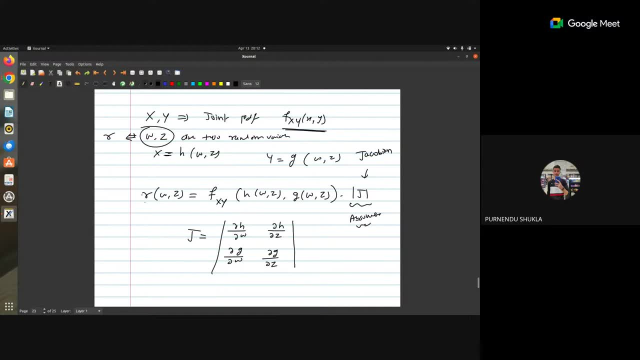 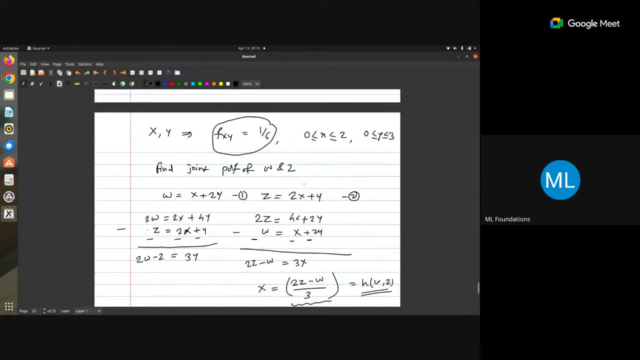 the joint probability for this. so this is the steps that we need to follow. yeah, so here what happens is x is actually a function of w and z, which are two other uh, random variables. y is also a function of two random variables, w and z. okay, basically, and that is what here happened, right? so actually, x is uh, because i can to write x in. 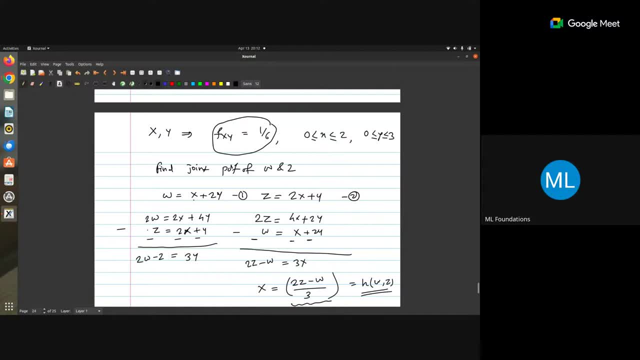 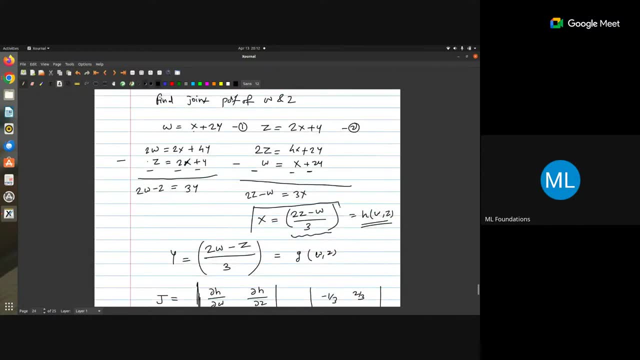 terms of w and uh, y here right, or w and z here right, huh, so uh, because you see, x is a function of this w and z. y is a function of w and z and i need to find what joint density of w and z, because this w and z are also two different random variables. basically, x and y are the 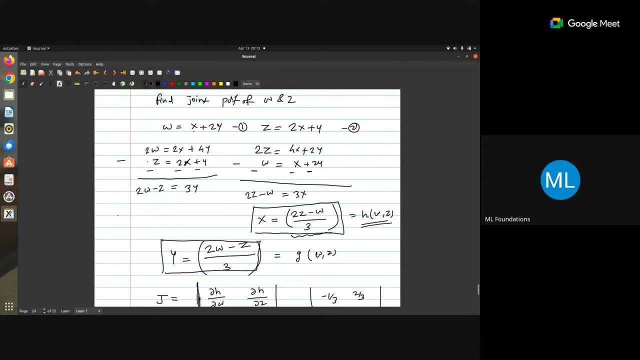 random variables which are dependent on w and z, w and z. okay, but i, i know the joint density of x and y. okay, but i wanted to find the joint density of what- w and z, w and z- and this is the procedure to find out. okay, so we'll see that, uh, how the support has changed. so what is the? 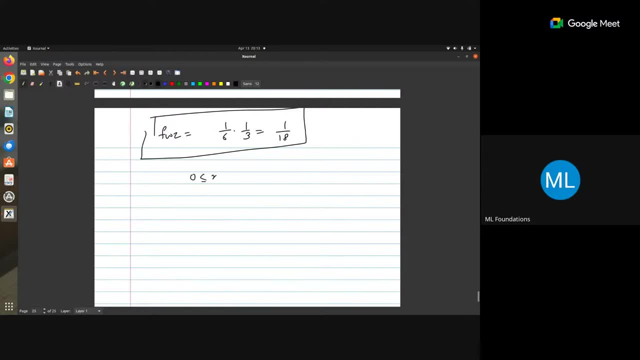 support. basically for x it was from 0 to 2 and y was having 0 to 3. so if i draw the support for x and y, how this will look? so x will go from, let's say, 0 to 2 and y will go from 0 to 3. so 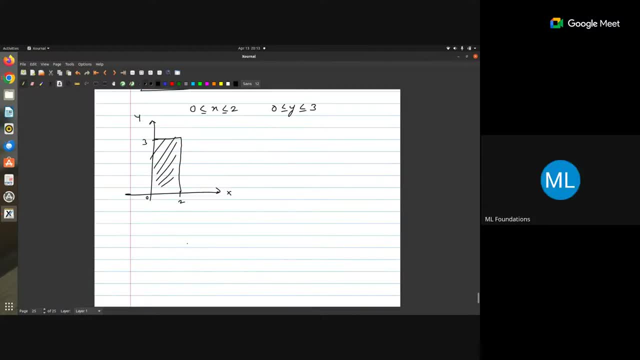 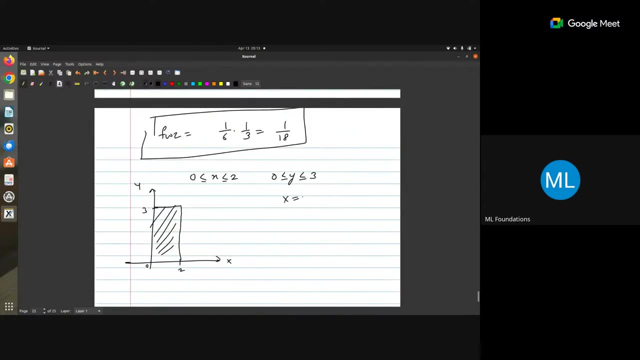 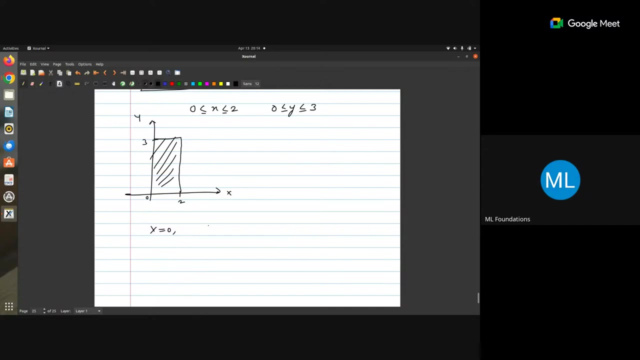 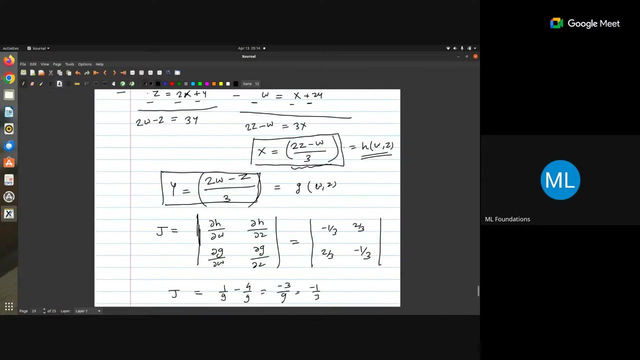 this will become some rectangular box right now. i wanted to check for y, w and z. so how to find the support now? so when x is equal to 0, i'll write it here so that we can see. so when x is equal to 0, uh, what does it mean? x equals to 0. that means 2z minus w by 3 equals. 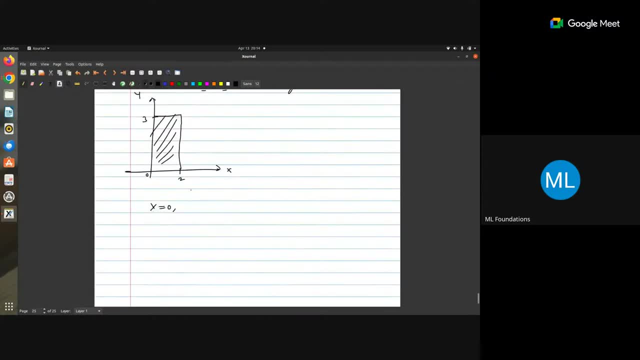 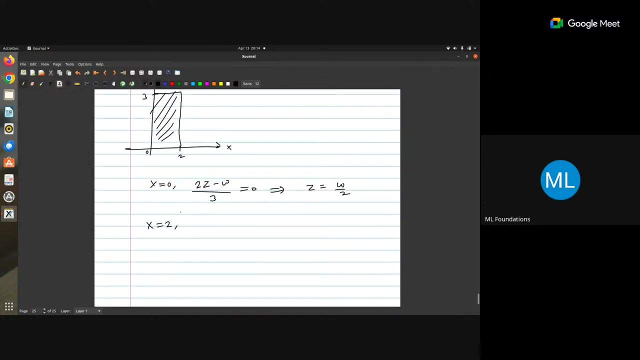 to 0, right? okay, so this is 2z minus w. divided by 3 is equal to 0. that gives me: uh, so let's say z equals to w by 2, okay, when x is equals to 2, because the support is going from 0 to 2, right? so that's why i'm just using the corner cases. that means 2z minus w. 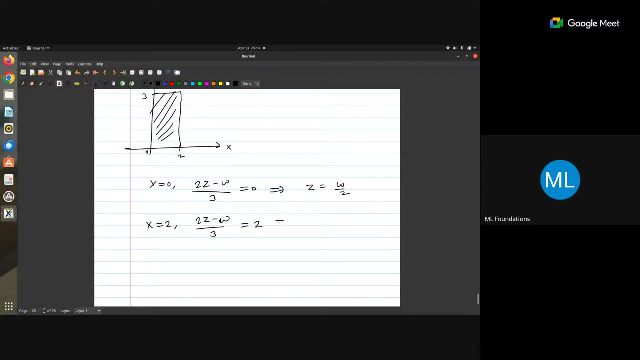 by 3 is equals to 2. that gives me what uh z equals to 6, z equals to uh 6. my 6 plus w by 2, w by 2, plus w by 2 plus into two is six, and then uh w plus this negative sign will go there. so six plus w by two, we will. 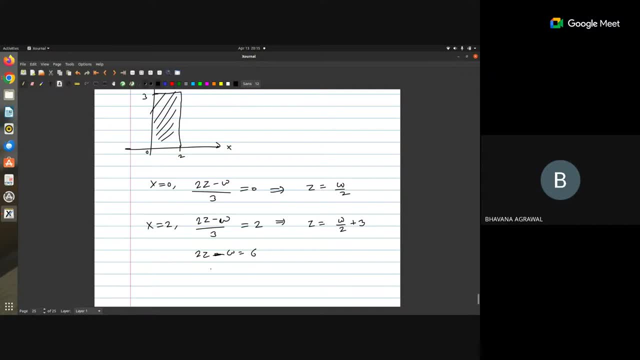 get now. this is six divided six by two to get three now. oh okay, so z equals two w by two plus correct, only right? oh okay, so z equals two w by two plus correct, only right? oh okay, so z equals two w by two plus correct, only right, yes, sir. 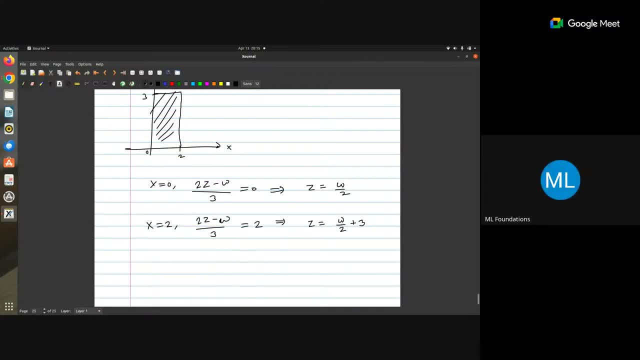 yes, sir, yes, sir, right, right, right is okay, right. yes, sir, is okay, right. yes, sir, is okay, right, yes, sir, okay. and when i have y okay, and when i have y okay, and when i have y, i equals to zero. y equals to zero means i equals to zero. y equals to zero means. 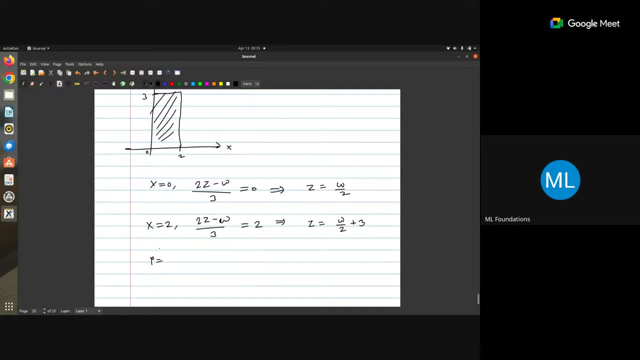 i equals to zero. y. equals to zero means what, what? what this? this problem is this. this problem is this. this problem is: w minus z by three: equals w minus z by three. equals w minus z by three. equals two minus z. two minus z by three. two minus z by three. 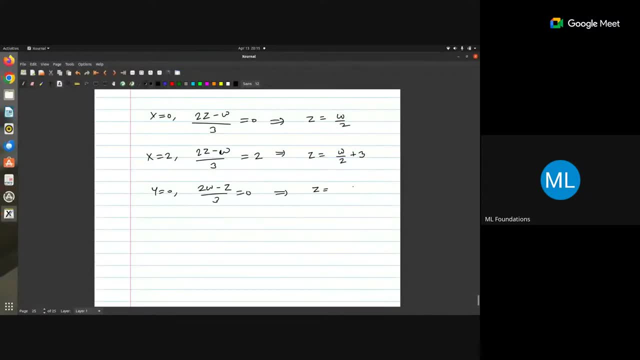 two minus z, by three plus zero, which gives me plus zero, which gives me plus zero, which gives me z equals to z, equals to z, equals to. here we find value of w you know same thing. it's not like because i need to find, because there are two x's right. one is initially it was x and y axis right. so i here what i'll. 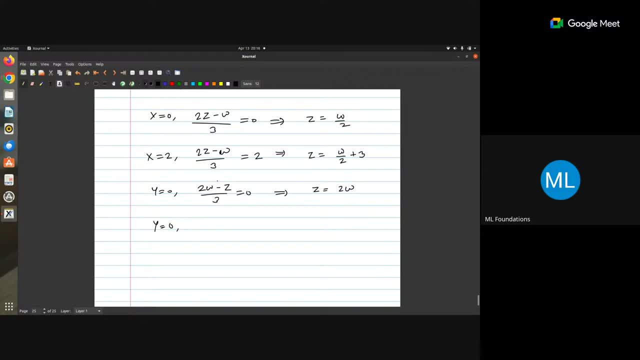 do is w and i'll plot w and z, so i'll make all this. uh, this will basically these are the lines only right: w by 2 is one line. w by 2 plus 3 is one line, right? yes, so when you have the equation of line you generally you have in this way right: w equals to 2x. 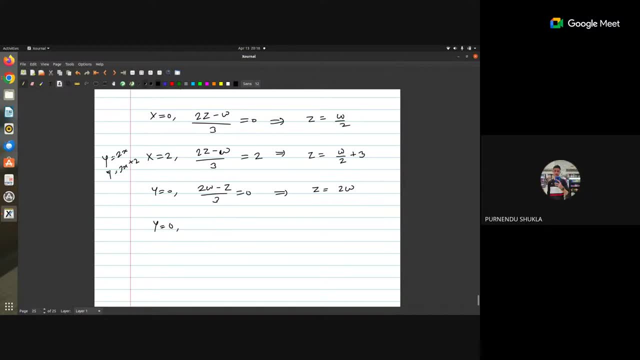 sorry, y equals to x, y equals to 3x plus 3, something like that. so everything i'm making into uh one variable: okay. so this w by z. okay, minus three, three equals to three. it gives me what uh z is. that equals to nine. nine by two, nine minus nine by two. nine plus two, two nine minus. 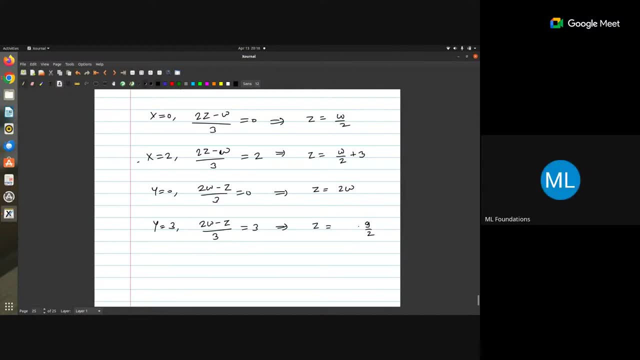 nine plus two, two, huh, right, so two w minus nine, nine, right, i know that uh, nine minus nine minus two w is equal to minus z, okay, so, so i'll just change one one thing, i'll, maybe i'll just uh make all things into, let's say: 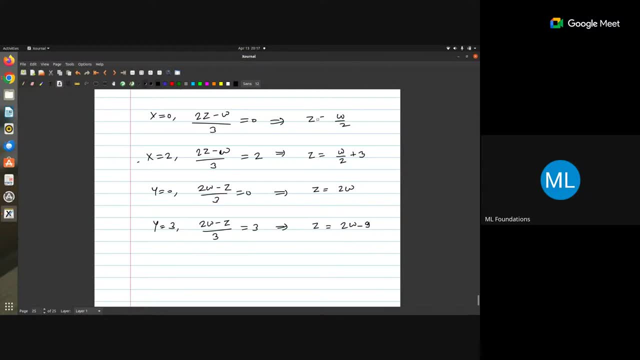 w will be my y axis, let's suppose. so sorry, w will be my y axis. so in that case, what will happen? uh, w will become 2z. it's okay, it doesn't matter anyway, but uh, let's say w. uh will be equals to 2z minus 6. 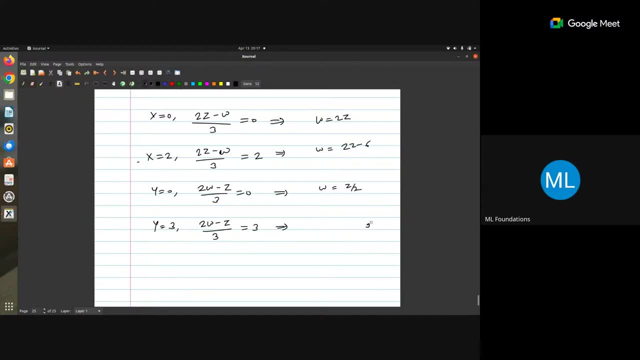 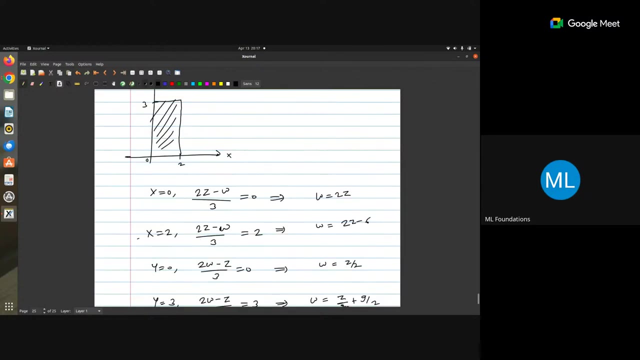 and on the second, the y axis, and in this case, if we plot it here, i have okay you, i'm glad you see that y is v, so j is solid here. w is equal to z by two and w will be equal to 1 by 2, z, z by 2, my, my. 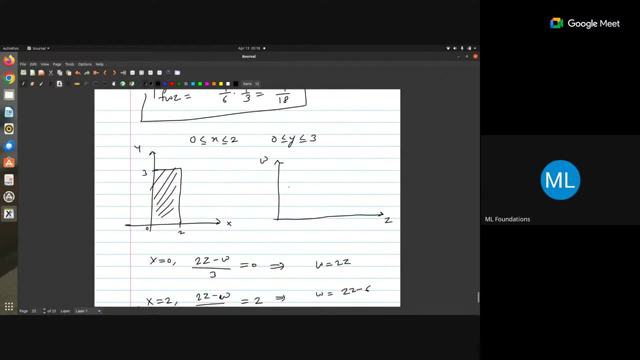 plus 9 by 2. okay, it's okay, yes, okay, okay. so if i wanted to plot this, here is that is w is w, w equals to 2z will be how how this will look like. this will be somewhat here, right, correct, yes, so how do you find we took z as a horizontal and w at vertical? no see, you can get. 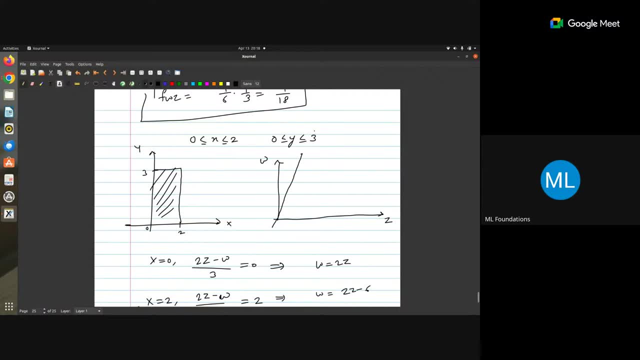 like w into uh, horizontal and z. it doesn't matter actually, right, you'll get some, okay, so but it because the dimensions you can look into, like uh, however you want to look, you can look at. currently, you understand this, it's w and z. are this uh? because, okay, i'll tell you that. 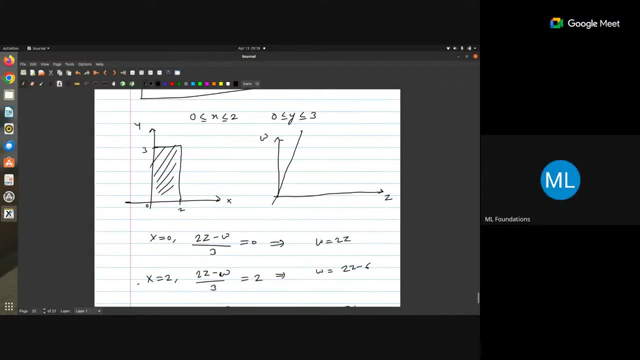 we took w or z. yeah, just no, i'm just trying to show you the support, so just look into this first. okay, we'll discuss it later, maybe. so this is: w equals to 2z. uh. w equals to 2z minus 6- uh. how. 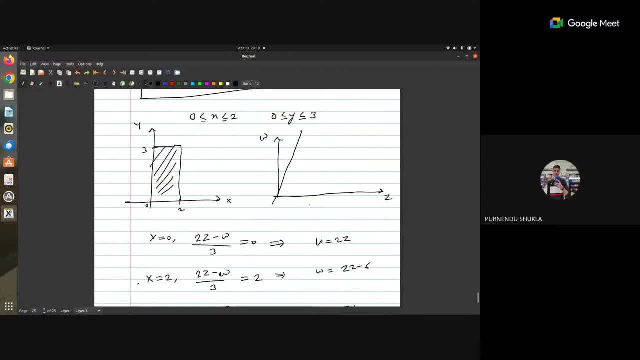 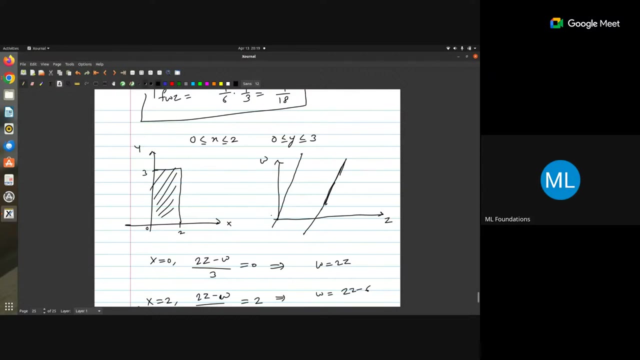 it will look like shift. yeah, so it will be like somewhat right. yes, correct. uh, then w equals to z by 2, because the slope will be lesser. so this will, uh, this will become what this correct? this is w equals to 2z. this is w equals to 2z minus 6.. uh, this is w equals to 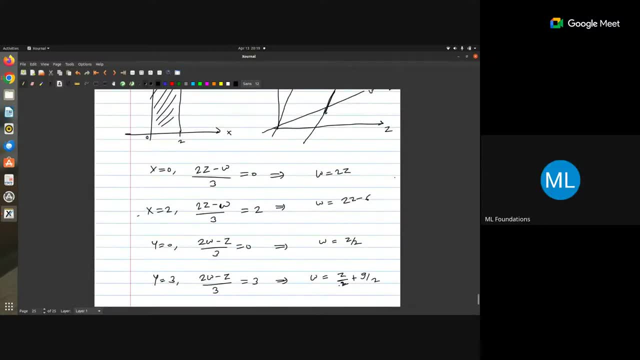 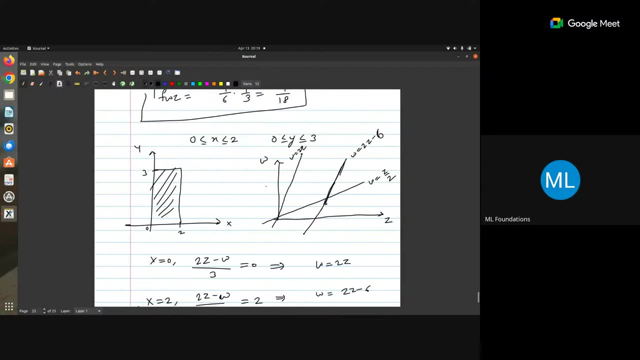 z by 2.. and last is z by 2 plus 9 by 2.. so this will be like this: here, somewhere here right 4.5 around 4.5, and the slope will be similar as that of z by 2.. so it is w equals to z by 2 plus 9 by 2. 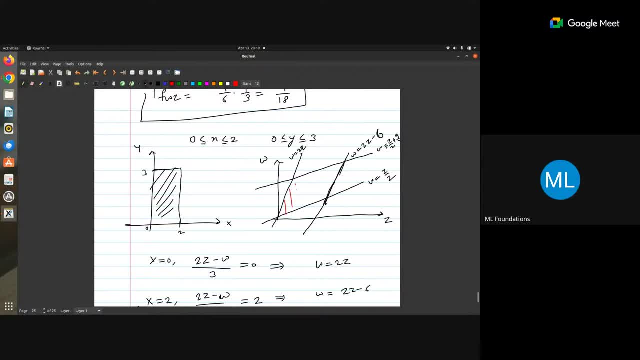 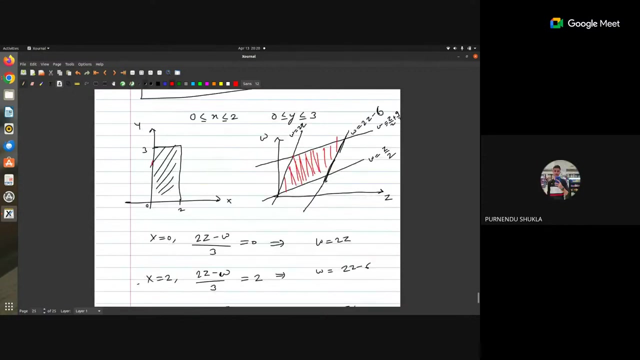 so now the support will be what? so? so initially, support support for x and y was uh. rectangular support is rhombus and generally you will find this kind of support there and this is a linear transformation. actually, yes, right, actually i could not understand why we do that. no, no, to understand the support: uh in if 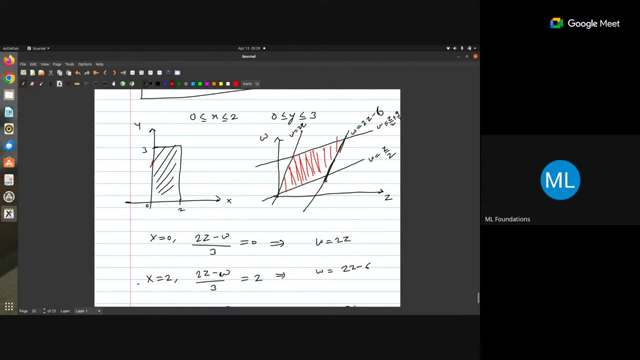 you have x and y in this fashion and let's say x and y are dependent on w and z. you have got the joint density function for x and y. so generally you find the probabilities by using the joint density right. so what is the probability here? it's one by six right area under this curve. what is the probability here? 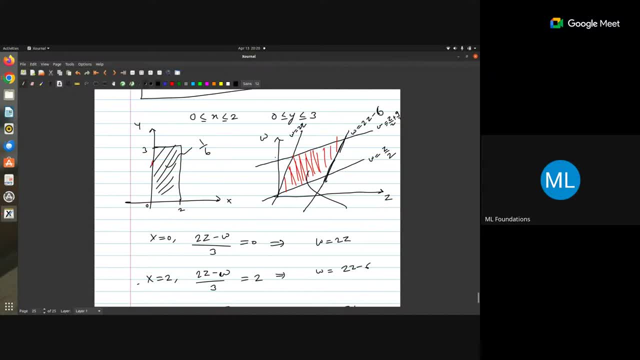 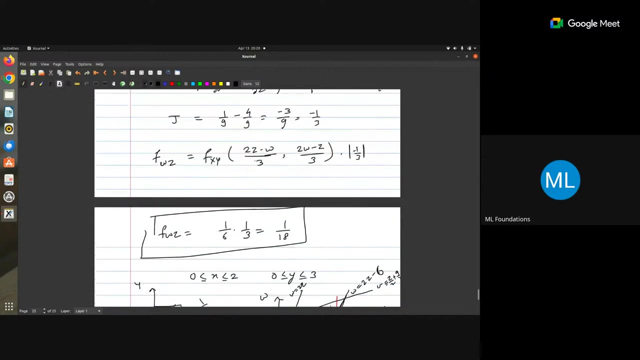 to find the probabilities. you you need to find what support correct. then only you will find the joint probabilities right and this, this will. it will come as 1 by 18.. but how you calculated that one? we have already calculated here. okay, support, but i want to know, means we already have random variables, so which can be used to define any. 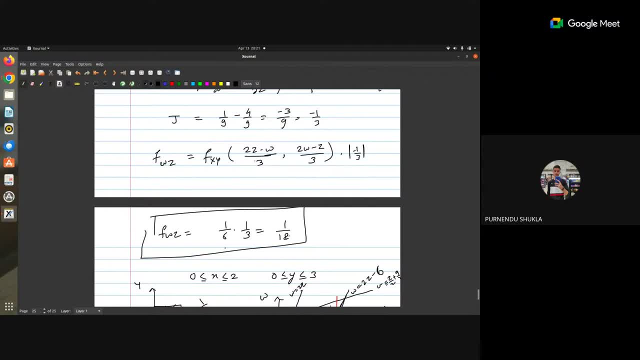 possible outcome for an event. but why do we need function of random variables? therefore, these type of functions there is uh, okay, so transformations are very much needed. so you have learned, uh, the linear algebra, right, yes, so what actually we do there generally, like, what are those transformation? linear algebra? i'll like 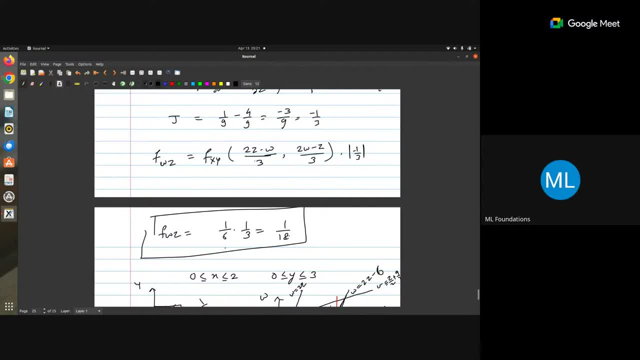 kind of uh, transformation, right, like to what is any matrix actually? it's a transformation actually, but generally okay, but generally it represents some vectors, right? or maybe you can see this system of linear equations. let's say, 2x plus 3y is equal to something. to express something: 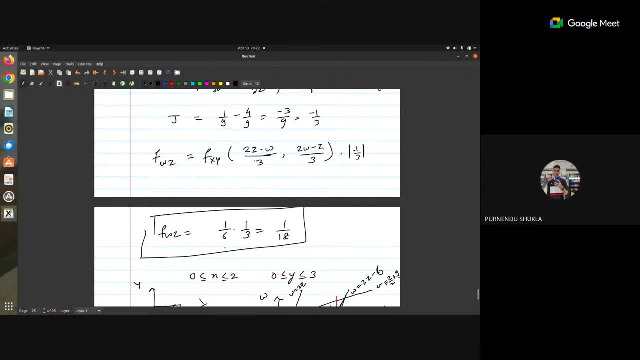 uh, 2x plus 5y is equals to something right, consider this as some functions of random variables. okay, and now the try to visualize there in: uh, you know three dimensions or something. so usually what you do is you try to solve some- uh, you know linear algebra you. why you wanted. 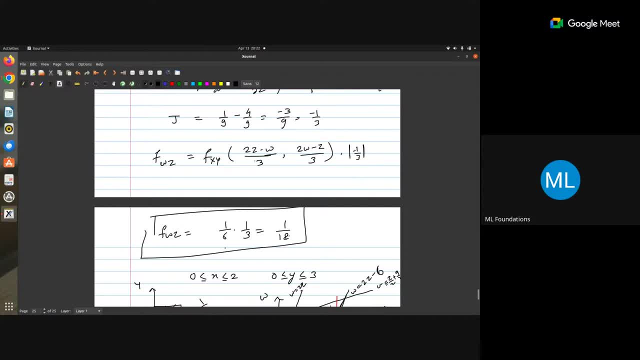 to solve that one: x and y. x and y are what? basically, those are solutions, actually solutions. but uh, initially, what are they? some random variables, only right. or or maybe some variables. they are variables, right. so x and y are the variables, they can take any values, but i wanted to find some optimum value, correct. 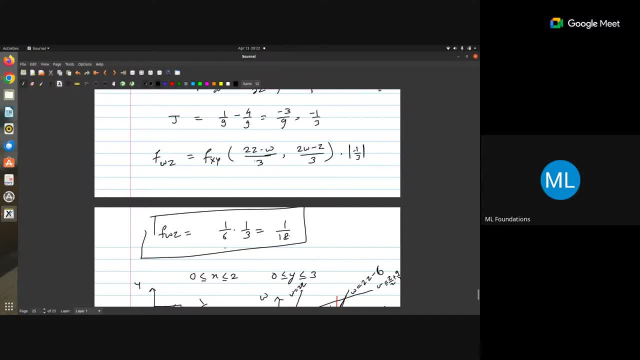 that's why you use their linear algebra and to find that what you do generally, you, you do the transformations. but why do you do the transformations there? without transformation are you not able to? sometimes it's not feasible to get the solution directly, so we change it in some linear fashion. 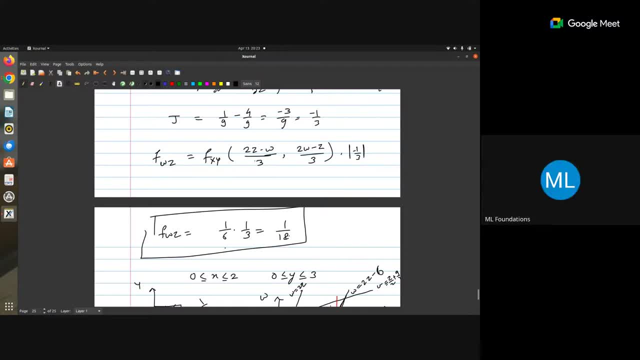 that we can. yes, here also there are. there is, there are possibilities that, uh, you may not get the solutions right. so what you have to do, you have to be able to change the variables, transform the variables and then find the probabilities. so the means in context of machine learning, uh, for matrices and linear 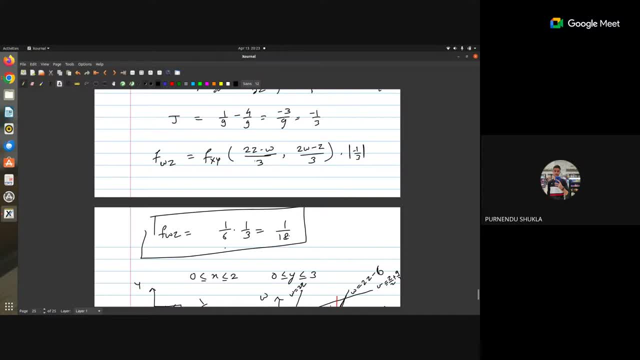 algebra that is required for calculating the different things in, uh say, features and labels. but this transform random variable how it is relevant is there. okay, so, okay, so okay. but then you if you see why the probability is necessary in machine learning. first of all, in general, because we need to map an input to an output. 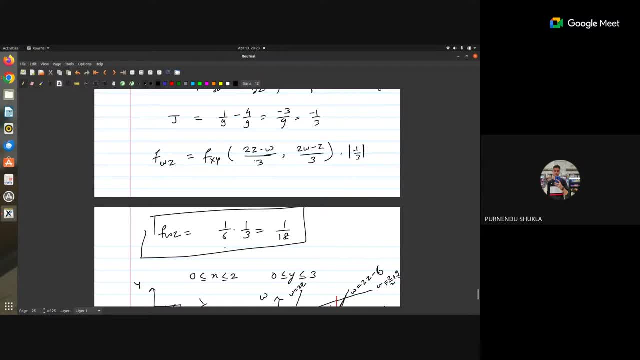 in such a fashion that which is the most likely that will happen. okay, so you are saying that there is some input coming and you will have some algorithm and you are just putting like getting out the values, right, but that algorithm inside, uh, is basically dependent on what those features or 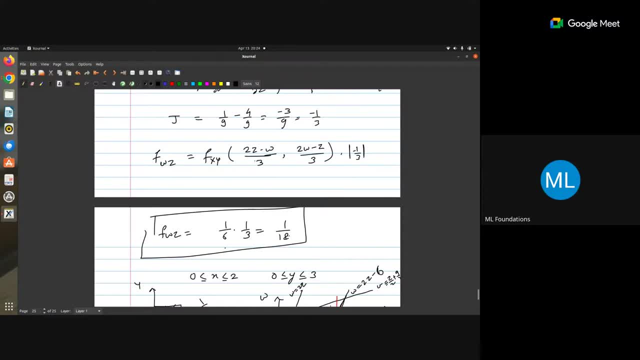 features. okay, those features. so let's say, these features are random variables. okay then, uh, what do you need there then? some transformation functions, right, generally see if you see that, uh, algorithm itself or may, the first, first week of this machine learning is what you have: some input. 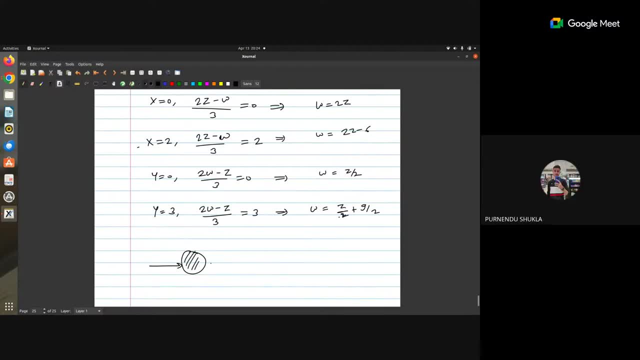 right, you do some. there isn't some algorithm- and you will have some output. output can be in terms of classes, you in terms of, uh, some values or something right, but generally they transform to the probabilities. yes, and from probabilities you say that, okay, which is the highest probability? 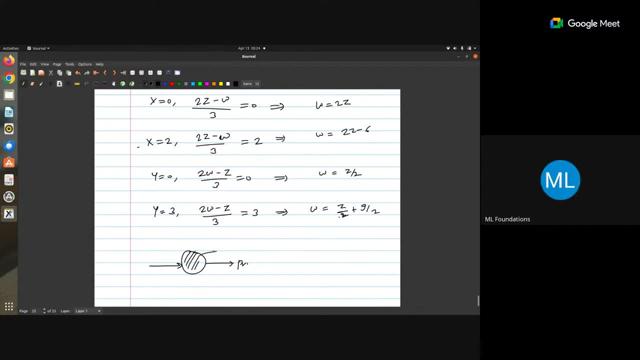 you will go to that class. but these probabilities will come from what? some function, right, some function, and there are basically some sigmoid function. is there function? yeah, you know this kind, you know some this kind of functions, but these functions will take what? some random variables. variables, yeah, do you understand now? so they- this is like. 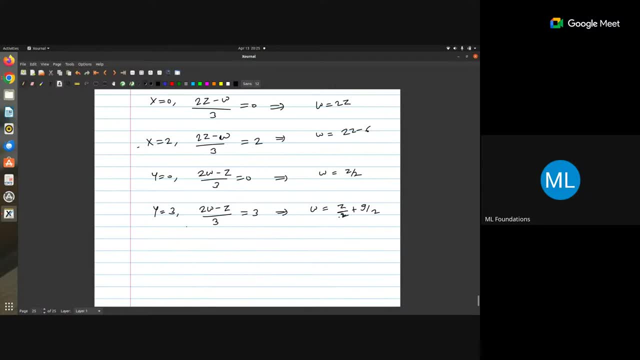 it's. they are all interdependent. uh, like, everything is interdependent here. so if you wanted to find the probabilities, that means it comes functions. functions are dependent on some input. x, x is what. these are the array of values, right? array of values, now this like big data. these are all array of values. are stored in what matrices? right, you try to get into some. 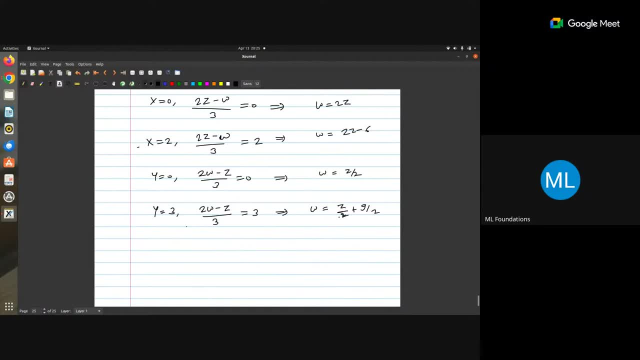 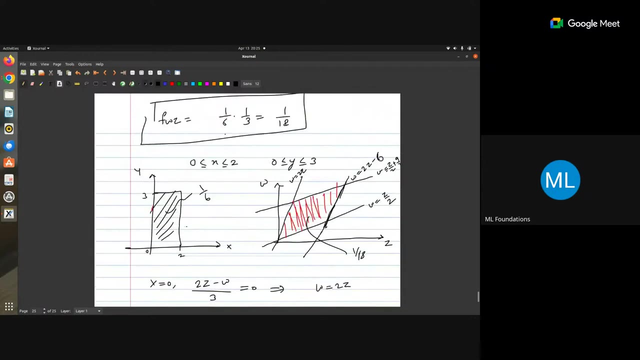 values. you make them into some like simpler values. let's say, now that becomes input to your function again and then that becomes a random variable or something, and then you just try to find the probabilities from there. okay, see this, this you are not doing it manually, anyway. 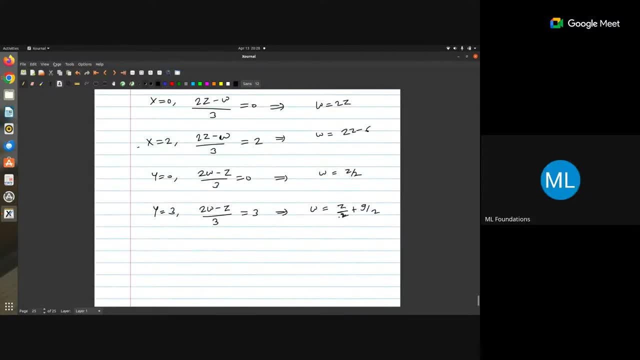 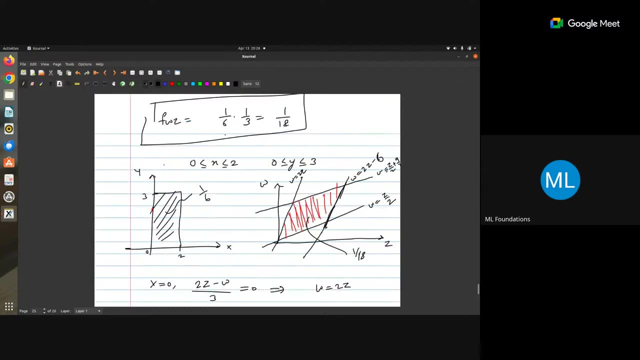 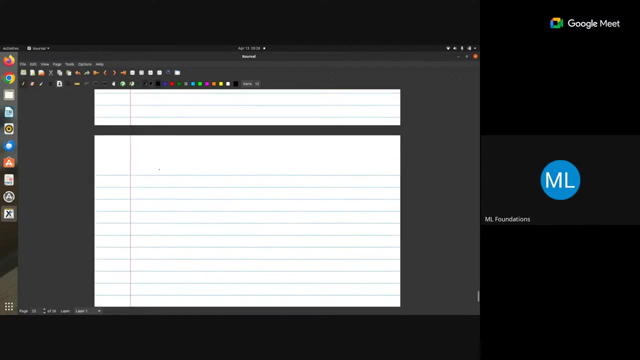 right, this, this things you uh for you, but you should understand how the machine is working. and better way to understand for human being is what uh, by doing like for two variables or single variable right and then you can just find it out, okay. so i'll just take one problem uh from. uh like professor's lecture only. 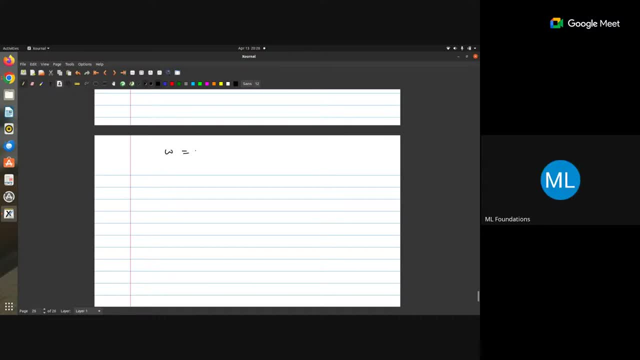 can you just try to find out, uh, the joint pdf for that, and will this uh? so let's say w is uh uniform in 0 comma 1. okay, x is uniform in, let's say, 0 comma 1, and, and i know that w and x are. 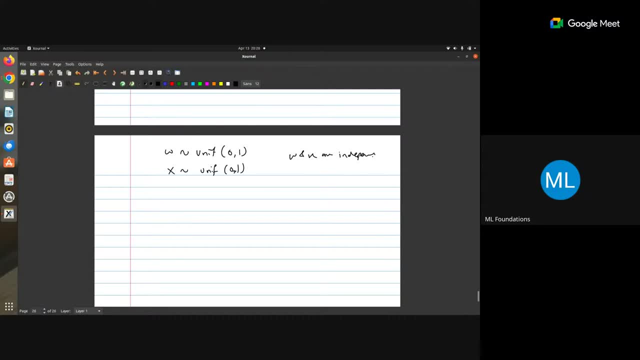 independent, okay now. so, uh, i know the thing, like the individual distributions here. what does that mean? and if they are independent, what does that mean? can i know the joint density of these two, w and x? from this information, are you able to come up with, uh, joint density? 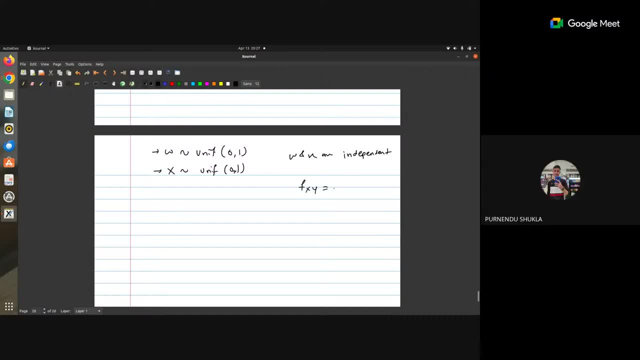 it's independent. so that means so if you can add those or multiply those, multiply right, marginal densities. this is independence, right? that means, if i have these two distributions, i can definitely have wx. right now, let's say some other. uh, variable y is such that it is a function. 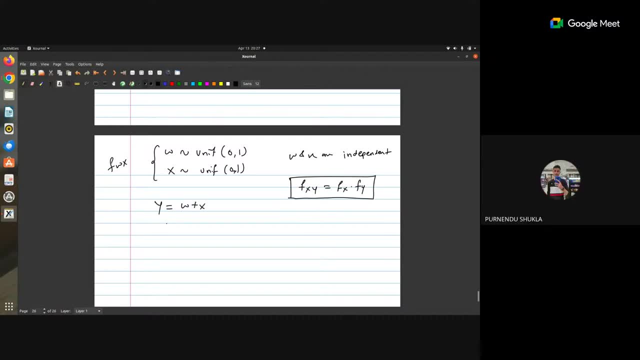 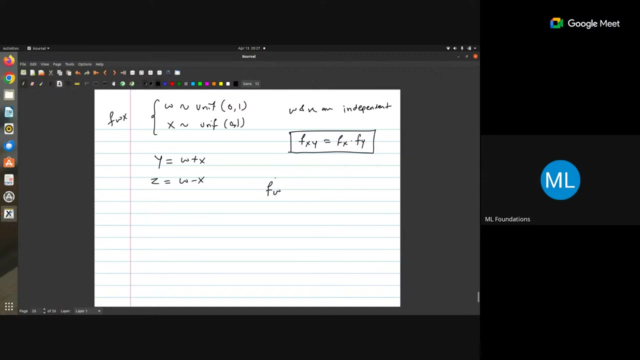 it is a uh, sir, but here this fx and fy. we need to find that right. yes, yes, definitely you have to find it out. so now i defined these two variables, y and z, can you find out f, uh, f, y, z for me this, take uh, let's say five minutes and uh, we'll see the solution. 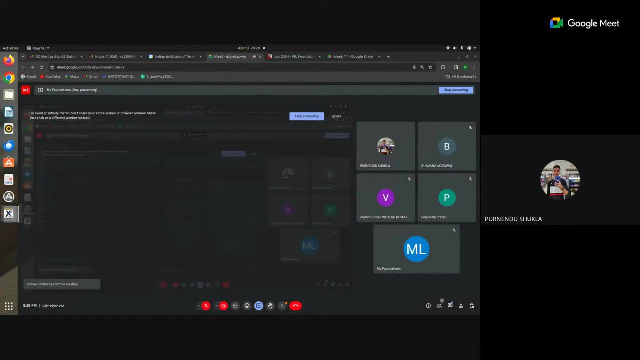 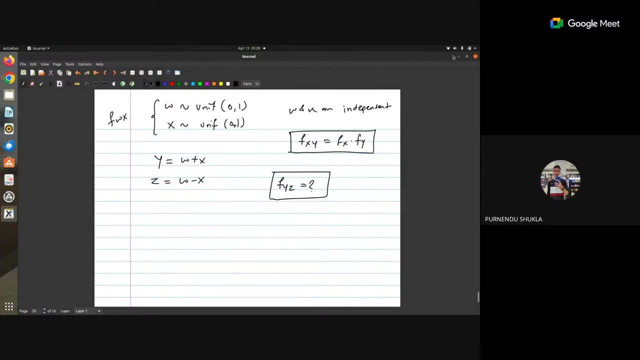 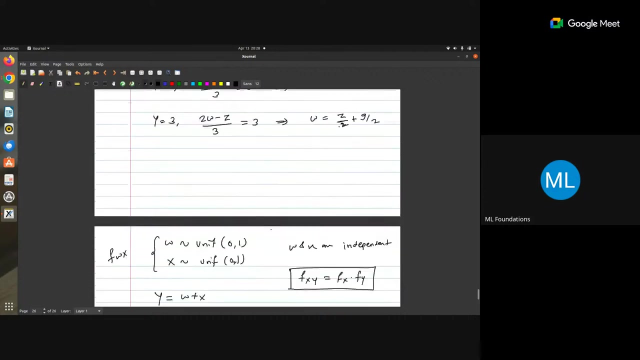 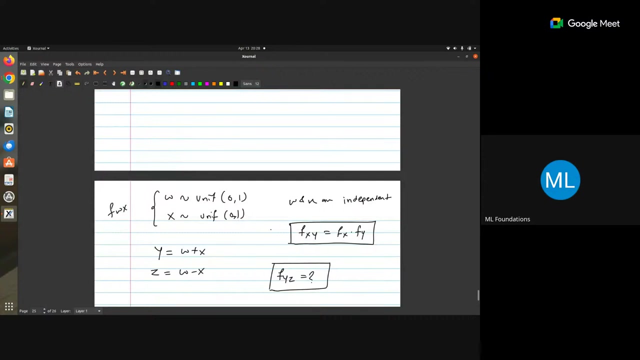 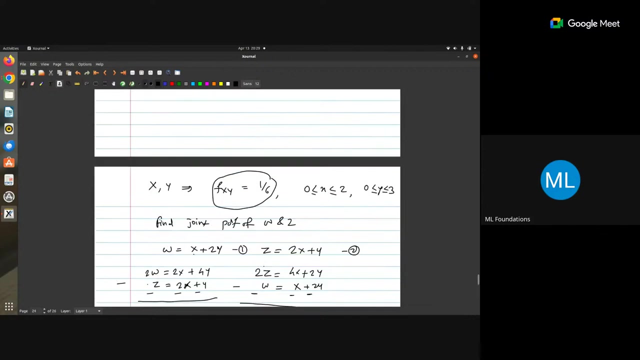 do you need the formula? he just said that was the first time that we saw it. yeah, yeah, first of all write down this problem, right, fine, and now? so how you think: yeah, okay, done, okay, I'll just show you the formula here. yes, now try to find out. join to. 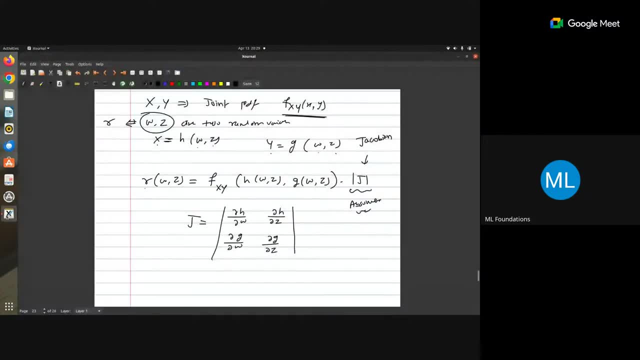 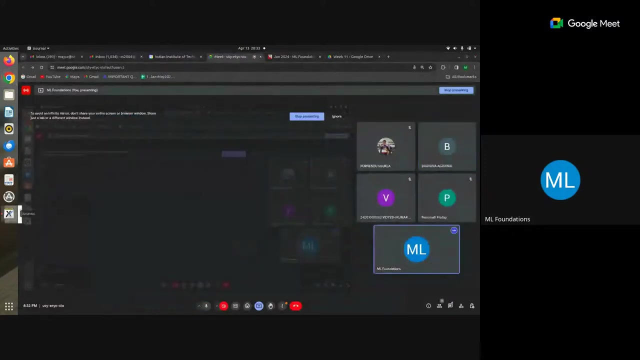 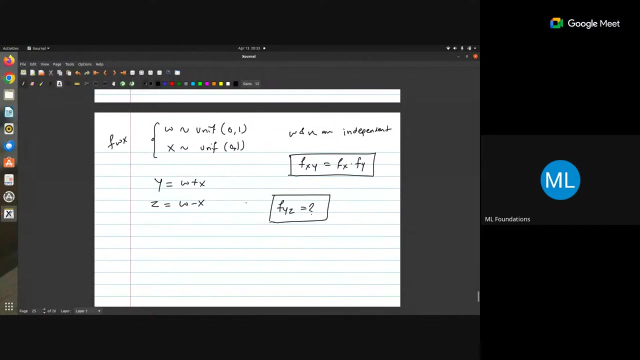 forget: you, you, you. so in this example you find HW said: but in this you given question: hello, sir, you, you, you, you, Okay. so is it done? Okay, let's try to find it out then. Okay, So what is a fix? Or maybe, if w of w is here, 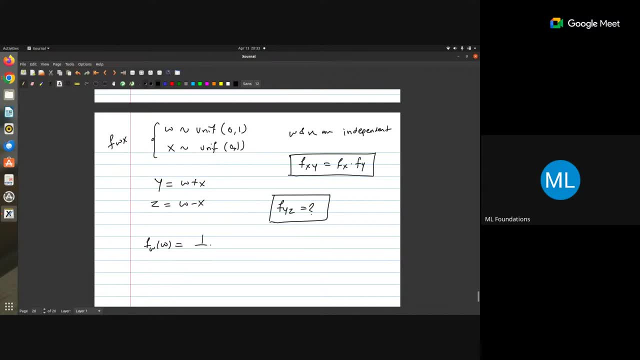 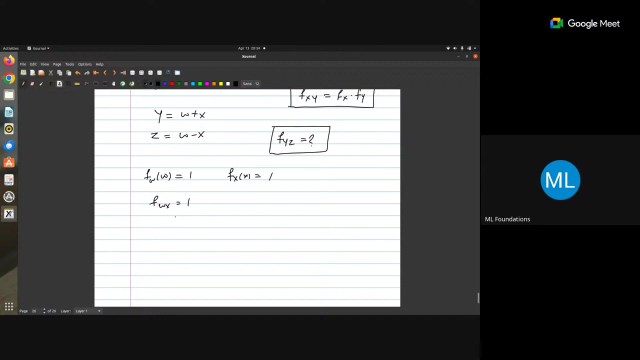 one upon b minus a right, So here it's 111.. Yeah, And what about f? x of x? It's one And it's also one. So if f w, x is one right, Multiplying both. So this f w of w into f x of x equals to one right. Now, 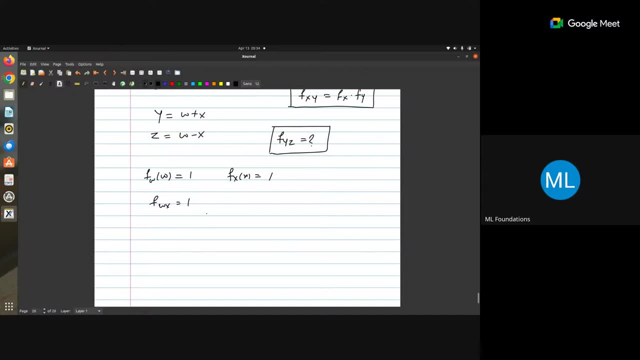 what about it? So let's say this there Now: this y is a function of w plus x, and z is a function of w minus x. What is Jacobian here? Jacobian will be del y of w, del y of x. 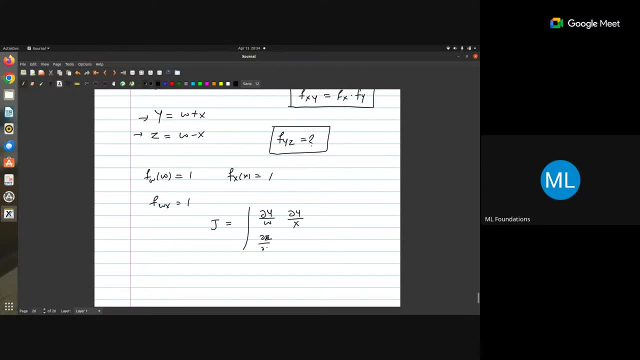 Right, And del z of w and del z of x. Okay, What is del y of w? One, Okay, Sorry, sorry, I think I did the mistake here. So this is one right And I need to find, first of all, 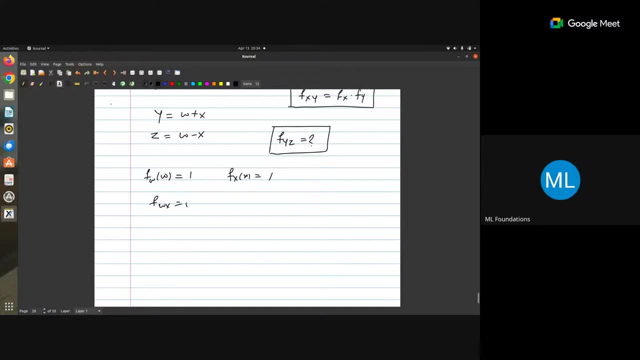 w in terms of, because this is an invertible function. how, how can i say that it's invertible? so, from yeah, so w will be what x minus y, no, y plus z upon two, right, yes, and x will be what y minus z. right, you are subtracting the both. the equation. 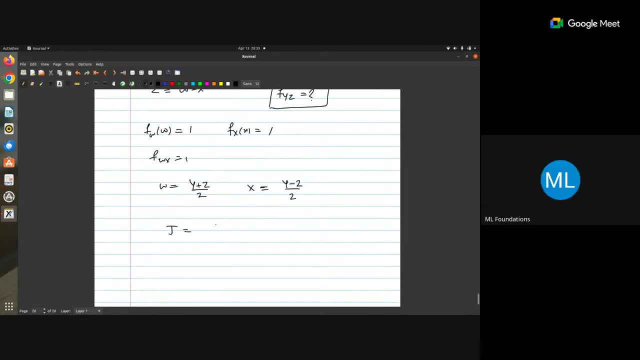 okay, so, and jacobian will be what del w of l y, del w of del z and del x of del y and del y, uh, elixir. well sir, how do you define this jacobian? you can see that right. no, no means. what is the? 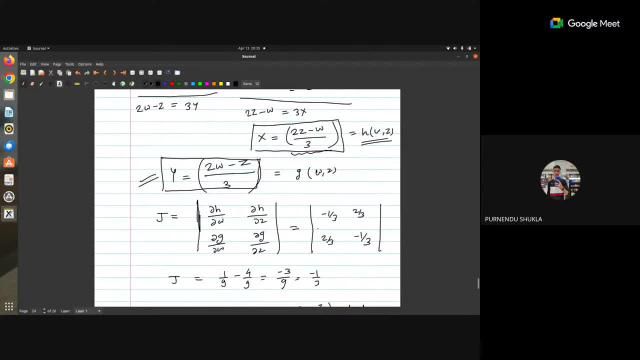 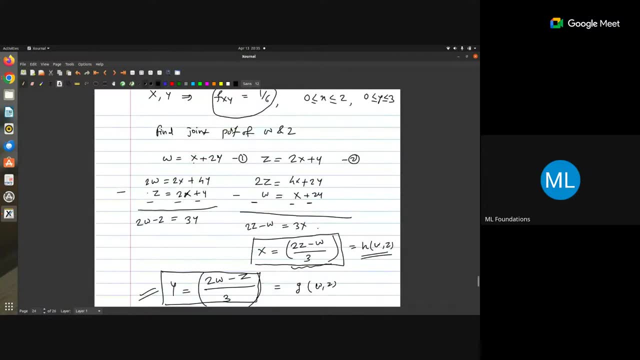 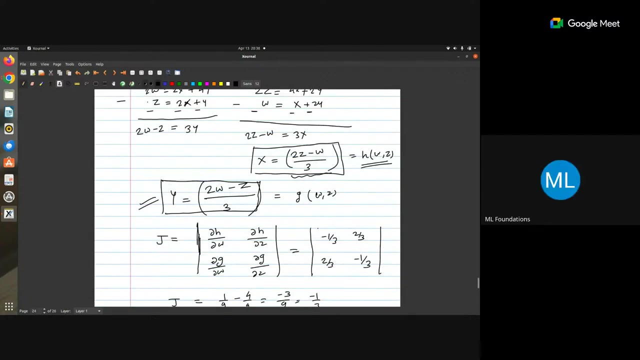 procedure, which which we take first ordinance, like yeah, yes, sir, that's right, okay, okay, so actually. so here you can see that, uh, so x, y will be our function here. right, so, okay, maybe else. okay, say here we put x, h as h and y is at g. oh you, you did it. uh, like, uh, opposite. 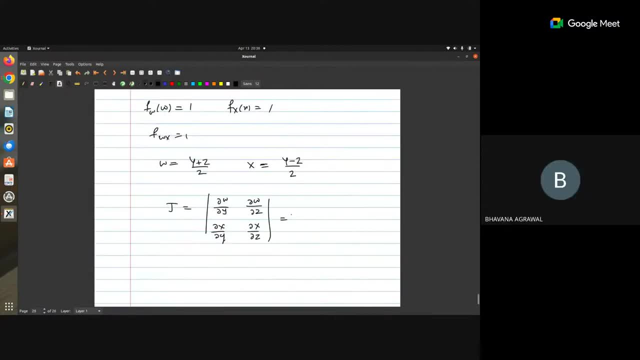 so you, i don't, i don't think that will change anything. yeah, it's okay, but i think it will change only the sign. right? anyway, jacobian, we are defining for: uh, absolutely, absolutely, first take w and then we take x. yes, so here, what will happen? it's okay, it's. 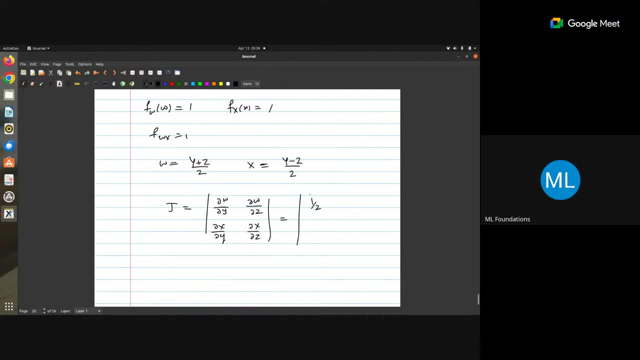 okay, i, i, if i take this one, what is your value? uh, came here for jacobian with your uh. you have taken some w and x later on, right? so what is your value, sir? one by two, uh, one by two and one by two, final, final jacob, you will see this, minus one by two, it's a zero, zero, zero. it will not come. 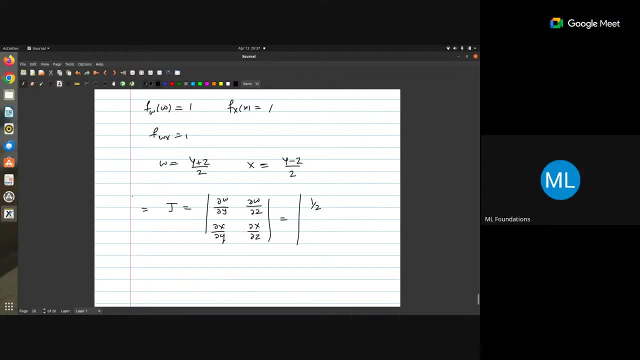 if it comes to zero, then it's not going to go zero. i don't think it is coming. so here you can see that w del w by del y is half del w by del z is, let's say, minus half, minus one by uh, minus one by two, minus one by two, right? 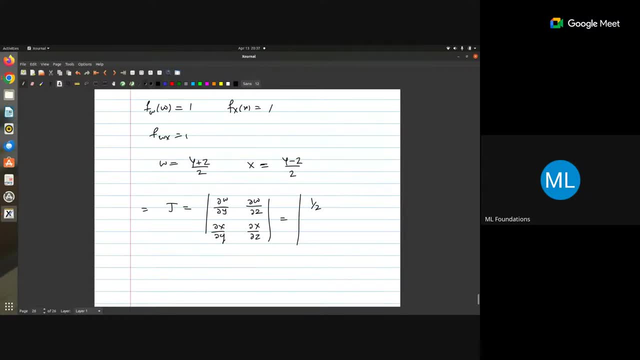 huh, that's correct. so you see, it's minus half here. okay, so, uh, and the next uh with respect to this will be half. yes, sir, y f z is equal to one by two, correct? right now, this will jacobian will be. uh, it is minus one by two into. 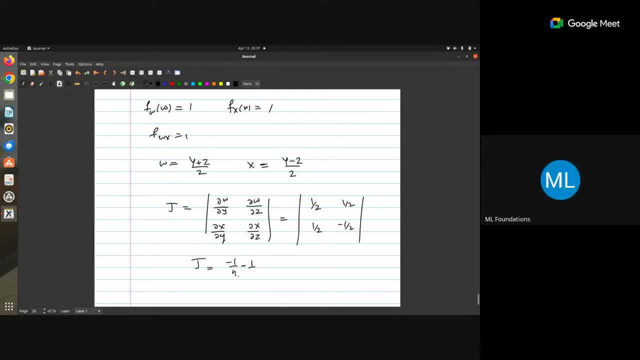 sorry, minus, then by four. sorry minus one by four, minus, uh, one by four. so this will become minus one by two. so yours also is coming same, right? you know the property of enemy, right? if i change the row, what, what will happen? only the sign will change, right? you know the linear algebra part of determine side. 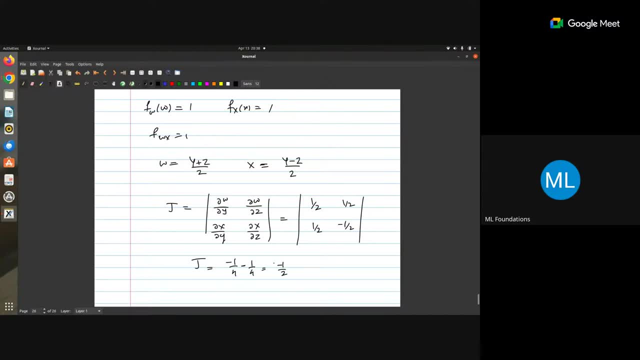 how you work with that maintenance. it will not change anything. it will just change the sign of the. it will not change the value right and that's why we are deixar algebraic part of the right part. it will not change the value right and that's why we are프� Kon grilling, you know it will not change anything. it will just change the sign of какое田가idade 빈, 3rd Beetle. it will not change the value right and that's why we are 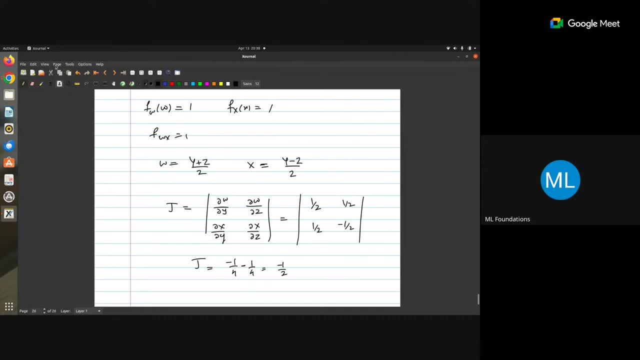 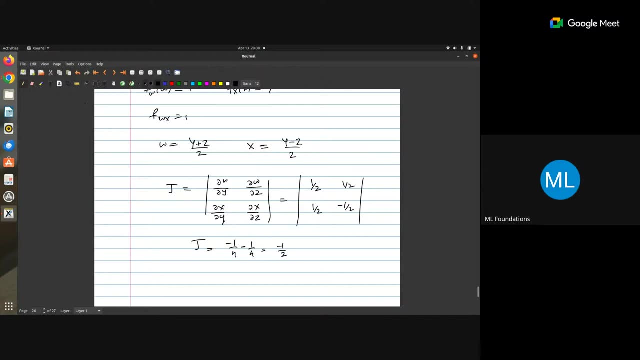 it doesn't matter how, which order you are taking this. you understand what are the properties of determinant. if I interchange the row, what will happen? only sign changes, sign in changes, values remaining same. so if I use del X by del Y in in the first row and del X by del Z in first row, and then W by del Y and del, 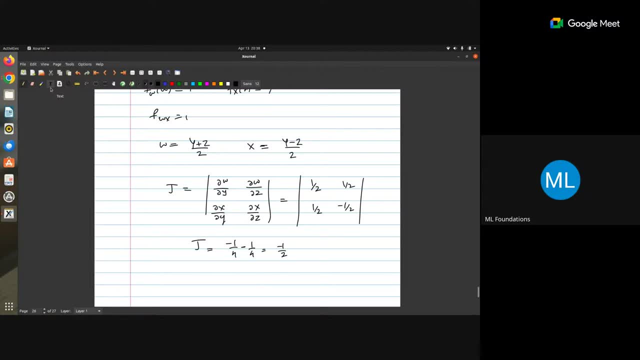 W, what is in second row. what will happen? nothing, it will just change the sign. similarly, if I take del W of del Y and del W del Z in in column wise, what will happen again? so that is why you need not to worry about, because if any change of 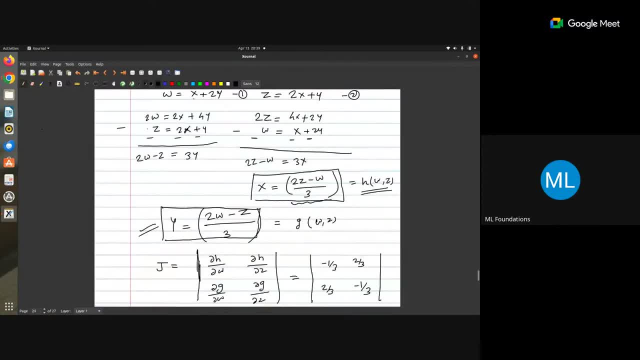 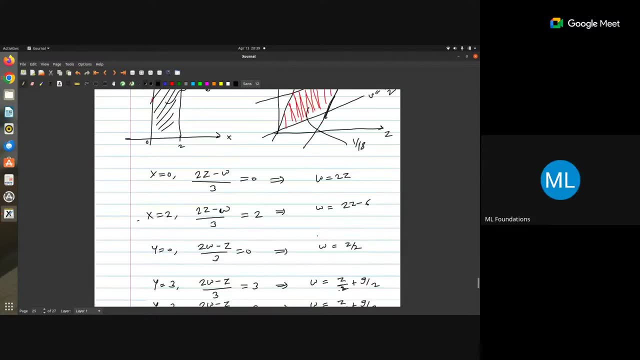 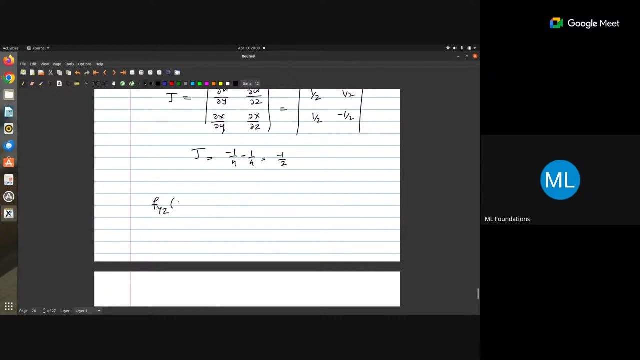 sign. it will be very accommodated here, because our formula is what it's absolute value right? so for everyone it will. the answer will remain the same. so now, if Y, Z of Y, comma Z will be what F, W, X of this, Y plus Z by 2 Y? 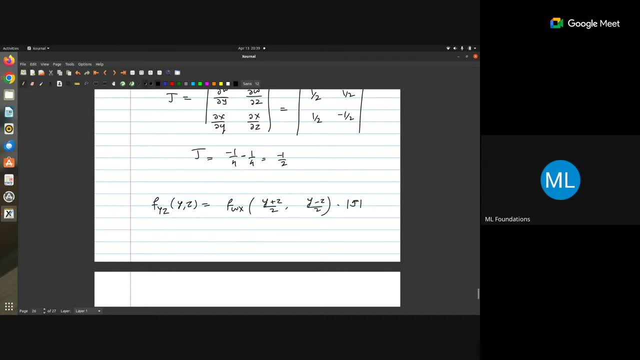 minus Z by 2, into what is it? F, W, X of any X and Y is what? so W and X is what? 1? 1, 1 into half, so the joint density will become 1 by 2. you understand this here, this F W X. I got it. 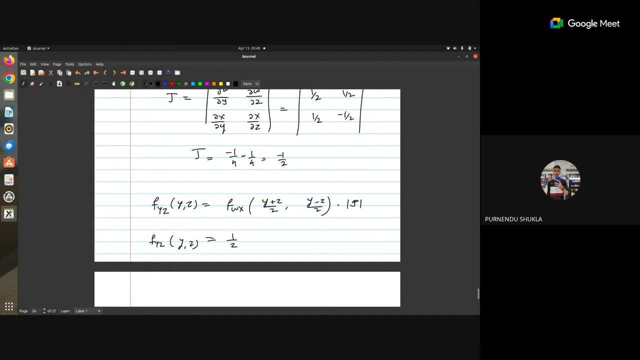 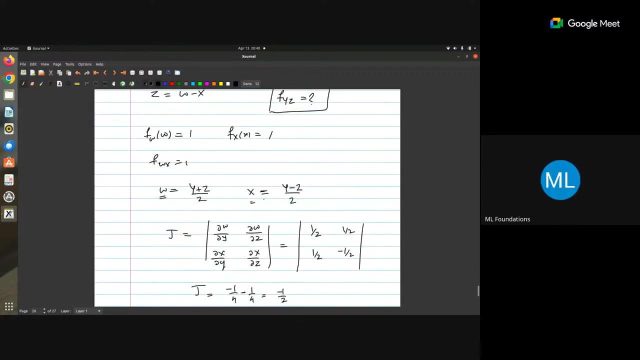 is 1, okay, and J also. we got like minus half okay, but this Y plus Z by 2, this part, this is X now, this is W now and this is X now. this we have found out here, right, it's W, this X, and our joint density is substituting: well, yeah, and our joint. 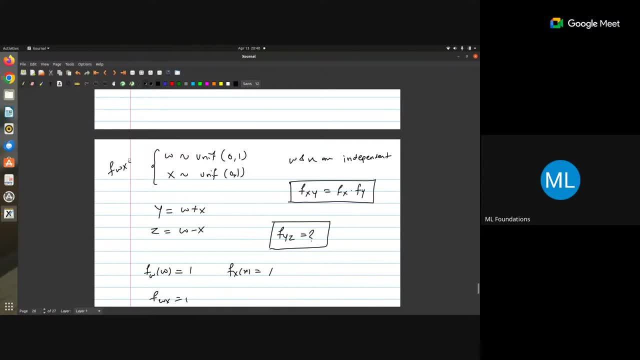 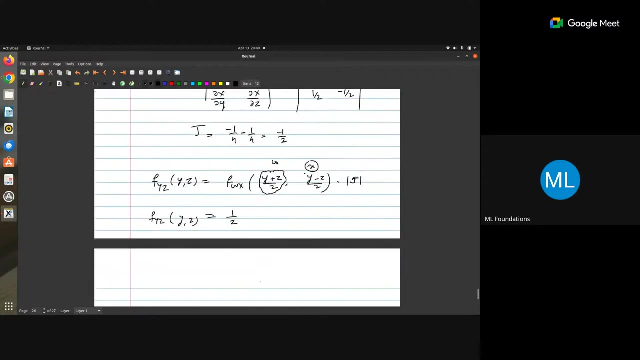 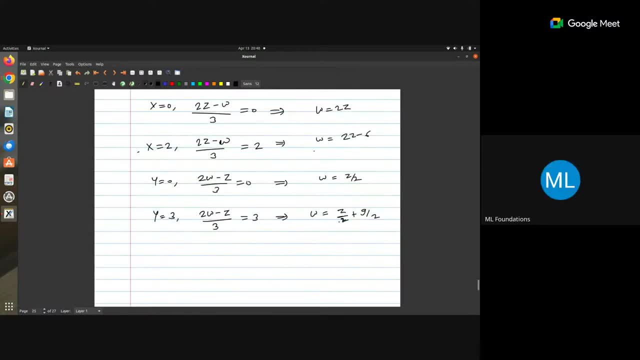 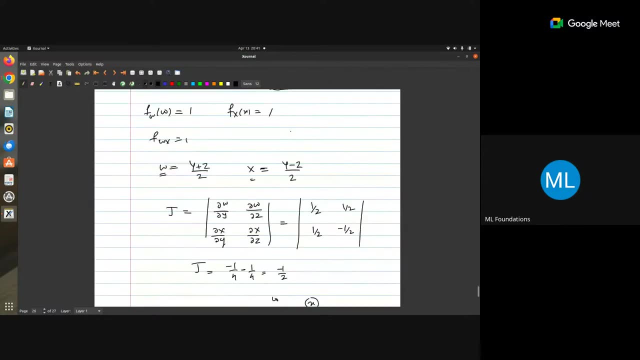 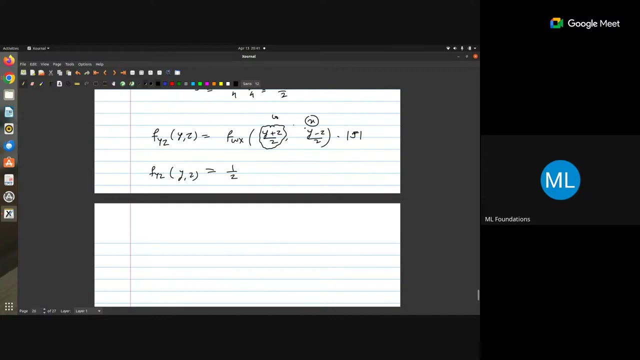 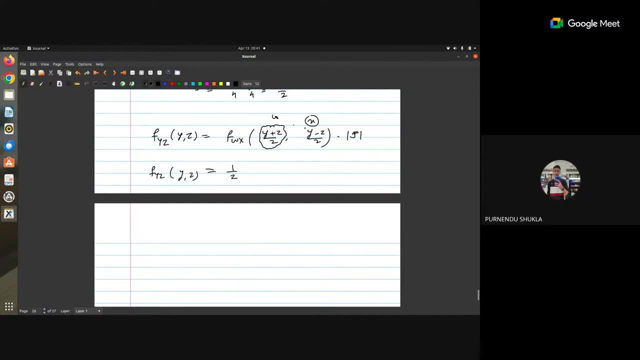 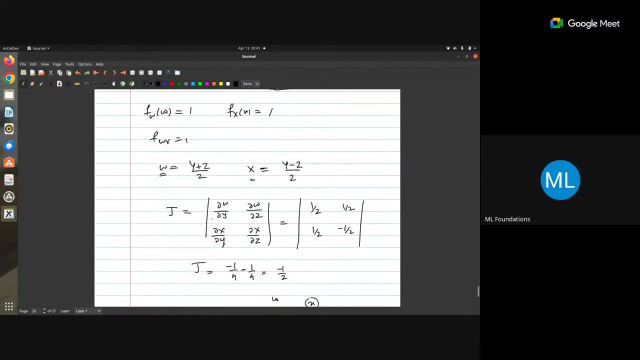 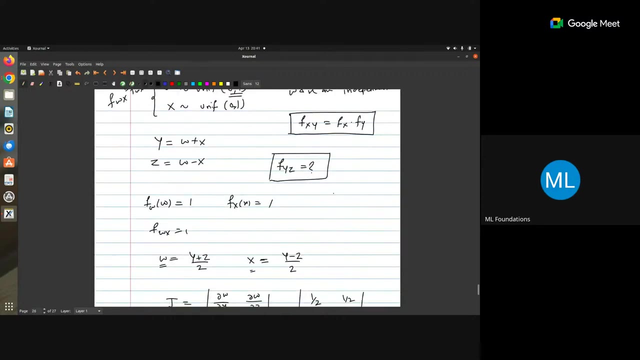 no, this is joint density, a sample, right. so okay, what is the support? okay, what is w? it was uniform between 0 and 1 and x is 0 and 1, right? so if i draw w and x here, suppose w here and x here, so w is 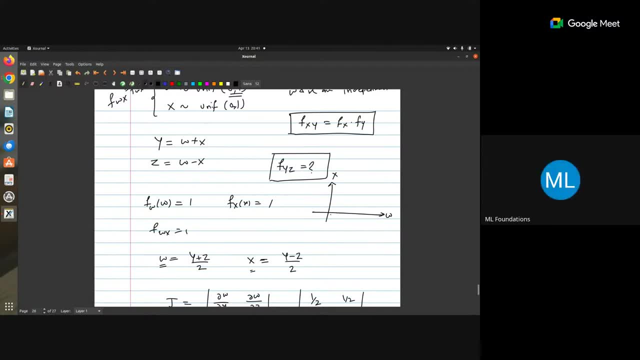 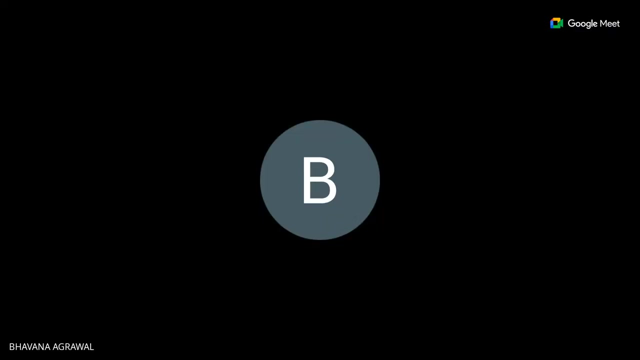 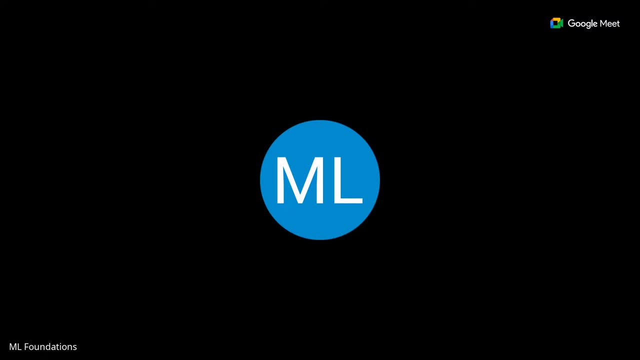 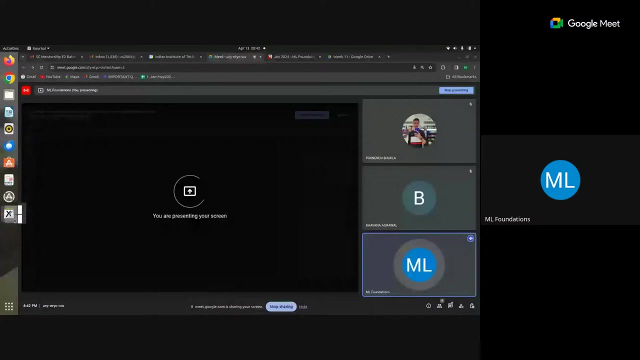 the support was here, from zero to one, zero to one here and three. So you're dead. and why Visible? Oh, okay, Screen is not a good one. Okay, only two of you are left here, I think the other class. 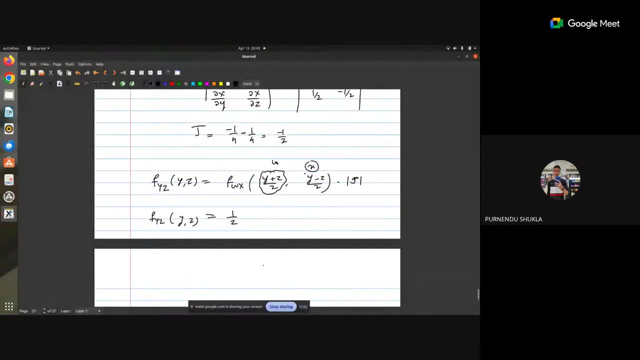 is going on right. I, I don't think there is no class, at least in my calendar. Oh, there are some few subjects where having the, let's just say this: Maybe I haven't taken, I have, yeah, Elephant TDS, Yeah. 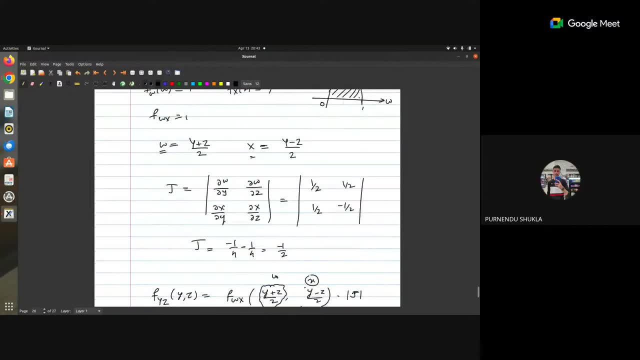 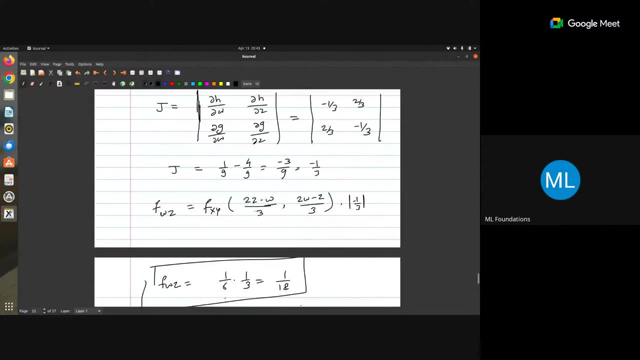 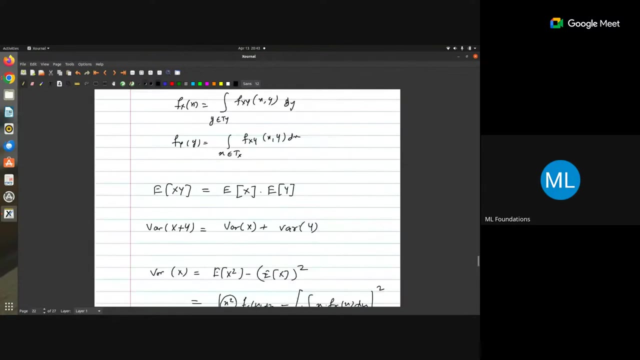 TDS is not there, PDS- I think it is having PDS. Okay, Uh, so basically, this is transformation of random variables. Uh, but I think, see, okay, this topic is very new for you guys. Maybe I will go through that one more time. uh again, Uh, okay, I'll try. 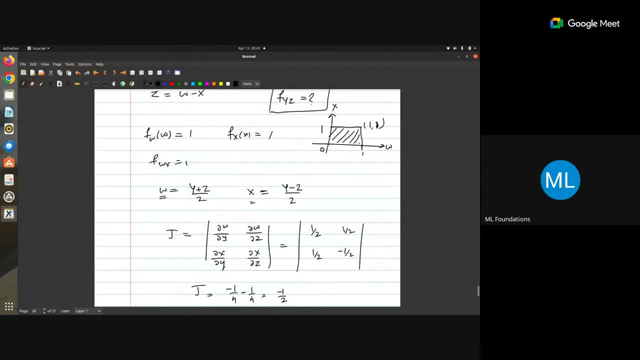 to show it again: We, we, we're not able to uh finish off any solve with the slides, So I'll just share you the slide, solve with the questions with you. Uh, you try to solve them later. One more thing is: uh, okay, I think we are left with. 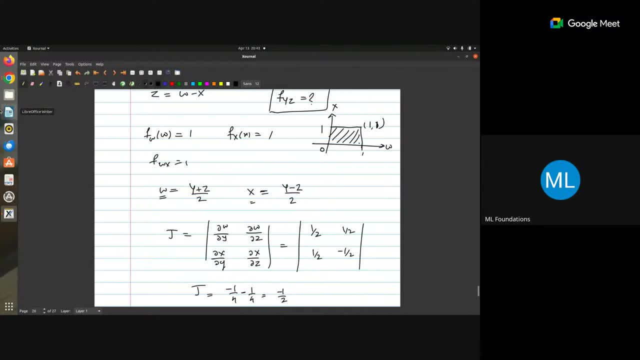 what uh inequalities? maybe we'll uh try to see it later on. Uh, inequalities are not 11, week 11. So I haven't done week 11 actually means I just started. Yes, Recap in week 11.. Actually I'm very like, But but eleven and twelve, uh deadline is at. 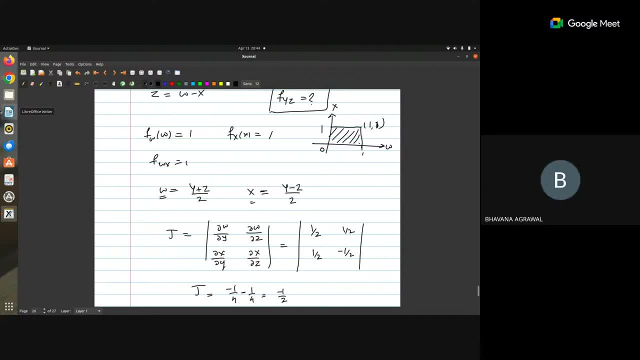 the same time, right? Yes, sir, No sir, Okay, Uh well, I think it's different, sir, It's different, It's different. Let me check, Is it tomorrow? I don't know. Okay, Okay, Fine, Fine, No issues, Sir. So it's the best. nine out. 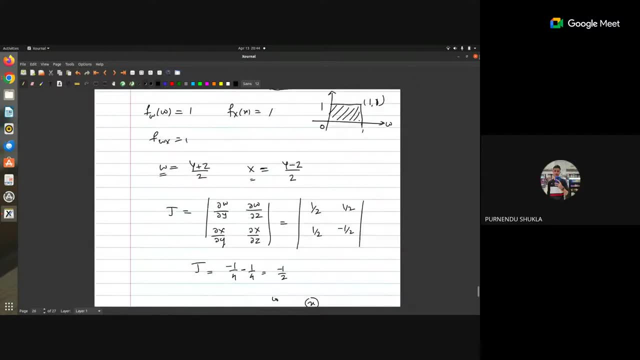 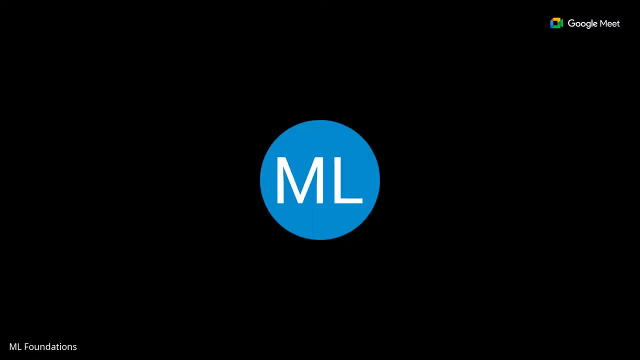 of twelve days. Yes, Yes, Yeah, Yeah. So I got hundred so I can take the chance there. Uh, okay, So that is fine. Uh, so I think most of you guys uh don't have to worry about I. 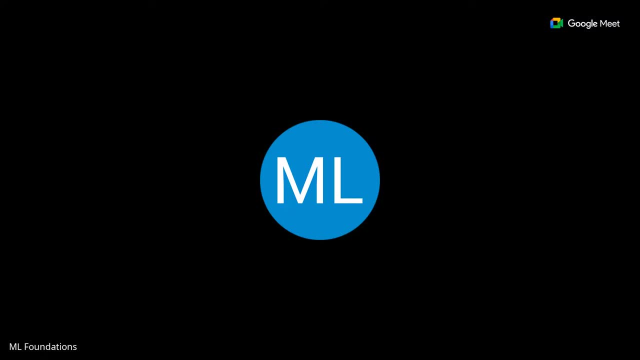 don't have to worry about it, But uh, okay, So next week what we can do is, uh, week twelve, because I think all of you have gone through the parameter estimations. I'll write down some questions and directly we'll solve. uh, try to solve. 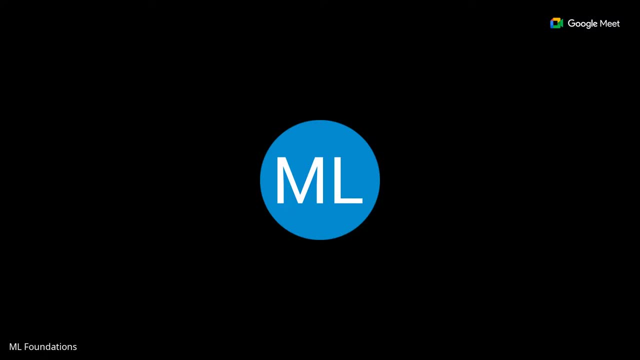 those, Uh, just make sure that. and one more: I think the topic remaining is inequalities. So inequalities estimation, you means estimation of parameters using ML. Yes, ML method, Only ML is there, Uh, not MMA also, sir, Or both are not there. 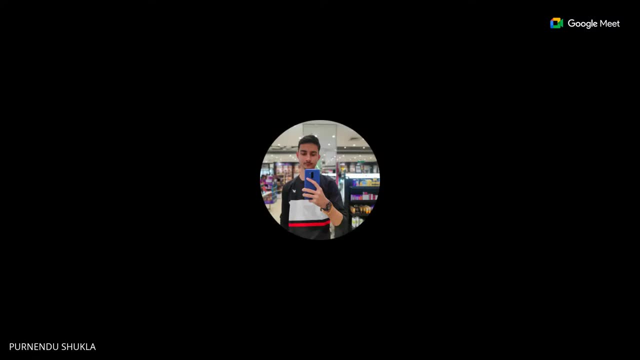 So actually I haven't completed my week eleven also. Okay, You guys, uh, carry on with the week eleven now, And I also need your some, some suggestions regarding, like I am right now in recap. I have just completed recap today, Okay, So means, 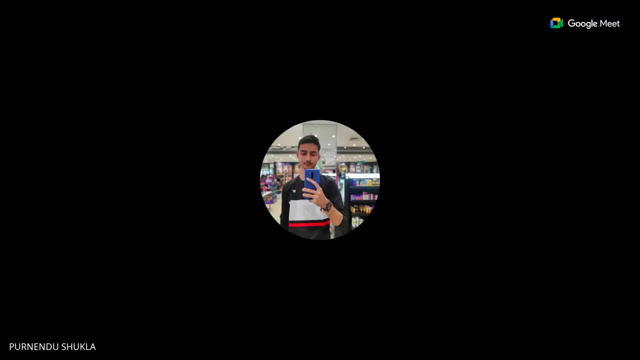 and we only left fourteen days to say So how should I prepare? Because I can't cover everything. like KKT is like uh means I'm not understanding anything from that KKT, uh, okay, what I can, what I can do is maybe next, next session, right. 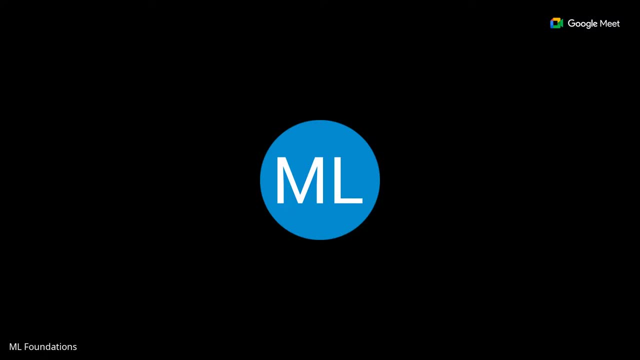 Uh, because week twelve is basically on parameter estimation. What we can do is maybe I'll go through the KKT question first, Maybe one hour I'll spend on KKT. Okay, It's not that difficult, I'll say, Because the the way we have the 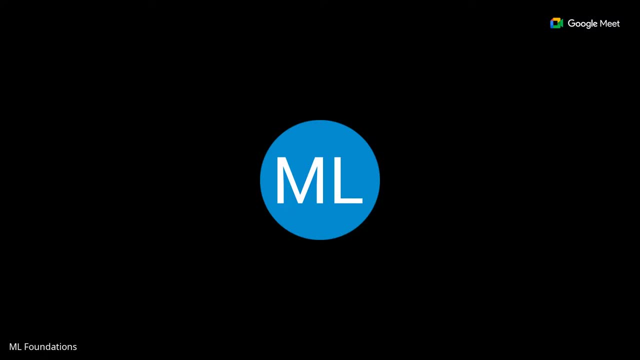 questions there. right, I'll try to take one question and I'll solve that question itself in front of you. KKT, you, you do not to go through the derivation. I have seen question where we can directly check by substituting the values in the answer: Yes, 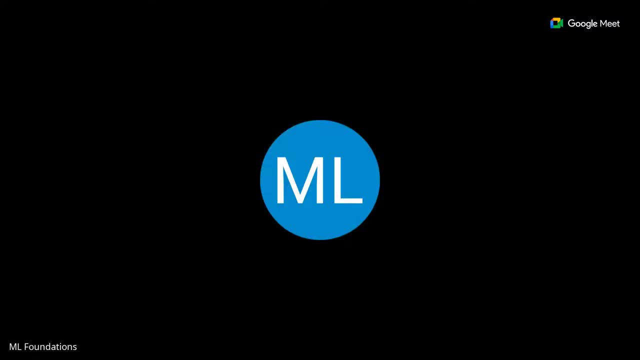 And yes, Solving based on the constraint. So if that is satisfies, we can directly do that. So if type of question comes, I am comfortable, No, no, but that it will not come that simple right. So okay, I'll, I'll just show you that KKT. 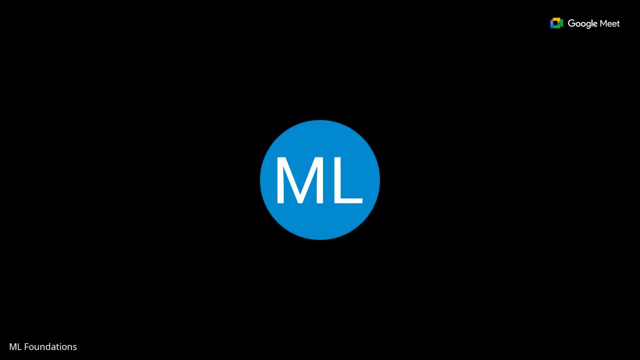 condition, Uh huh. So basically, I'll try to tell you that important topics are this: the transformation of random variables- Uh huh. So you have to go through and to understand the transformation of random variables, you have to understand the joint density and everything: Joint density. 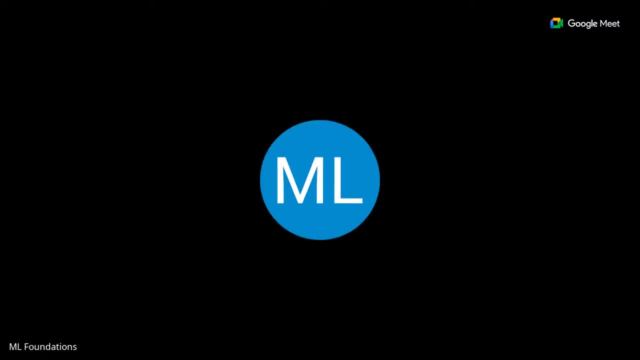 marginal and conditional, And then you should get it like: Then it is easy. for What about? what about expectation variance, Covariance, correlation, Covariance and correlation? Don't worry about it currently, but you should know. variance and expectation, Okay. Expectation variance, those topics you should be, and not for only single variation. 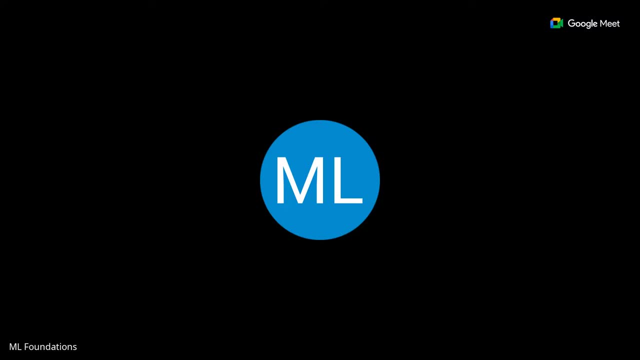 variable, multiple random variables, which is basically two random variables for three random variables. Same method we follow, like we follow today for joint: Yes, same thing. Then I have to check, because I scored like C in the stats too, So then you have to like work on that. 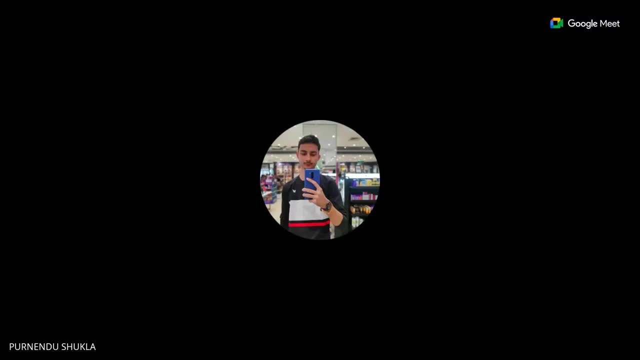 Basically the problem is those inequality questions were there so they took like around my 12 to 15 marks. OK, So it is sufficient to, if I am, go through stat 2 and not listening to 11.. So, 11-week transformation of random variable. 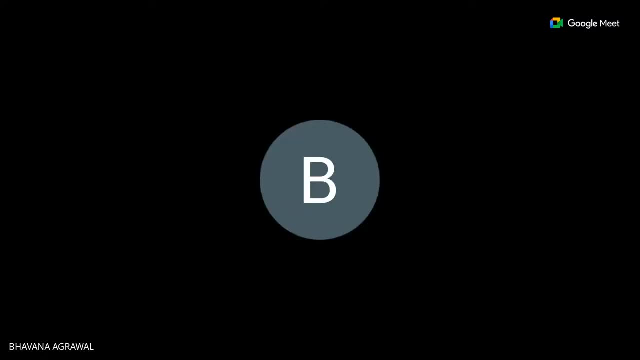 it's not covered in stats 2.. But this part is taken only Yes, Yeah, OK, Yeah, Fine, We will just. maybe what we can do is next week, right one of the session, I'll make KKT conditions. 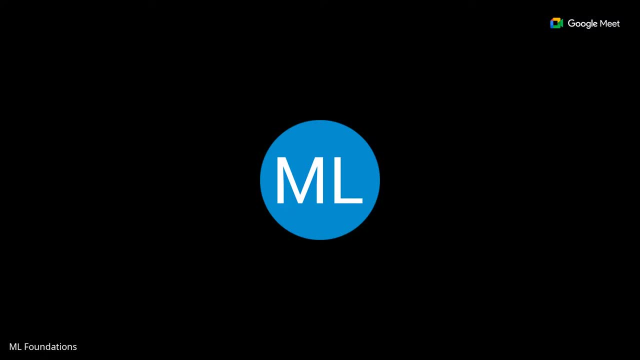 I'll talk about KKT conditions and parameter estimation more, And because there is one more topic in actually week 12, which is important- is Gaussian mixture models, But because that will also take one hour or something, So we'll see what we can do. 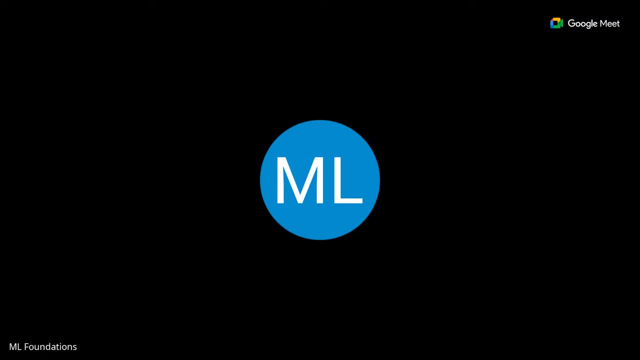 Maybe I'll make up into the next week. Maybe we'll have, Instead of solving some questions in mock, we'll just try to understand. Or maybe we'll try to understand When will release Mock next week We can. So today's are you uploaded on the? 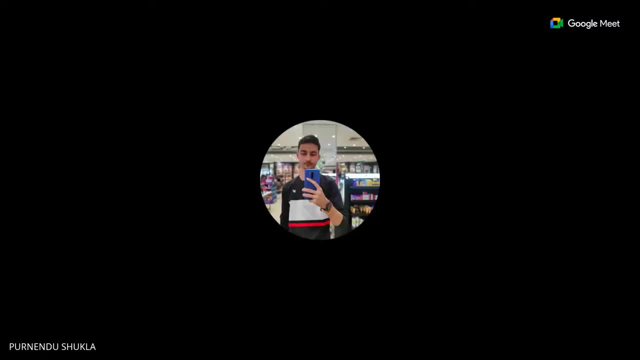 Yes, No, no, I'll upload. I'll ask them to upload. OK, Both the 11th week only. So see, basically I have completed 11th week today, So I don't think I have left any. 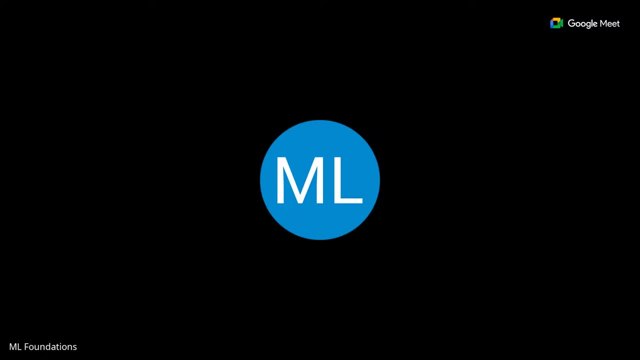 OK, And transformation also. is there Uniform exponential normal? I didn't cover because most of you know the basic things. we know. Yeah, So week 12, I'll just. And what about distributions for week 11.. In the recap there are distributions also. 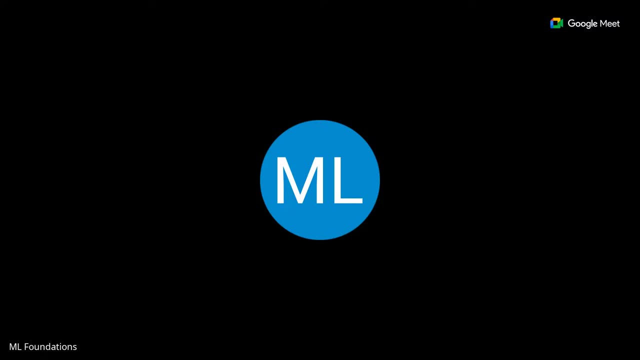 You have to understand, You have to know that. So there's basically three and three are there, I guess? Three from discrete, three from continuous. So week 12, right do is, instead of going through, solve with us week 12, uh, what we can do is i'll go through the.